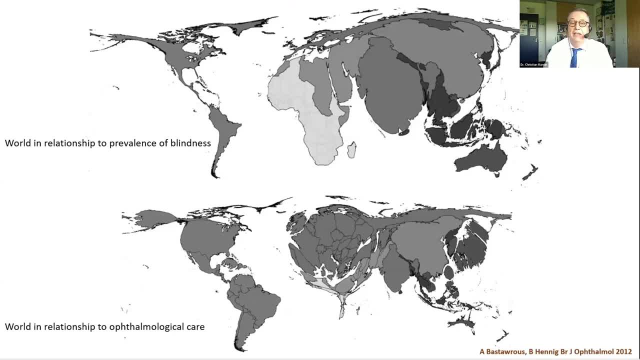 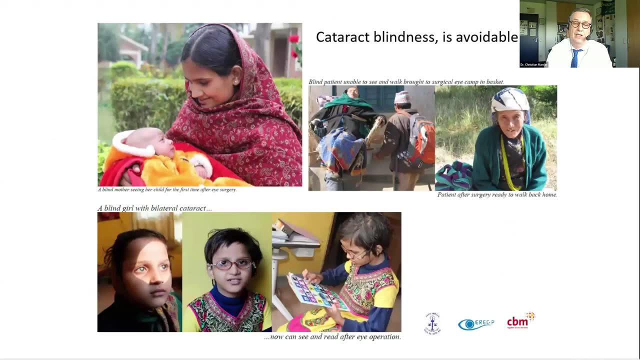 care most often lacks in the areas where blindness is most prominent And the main cause, as I mentioned, is, of course, still cataract. Cataract is a topic and a problem of excess of patients to healthcare most often And I had to experience in Nepal, in Lahan, in Behatnagar, in a CBM project. 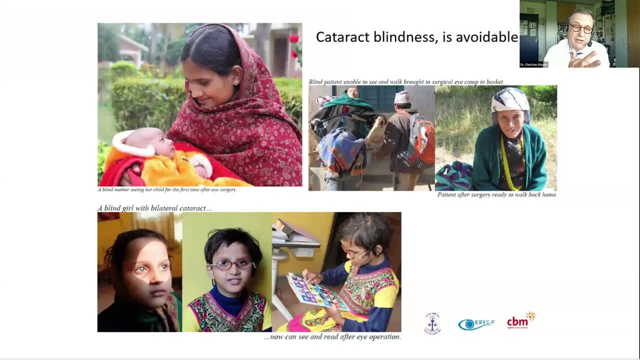 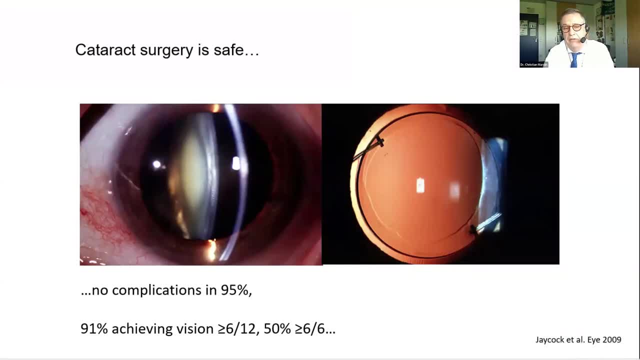 And the main cause, as I mentioned, is the cataract. The cataract has performed nowadays and in all parts of the world. FACU has become the standard is a safe surgery. It has no complications in 95%. 91% of the patients achieve a vision more than 612. And 50% even more than 100%. 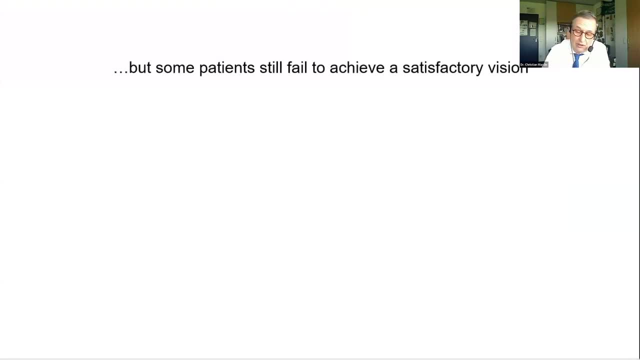 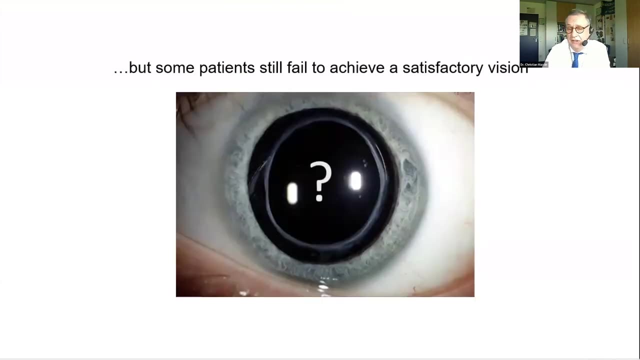 But some patients, as we have experienced all in our everyday practice, fail a satisfactory vision, And most often it is the question why this happens, And sometimes even ophthalmoscopy doesn't give us the explanation. So we talked today about using the optical coherence tomography, or OCT, to anticipate possible reasons for an unfavorable 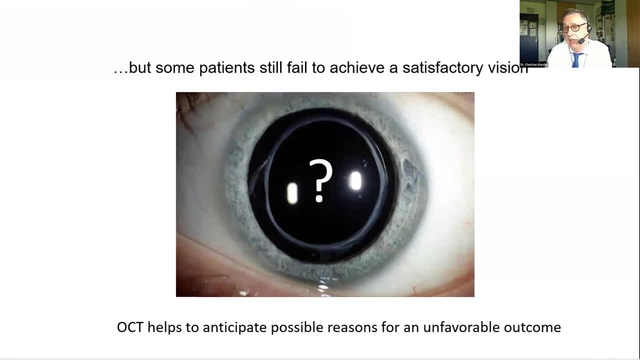 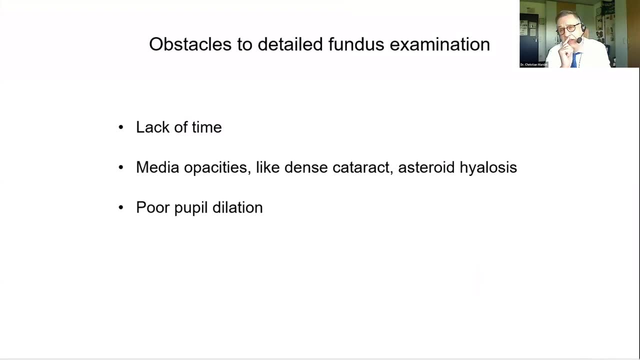 outcome or to explain an unfavorable outcome after cataract surgery. if this happens, The main obstacles to a detailed fundus examination- and the fundus is most often the key for an unhappy outcome, either retina or optic nerve- is most often the lack of time For our 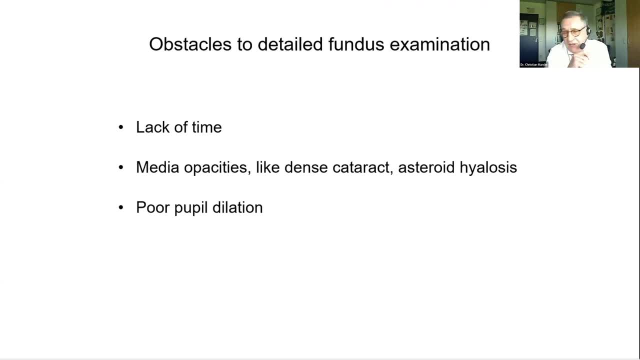 patients. we are all very busy. Medial opacities like dense cataract, the disease we want to treat, asterothiolosis, vitreous hemorrhages and pure pupil dilation, as we happen to see it in pseudo-exfoliation. 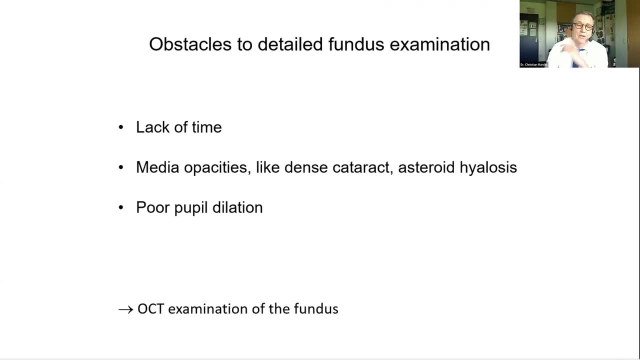 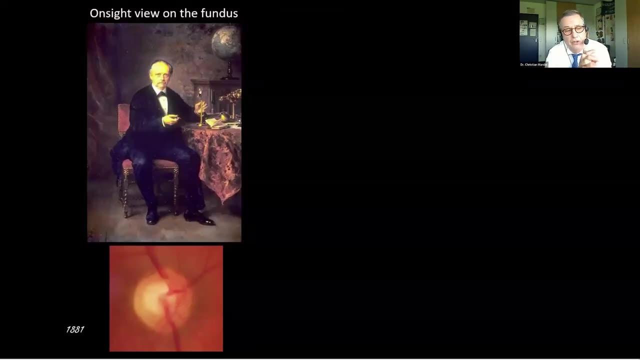 So here OCT examination can help a lot if we become able to examine the fundus more in detail. Hermann von Helmholtz in 1881 gave us the ophthalmoscope and the ability to have the onsite of the human fundus, But with optical coherence tomography. and you know all these. 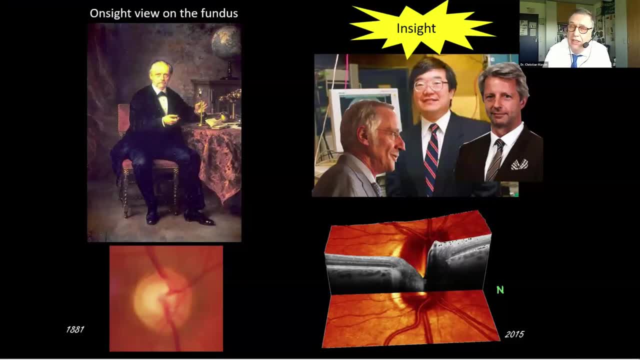 three people, it is very difficult to determine if the fundus is real or not. He also helped develop this technique a lot, which gives us an insight into the tissue of retina and optic nerve head to understand in vivo better subtle changes most often invisible to us. 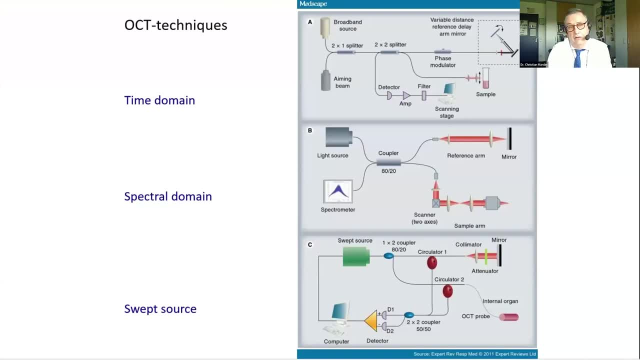 during ophthalmoscopy. Roughly the OCT techniques have developed a lot in the past 20 years. We all remember the time domain status OCT from Saez, which was a pioneer for everyday use of OCT over spectral domain technique. Now SWAP source technique is available and roughly 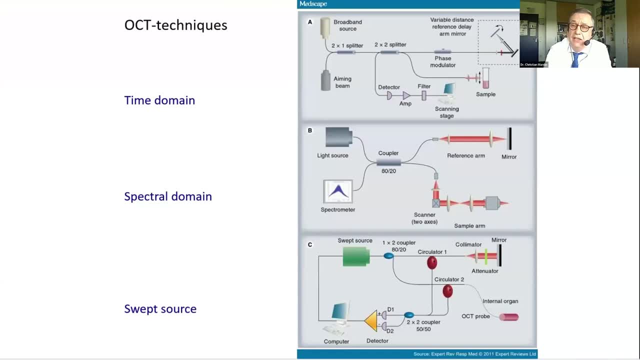 laser light, like in echography, is sent onto the tissue of the eye and is slowed down by the tissue And the slow down or laser light change in the spectrum, as we do with the spectral domain, OCT is then computed And, like in echography, the two differences in the laser light 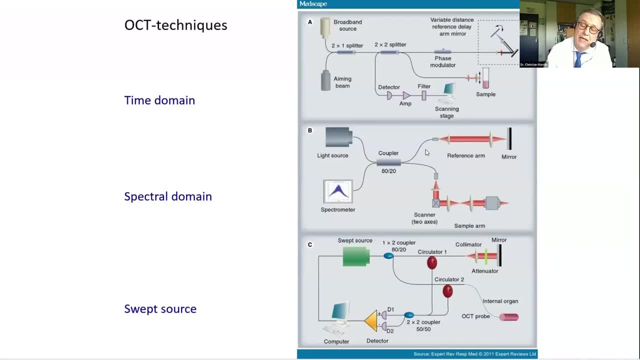 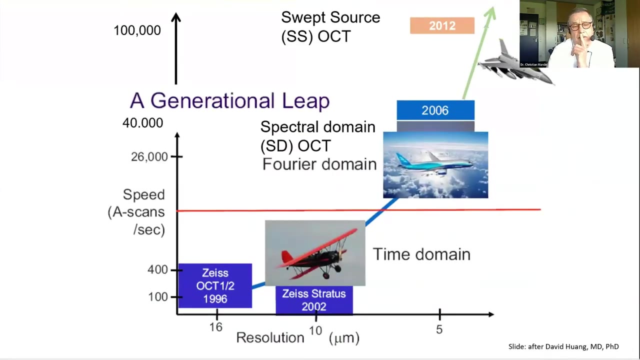 going into the eye and coming out of the eye is compared by the computer and then translated into a picture which reminds us of the histology of the eye. with high resolution Spectral domain, OCT, has not improved a lot in axial resolution up to five to three microns, but also has become a very 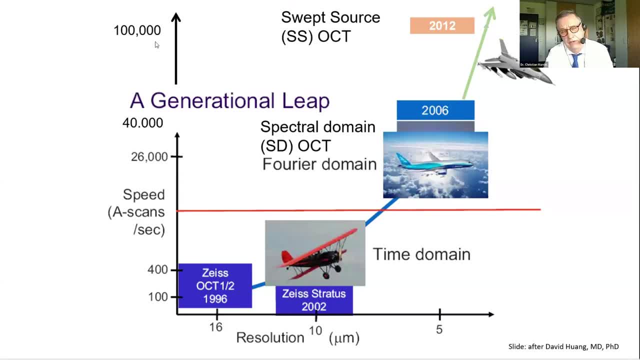 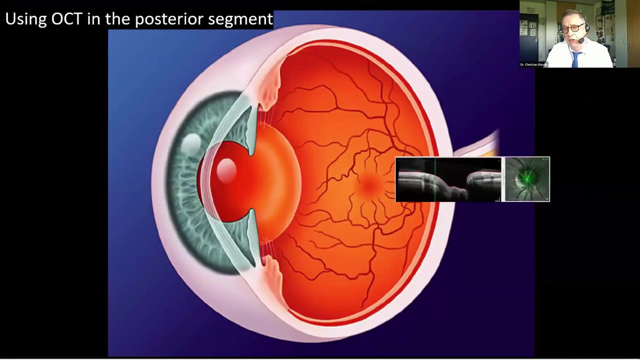 fast technique with more than 100,000 eye scans a second. So we are available to examine our patient, even if patients are difficult in cooperation, in a very short time And it's a non-invasive examination. So when we do that, on the posterior pole we are able to visualize the optic nerve head. 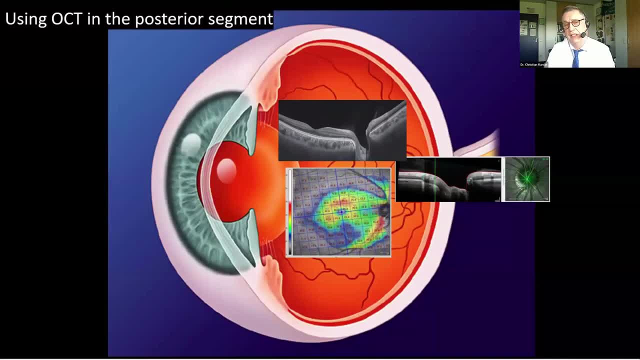 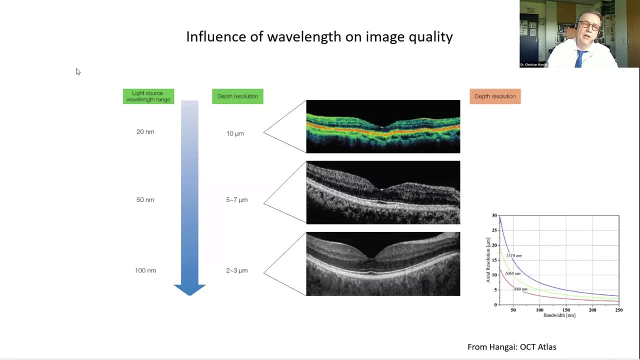 the retina. We are able, with fast OCTs, to create volumes of the retina and measure different tissues important to us in everyday use. One achievement is the development of broader wavelengths for the laser source. Broader wavelengths have been very expensive in the past, but now it's commercially available. 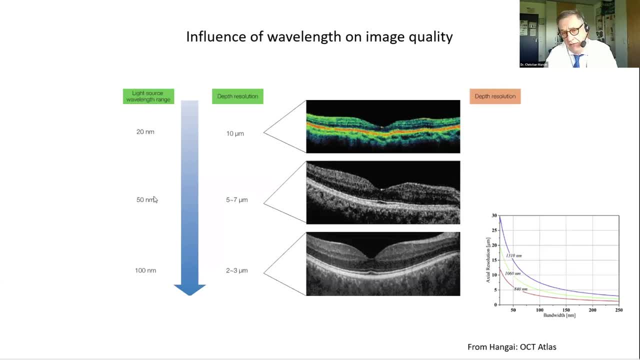 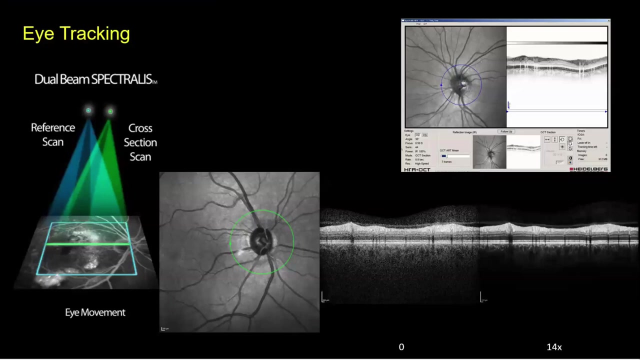 in all the devices, And the broader laser wavelength helps us to improve the axial resolution on the fundus and gives us a better and more detailed image Thanks to the modern techniques of laser light. Another very important achievement is a kind of eye tracking. 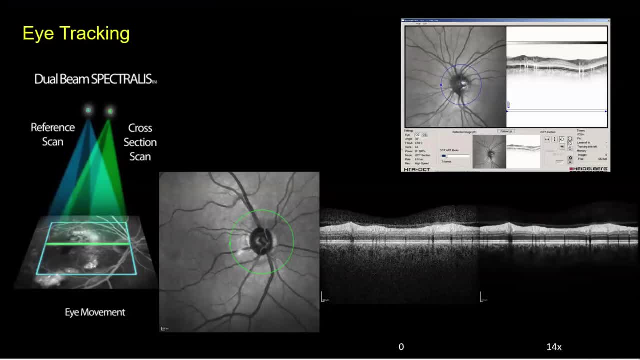 And I will show you in the following most often examples from the Spectralis OCT on the fundus, because we use it in everyday work. And the Spectralis has a special feature: It has two lenses: One is laser beams scanning the fundus and one serves as a reference scan. 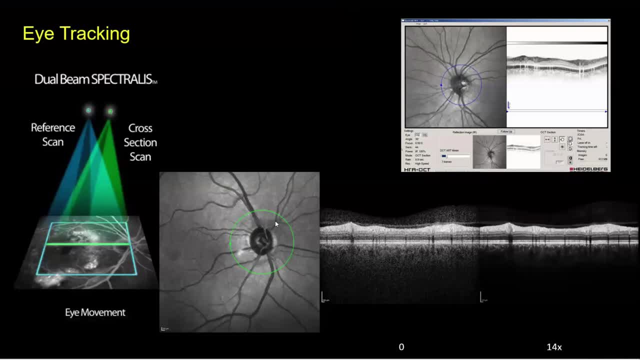 The other is the examining scan. So you are averaging on a single safe spot. And by averaging the scans on the spot you increase the resolution of your B-scan image. On the upper right-hand corner you see the example. The patient moves his eyes but the picture doesn't move and is averaged. 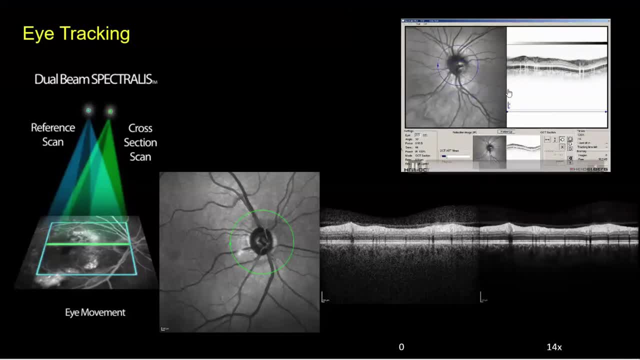 And it becomes sharper and sharper by averaging. And this is not only easy for patients who can't cooperate easily, like children, elderly or mentally disabled patients, but it helps also to find the same spot in the following follow-up examination and then to compare two time points. 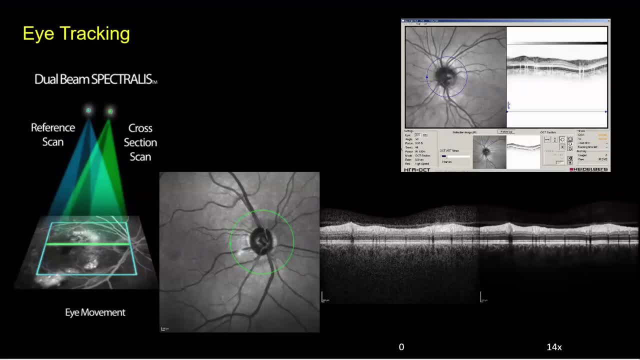 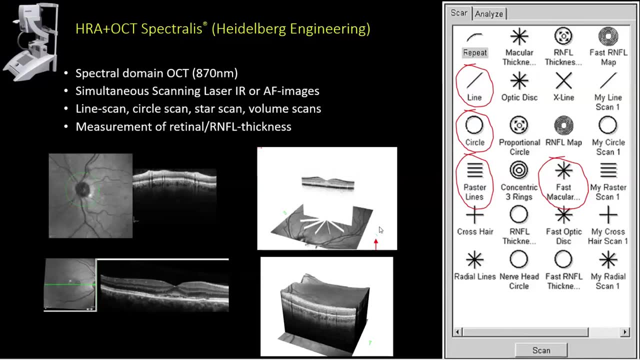 And this helps a lot. Thank you, Thank you, Thank you. Awesome, Thank you. It was very helpful. It's very important to even find very subtle changes of the retina and optic nerve head. Beautiful Different scan patterns, line scans and volume scans are offered by this very fast. 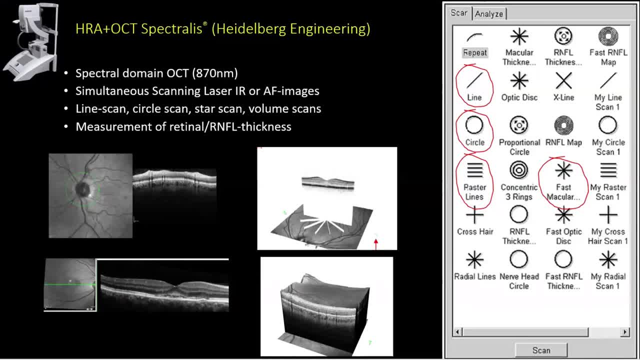 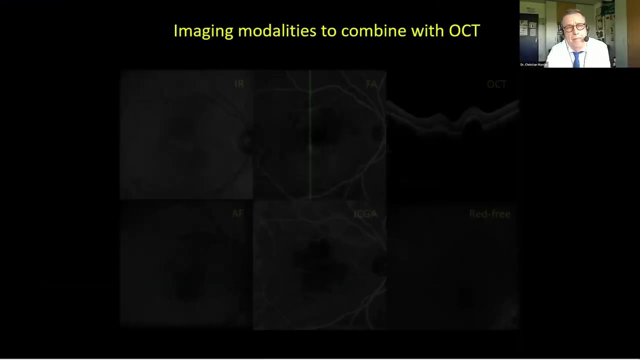 technique and very high resolution technique And in the setting of cataract surgery, most often line scans, circle scans, fast star scans or volume scans are used in order to detect any damage to the patient's eye, detect pathology of the fundus of the retina and the optic nerve head. 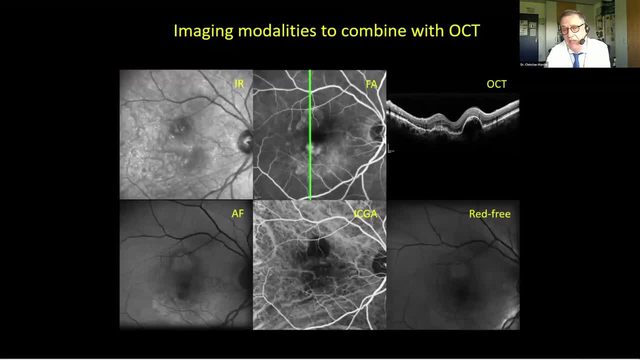 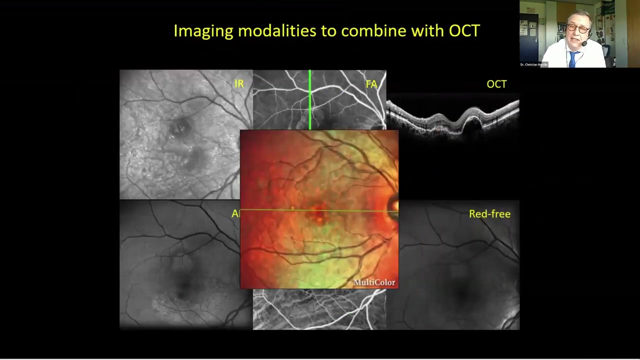 The nice thing that in most available OCT devices you don't only have an OCT scan but you can combine the OCT modality with infrared pictures, the fluorescein angiography, with ICG, autofluorescence, red-free pictures or even multicolor images and get a very 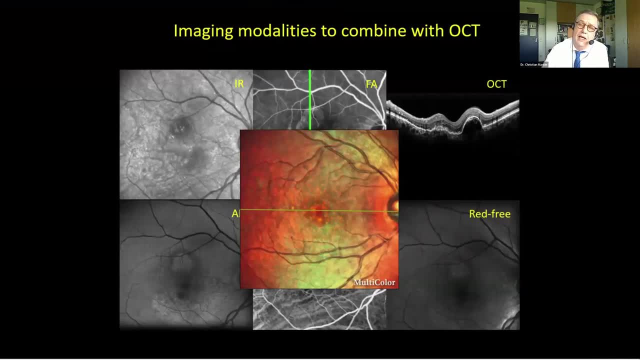 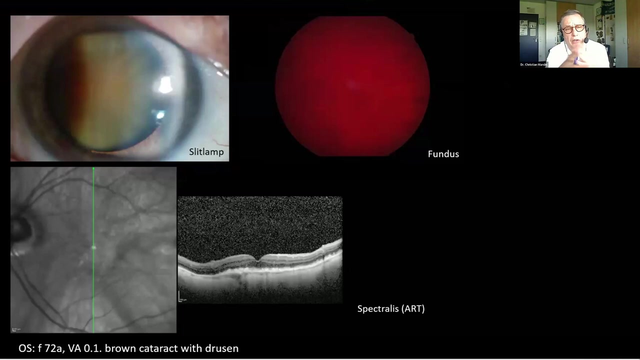 good idea of the fundus, not only by scanning a certain area, but getting an on-view on the fundus with false colors, which helps a lot to detect pathologies sometimes hidden from our eyes doing ophthalmoscopy. This is an example of a 72-year-old lady. 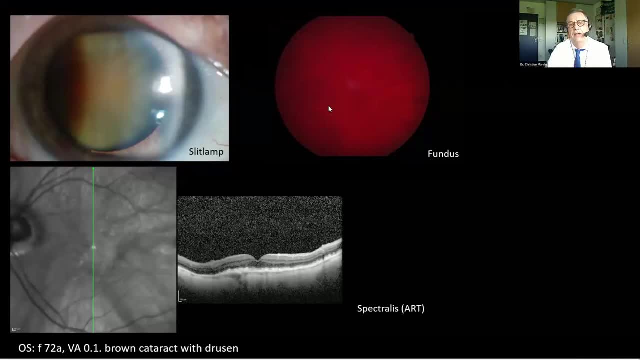 You see the brunessent cataract at the slit lamp and the fundus image just gives you an idea that the optic nerve head could be situated here. the retinal vessels, this could be the macula, but you don't see any details. 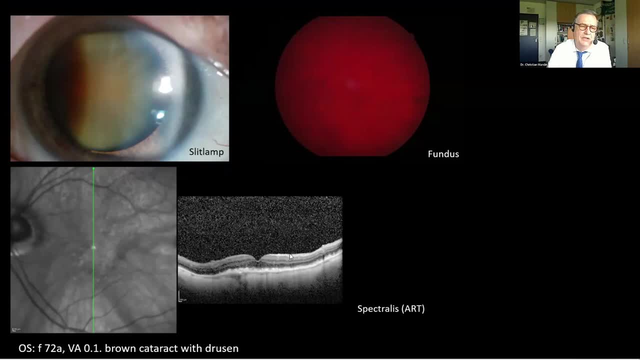 By doing OCT with the spectralis, you are able to see that the patient has chosen changes of the OCT. Okay, So you can see that the OCT image is not visible. You can see the photoreceptors perhaps not permitting full vision after cataract surgery. 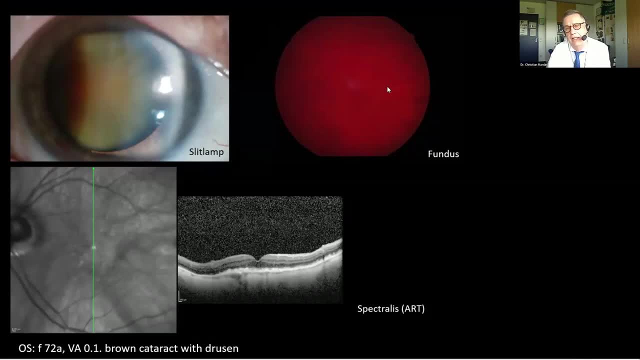 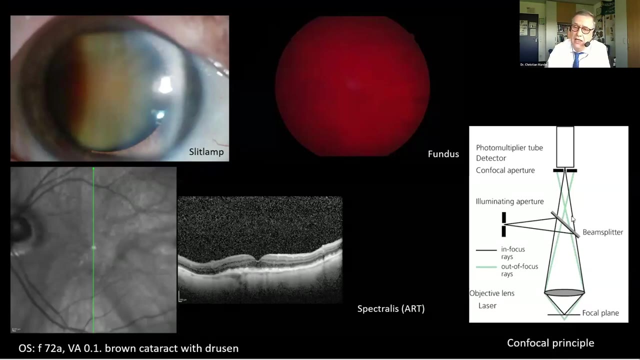 Also, you get an infrared image, laser scanning image of the fundus which is more detailed when our white light fundus image due to inward and backward scatter of the light due to the opaque lens. One technique helping us in the OCT device is the confocal principle, improving the sharpness. 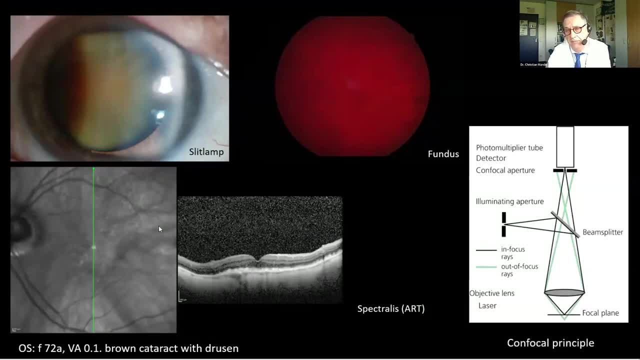 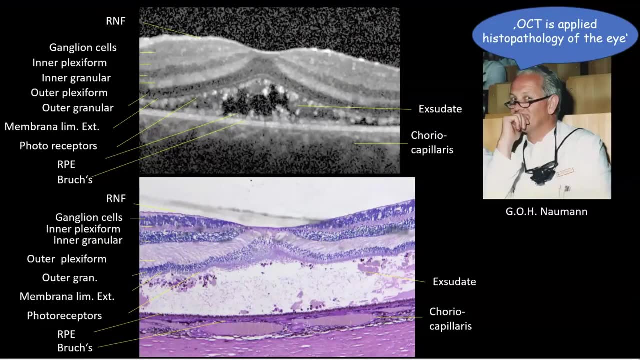 of the OCT images. even in the SLO scan a lot With the high resolution up to three microns we get an image very much similar to histology. we all know from our medical school And here's an example of a patient where the eye had to be inoculated due to a choroidal 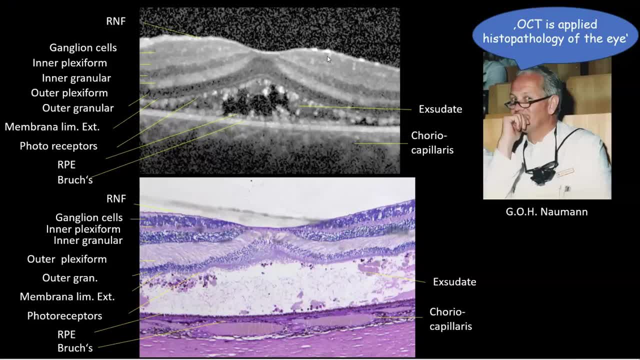 melanoma And we tried to, Okay, We tried to compare the OCT scan before operation with the histology after removal of the eye And you see that the layering of the retina is very similar to histology. Of course we had the artifacts by the histological preparation, but the exudates and the cells 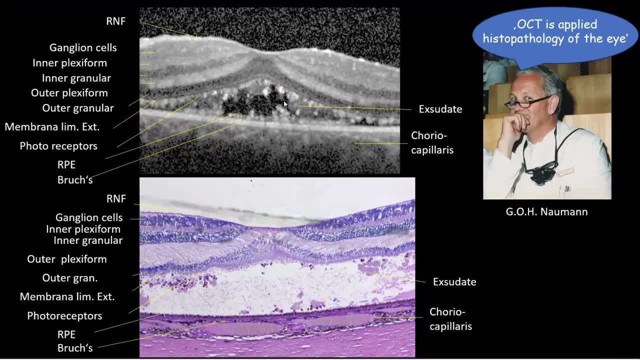 under the retina are nicely depicted in the in vivo picture prior to surgery. So OCT gives us, with the structure OCT, a very good, Very good image and very comparable to histology. Even the slight epidermal membrane you depict here in histology is found also in the in. 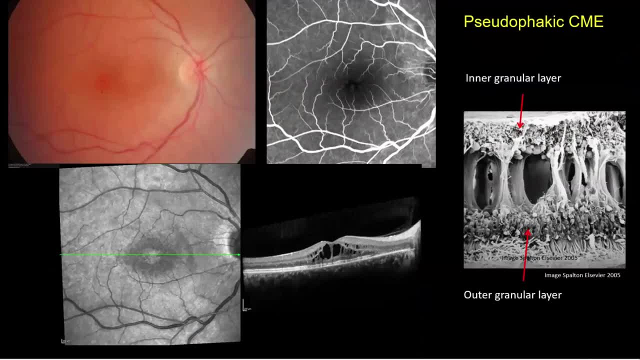 vivo picture. Main problem after cataract surgery- and this happens in about 2% of our patients, even if the cataract surgery was uncomplicated and it will resolve in 90% after one year- is cystoid macular degeneration. 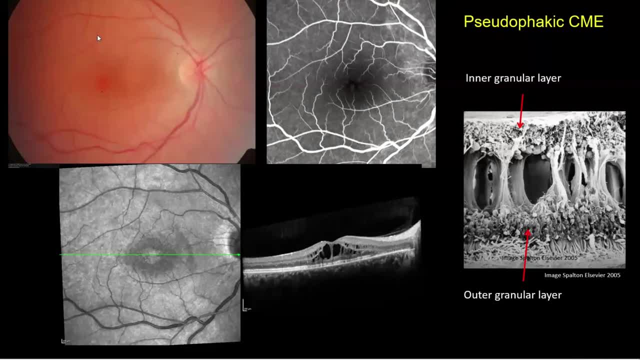 The whole thing is very similar to the cystoid macular edema, or CME. When you do ophthalmoscopy, even with dilated pupils, it's sometimes very subtle and can't be appreciated. But when you do OCT scan you immediately see the cystoid spaces in the inner nuclear. 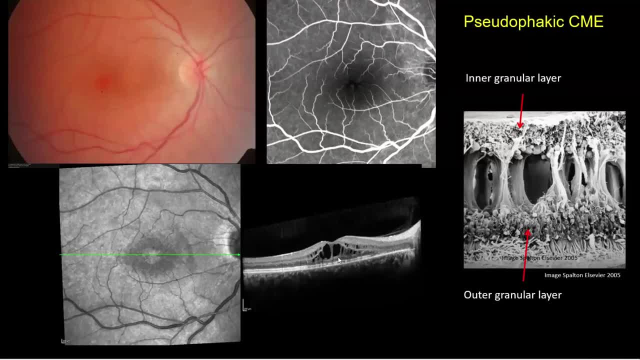 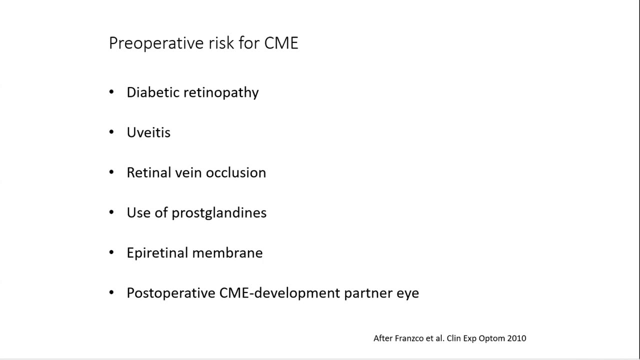 and the outer plexiform layer and very much resembling the nice electron microscopy images from the atlas of Spalton. Okay, So what is the preoperative risk for cystoid macular edema? It's most often diabetic retinopathy. 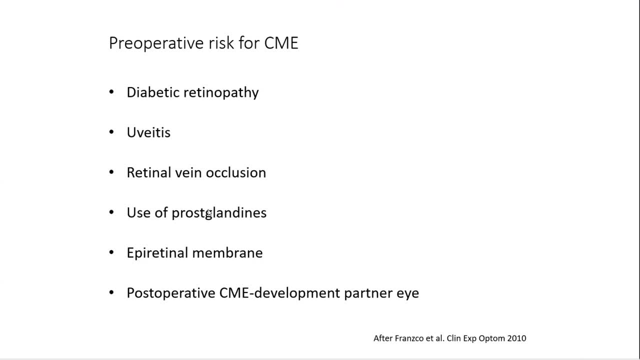 It's uveitis, It's a lateral vein occlusion use of proxaglandins in glaucoma patients, epiretinal membranes and the history of the partner eye. If the partner eye also developed CME, then the eye- the second eye- we will do surgery. 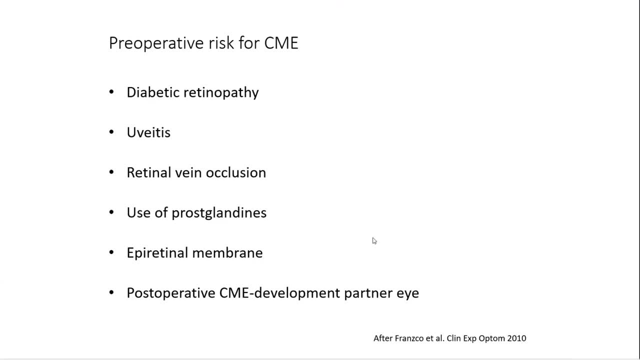 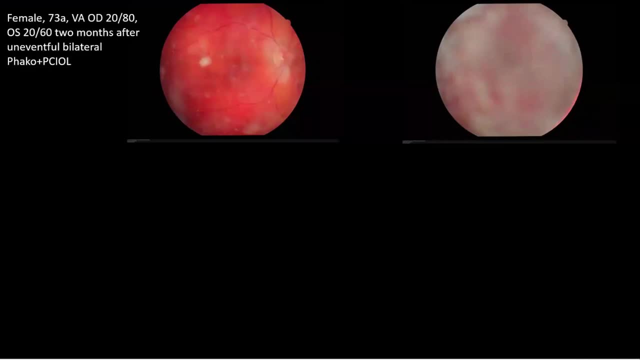 on is liable to get OCT. Okay, So here's an example of a female who, two months after uneventful bilateral FACO with PCIOL, still did not gain full vision. back On the fundus picture we see that on the left hand more than the right hand side. 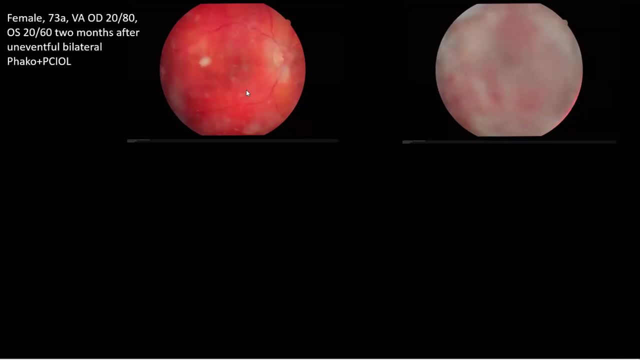 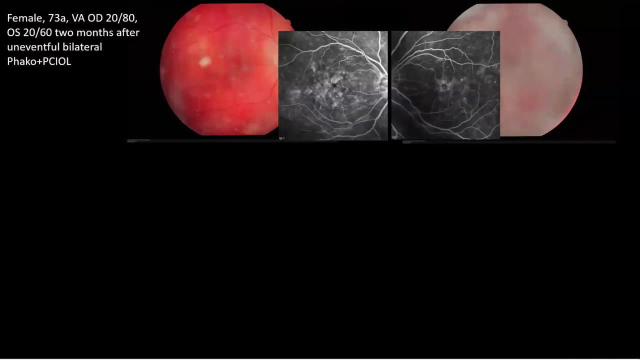 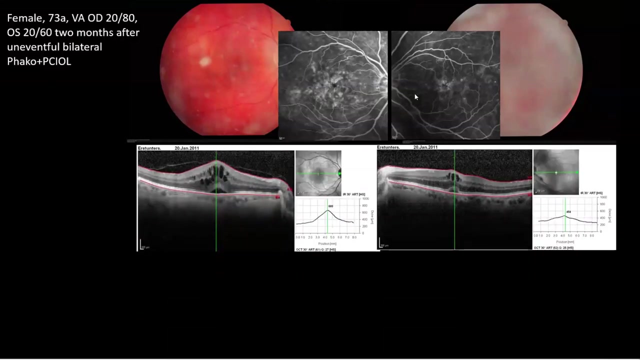 the patient has an asterisk hyalosis blocking a nice and sharp fundus image and blocking our eyes from reality. When we look with the SLO picture in the infrared spectrum of our OCT and then afterwards using in the FLA with fluorescein angiograph, we nicely depict the cystoid macular edema. 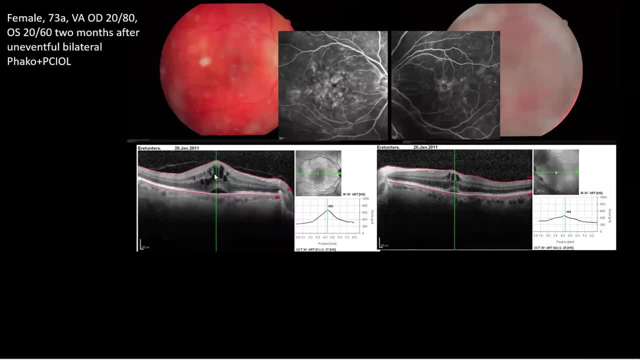 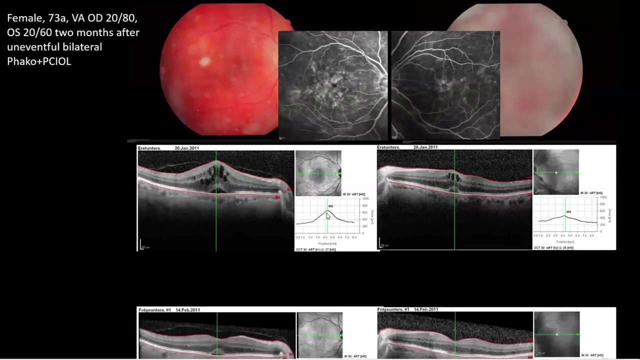 And with the OCT we can measure even the central vaginal thickness and appreciate the cystoid macular edema. So in the time of OCT we can stop doing the fluorescein angiography to find out the cystoid macular edema, because I have the OCT. 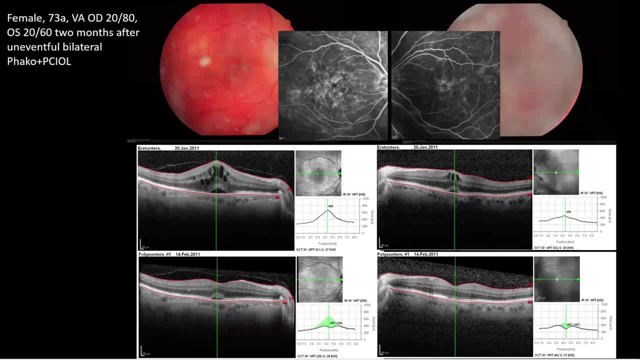 So after the treatment with anti-inflammatory eye drops and carboanhydrase inhibitors, the cystoid macular edema resolved in this patient and visual acuity increased again And again. you see the beauty of scanning the same spot as in the first picture. 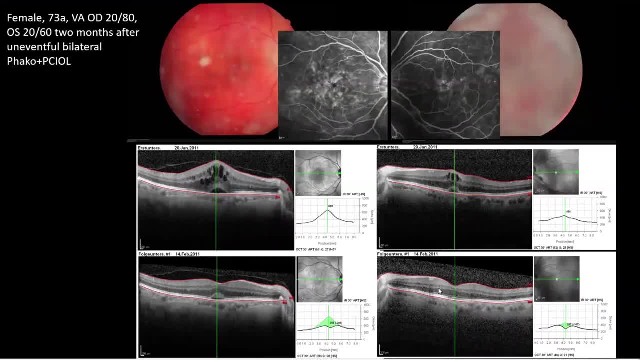 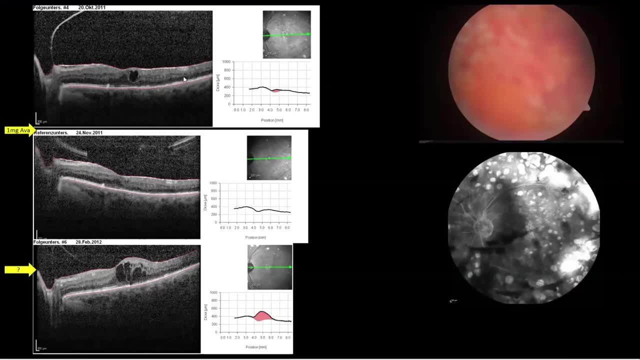 You can directly say what has changed or what has not. Okay, So what has not changed if you are not successful? This is a patient with diabetes. After cataract surgery developed the cystoid macular edema. anti-VEGF therapy was done. 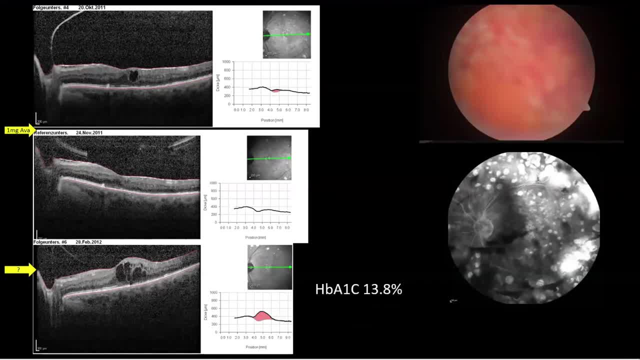 but was not successful. And the main reason in this patient was an uncontrolled blood sugar. And the second thing is that the patient not only has diabetic retinopathy Nicely visible in the infrared picture, much better than an ophthalmoscopy. 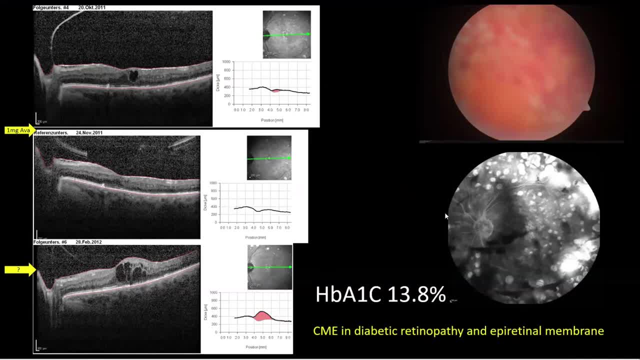 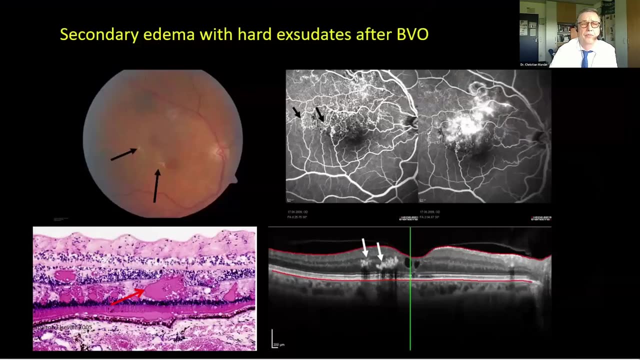 But also has an epiretinal membrane, And this example gives us one reason why cystoid macular edema may develop after cataract surgery is an uncontrolled blood sugar, And patients should be advised to improve the situation prior to cataract surgery. 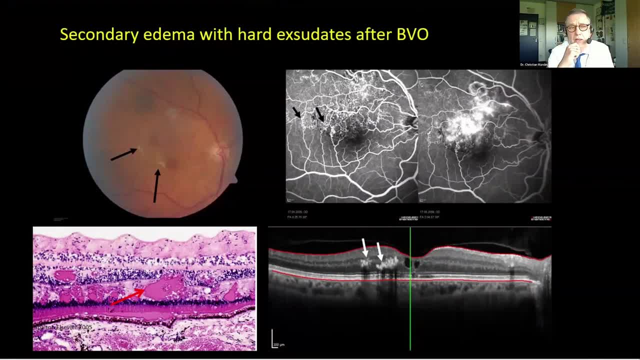 Also secondary edema after branch vein occlusion. When the hemorrhage has disappeared then you have to do a very detailed ophthalmoscopy to find this hard subtle exudates. The hemorrhages have dissolved And in the fluorescein angiography you see the collateral vessels between the perfused. 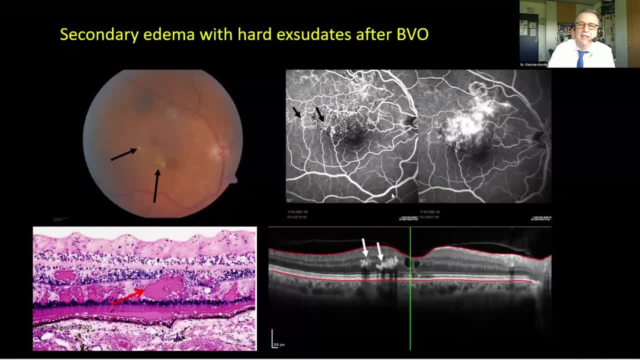 and non-perfused area causing exudates and cystoid edema Nicely depicted here in the OCT scan, And this problem should be addressed Prior to cataract surgery, Because after cataract surgery this exudates and especially cystoid macular edema may get. 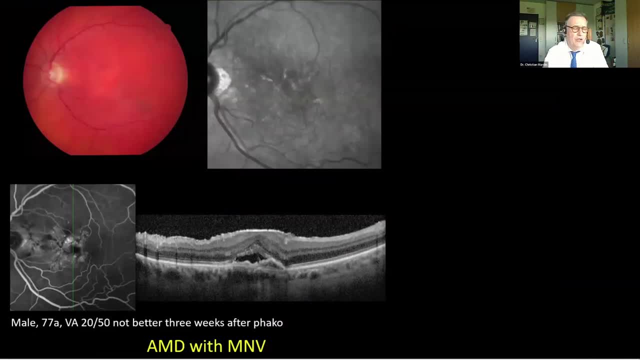 more. Here's a patient, a male patient, 77 years old. This is the fundus picture. a little bit of bruising paleness, but nothing special. Got cataract surgery and did not improve after three weeks after FACU. 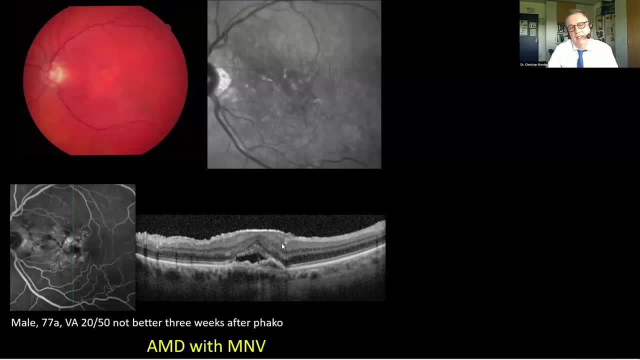 So FLA and OCT scan was done And then it becomes visible that the patient has a subretinal edema fluid under the retina and under the pigment epithelium, Very much hinting towards MND and AMD. And this patient was lucky enough not to get the hemorrhage after the cataract surgery. 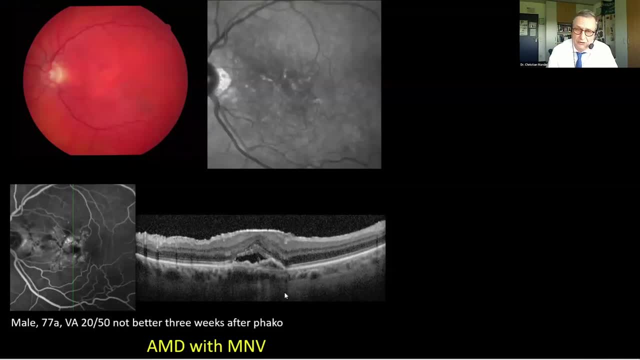 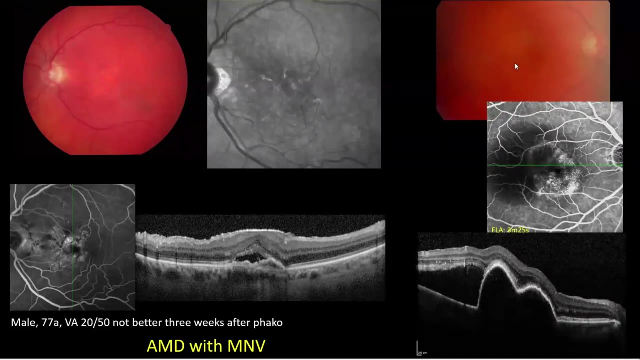 In this case, if we would have a good OCT image prior to surgery, We would have treated the MND first before doing the cataract surgery, or then doing a combination of both. The same is true for this patient. The fundus picture doesn't reveal any sign of MND. no hemorrhages, no exudates. 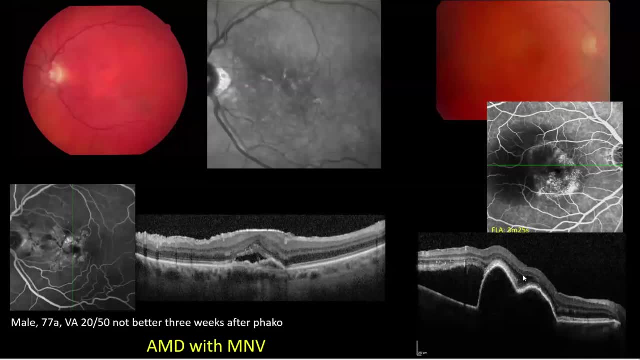 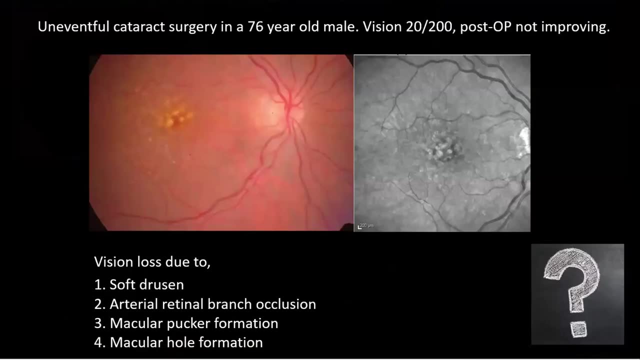 But in this OCT scan you see the giant pigment epithelium detachment and the subretinal fluid. So Okay, So this is a question to you. This is also an old male with uneventful cataract surgery, but after surgery vision was not. 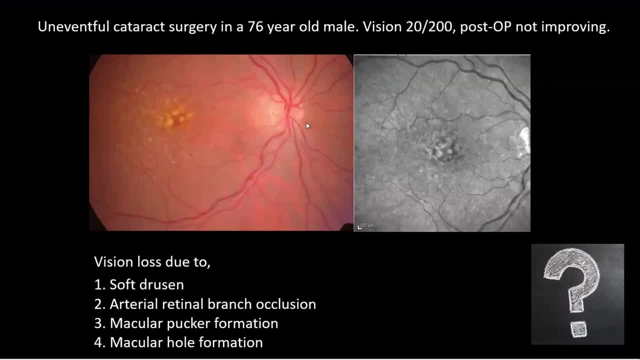 improving and the patient was very not much satisfied. So you see the fundus picture here on the left-hand side, the infrared picture on the right-hand side. And now I would ask you: what do you think? What is the reason for the vision loss? 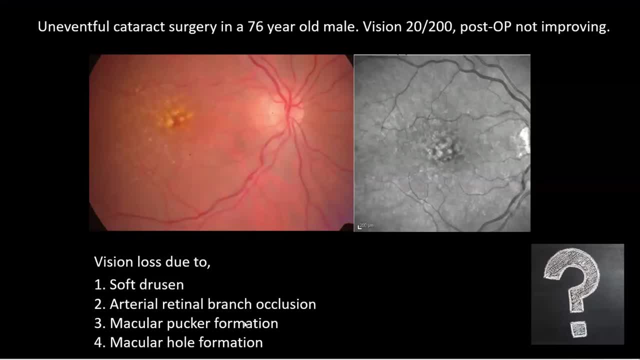 Soft drusen, Arterial branch occlusion, macular paca formation or macular hole formation. You may now vote and then we look what your opinion is. I think this makes the whole lecture a little bit more vivid. 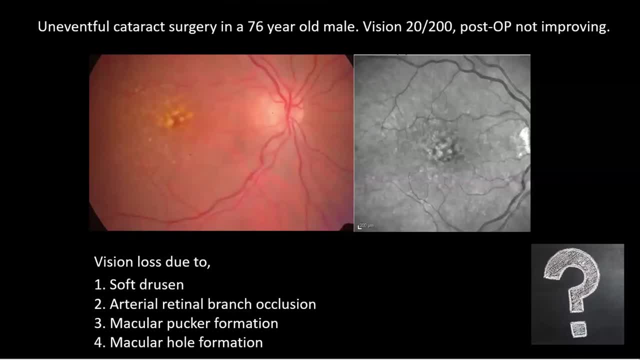 You have 30 seconds and then we will look how you decide. So the polling is in favor of soft drusen. That's the majority And thank you very much. Thank you very much for voting Now. we will have a look. 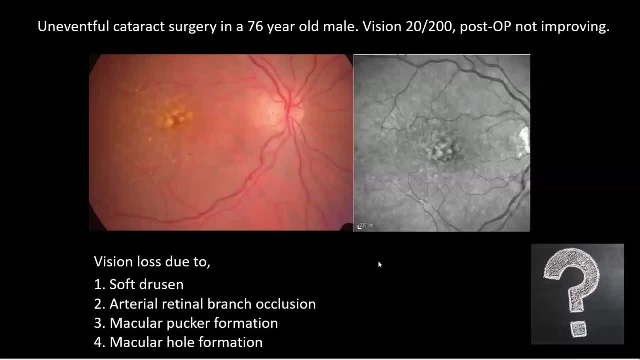 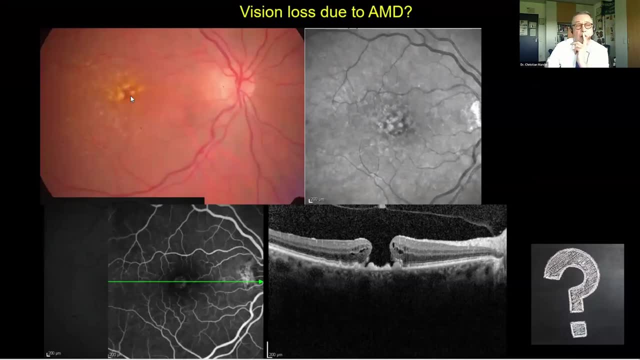 The OCT, in this case, helps us. And what do we find? It was the minority already I'm hinting towards. yes, it was a full thickness macular hole, stage four, according to guess, And when you look very closely you might see the slight ring in the center showing 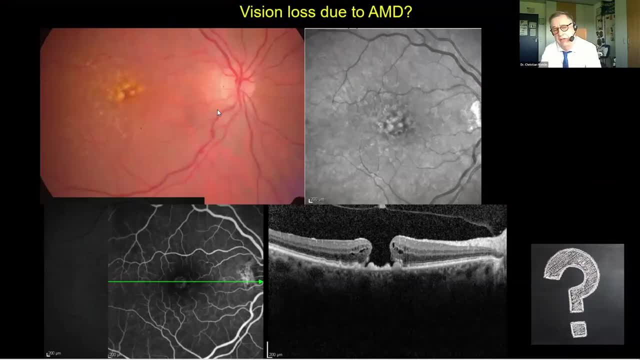 you an ophthalmoscopy? That might be an ophthalmoscope, That might be an ophthalmoscope, That might be a macular hole But very difficult to see. But it's just one click with OCT. And if this would have been appreciated prior to surgery, the whole cause of the surgery. 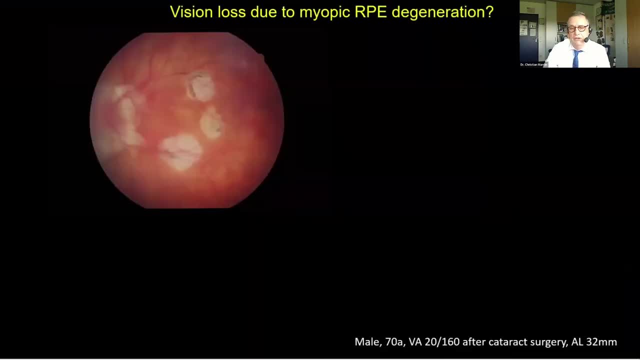 would have been different. So this is another male after cataract surgery, still not satisfied with a very long axial length of 32 millimeter. You see the posterior atrophy of the pigmentoepithelium and the choroid, The myopic disc. 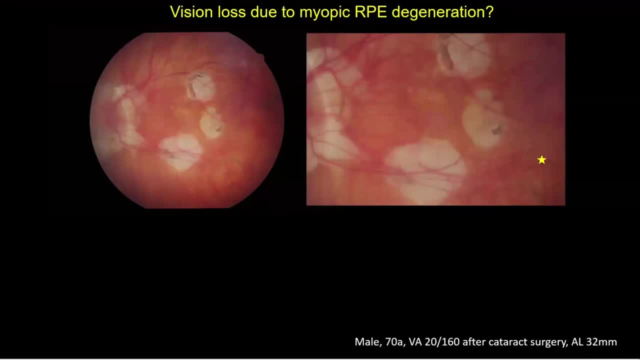 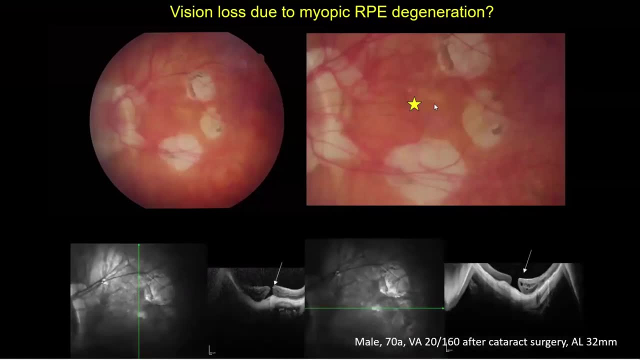 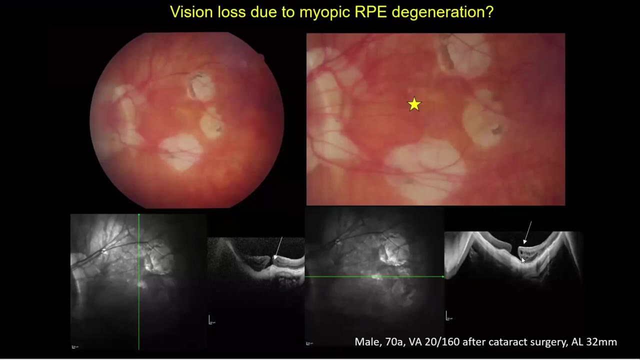 And also in this patient. when you look very closely and you test the fixation, the fixation seems to be at the place where it should be. But again, this patient had this small macular hole And this was the reason why cataract surgery didn't help him much. 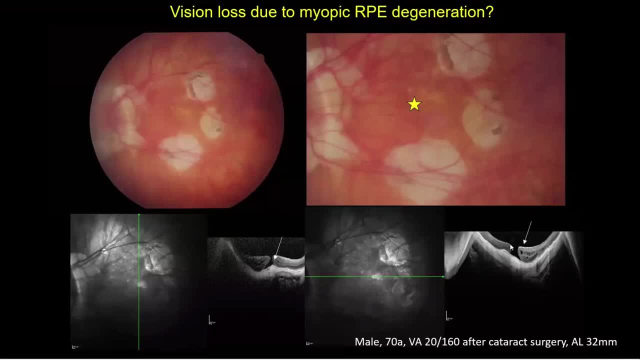 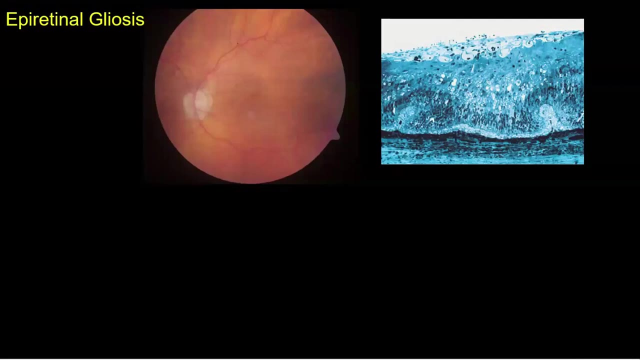 And the next question is to do retractomy and peeling on him. But this again would have been appreciated If OCT scan would have been done prior to surgery. Epiretinal gliosis is very often a reason for reduced vision after surgery and even 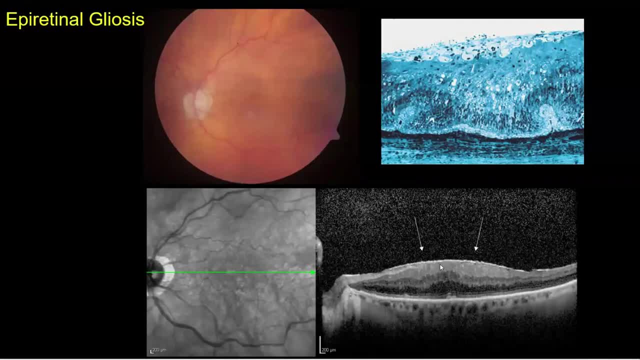 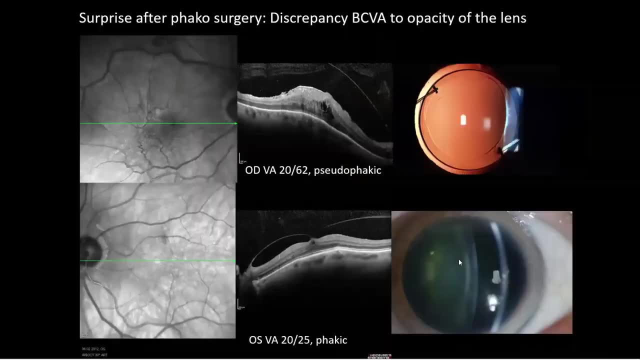 causes cystic macular edema to a higher extent after cataract surgery and should be appreciated before surgery and discussed with the patient. This is an example where in the pseudophagic eye the patient did get a little bit of a cataract. 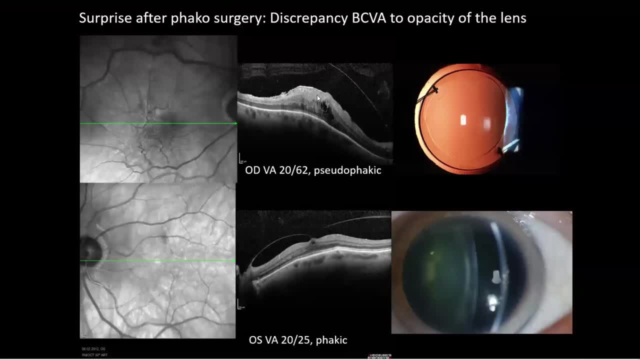 The patient did not gain much vision due to this huge epiretinal membrane and thickening of the central retinal thickness. On the other eye, with a slight cataract, vision was not too bad. He had a vitreo-macular traction and vision was much better all the same when on the 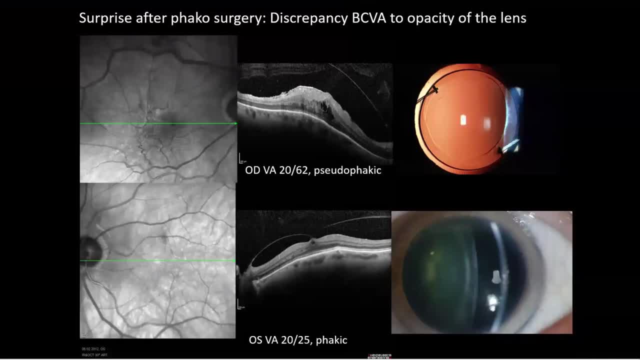 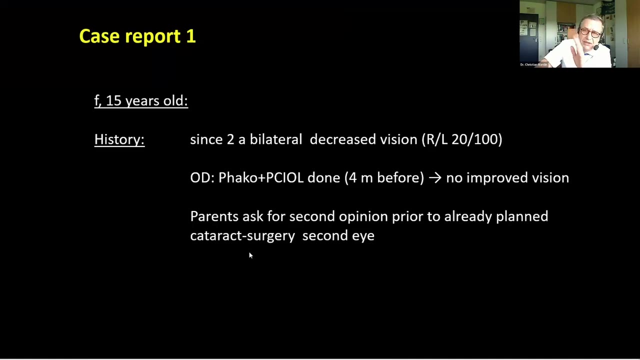 other eye. So the patient has not only cataract but a vitreo-retinal problem And in this case could have been advised differently prior to surgery. This is a very rare but a little bit sad case of a 15-year-old girl which showed to. 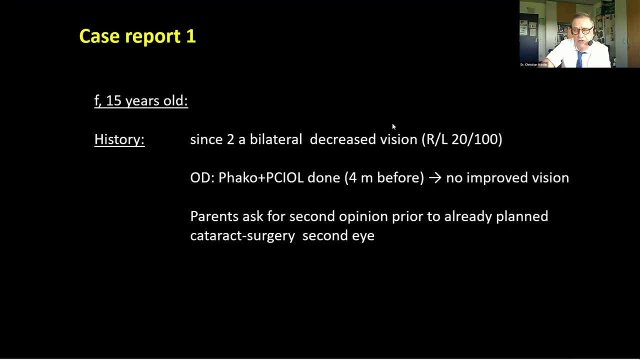 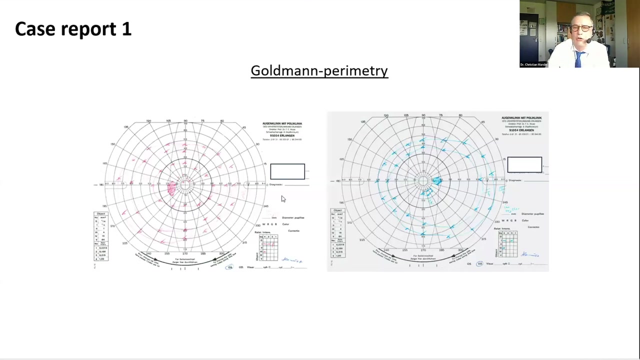 the doctor a bilateral decreased vision since two years And on the right-hand side a FACO was done with PCIOL four months before. Vision did not improve and the patient was shown to us because the parents asked for a second opinion. So of course you think of something neurologic to do a visual field. 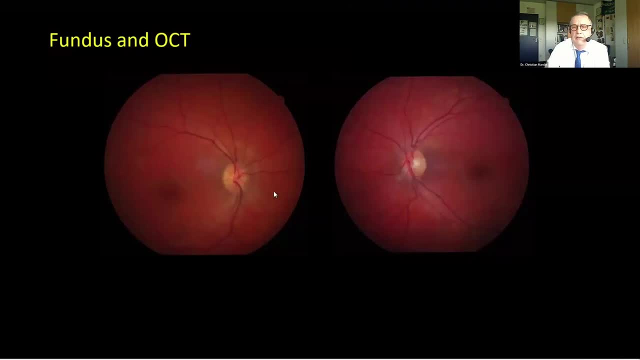 This was quite okay. You look at the fundus. These are the fundus pictures of the girl healthy optic disc. not very, not much change on the fundus, Perhaps a little bit. these light spots on the left-hand side, the right fundus looks. 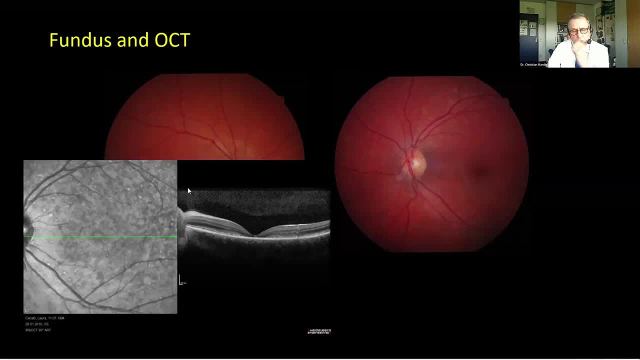 on the image, quite nice. When we do the infrared Okay Imaging or the infrared imaging, we see that the patient has the typical or atypical- in this case drusen. And when you do OCT scan, you realize that the photoreceptor outer segments are no more. 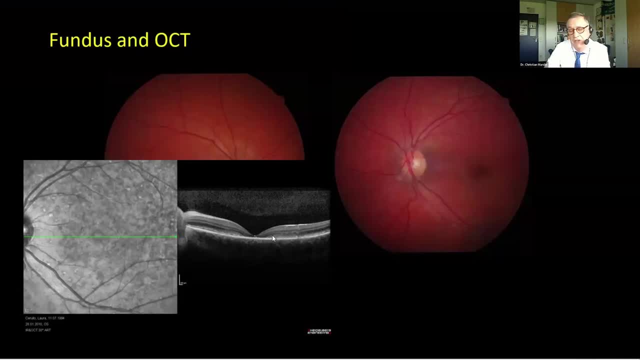 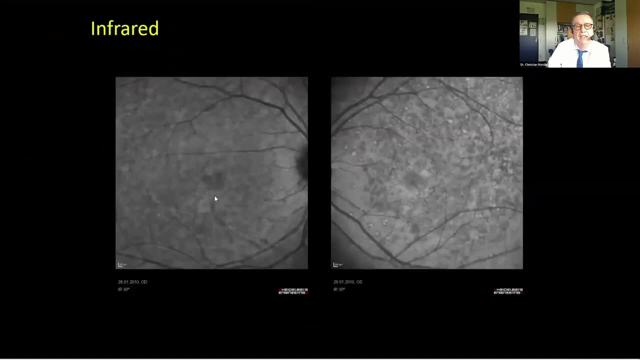 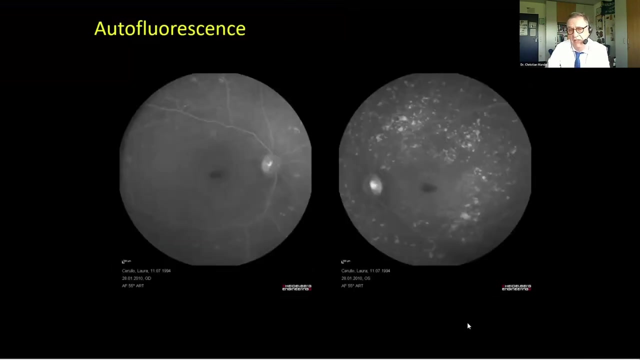 present in the center of this patient. This was the reason why visual acuity dropped down and cataract surgery did not help. The picture on the right-hand side, and on the left-hand side you see this atypical drusen, And I think everybody else of you already has an idea: autofluorescence, it's a typical. 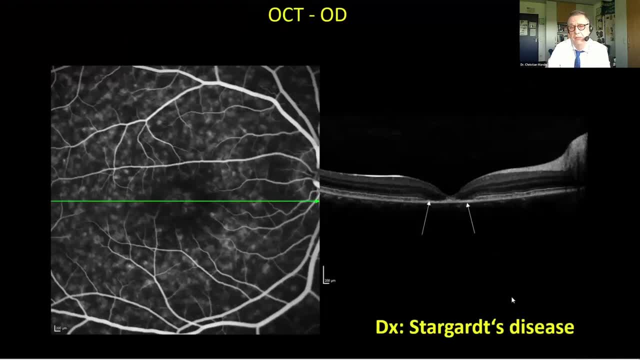 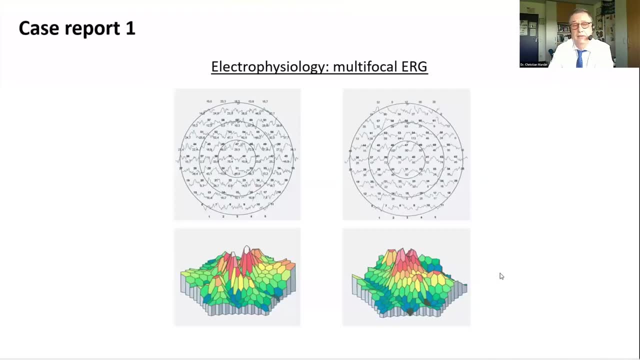 picture of a Stargardt's disease And this patient was suffering from the Stargardt's disease and therefore cataract surgery did not help a lot, but the patient lost its accommodation ability And also multifocal ERG. you'll see the changes typical for the central diminished vision. 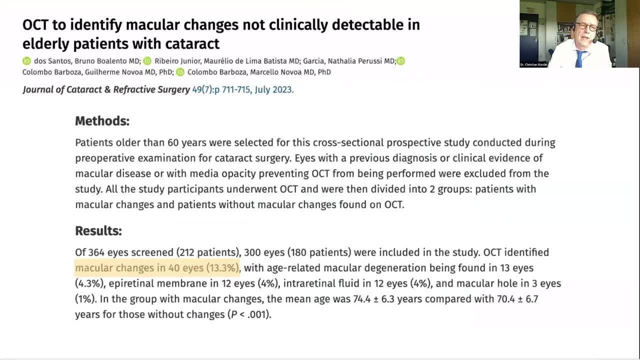 in Stargardt's disease In a nice publication from Brazil, Dos Santos, and colleagues did OCT scans prior to macular surgery and they found in eyes which clinically looked okay in 13.3% macular pathologies and changes. 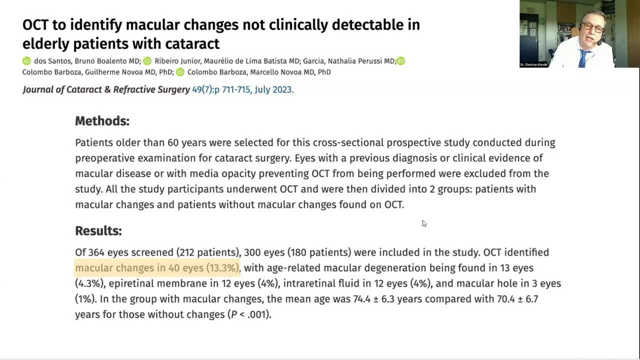 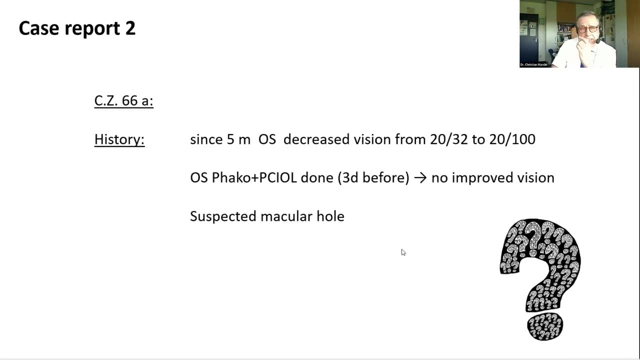 And I think that's a high percentage, which would advise to do us OCT on patients where we are not Okay, Okay, Fully okay with the vision, in correlation perhaps to the cataract. This is the second case and this is a 60-year-old person and, since five months, decreased vision. 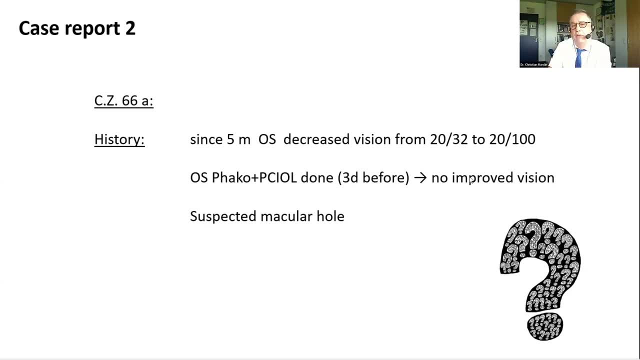 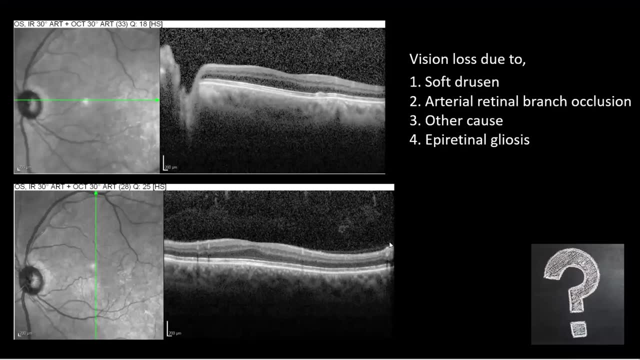 and FACO PCI-OL was done three days before. vision did not improve And it was a suspected macular hole in this patient. So I will I show you the OCT scan of the left eye and I would ask you again the vision loss. 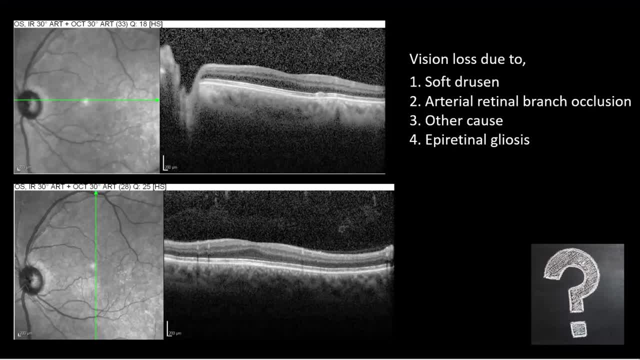 of this patient. when you look at the OCT of our patient is due to soft drusen, an arterial lateral branch occlusion. any other cause or epiretinal gliosis. What do you think You may vote now again? 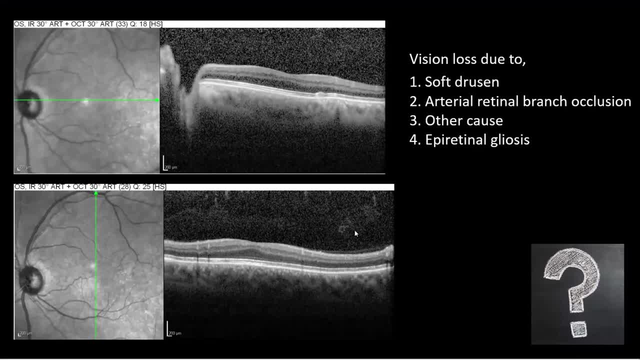 You have 30 seconds time. Again, on the left-hand side you have the infrared image. You have a horizontal and a vertical high-resolution scan. The scan is a little bit blurred, but all the structures can be seen easily. Yes, 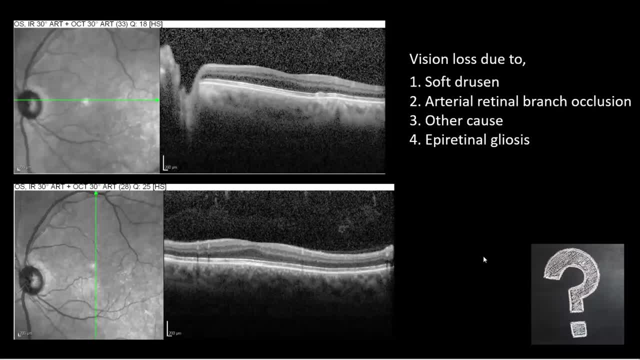 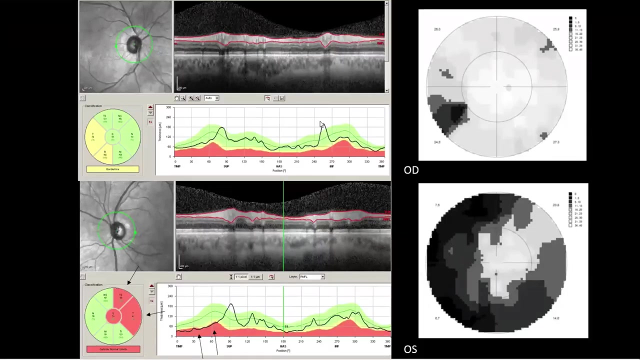 And this polling fits quite well to the case. It's nearly equivocal for all options and majority may ask for other cause And in this case the majority, as always, is right and we have a look at the patient. So when you look at the optic nerve head a little bit more nasally, you will realize. 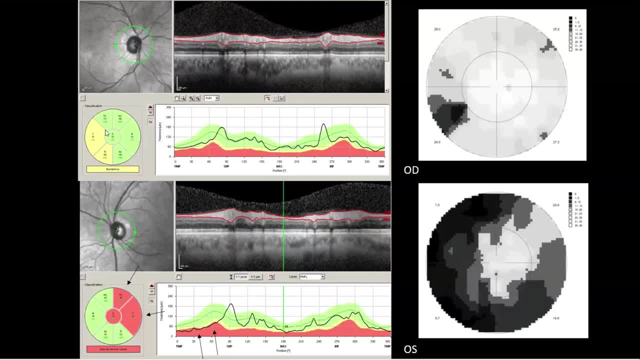 with your OCT that on the left-hand side more than on the right-hand side, you have an atrophy of the retinal nerve, The retinal nerve fiber layers. Of course you do a visual field and you'll see on the right-hand side slight defects. 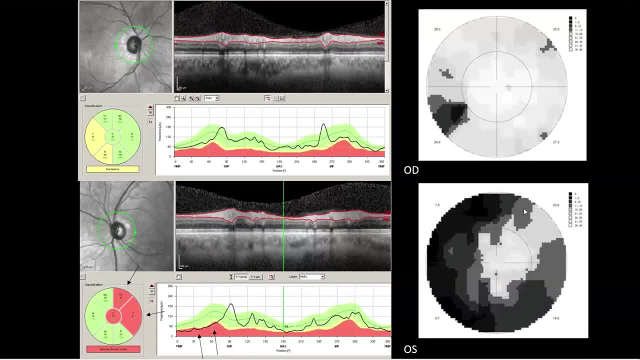 of the visual field on the nasal side, but on the left-hand side you have a nearly circular loss of visual field with a preserved center. And here we have to ask the question why the patient has an optic atrophy. The most common cause is the retinal nerve. 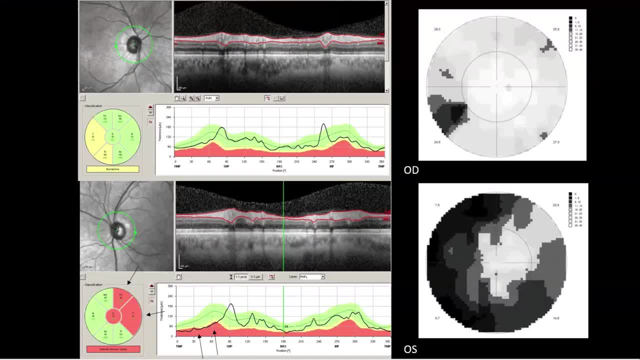 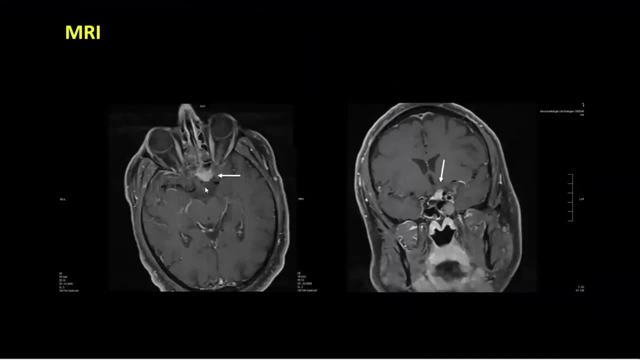 The most common cause, of course, is glaucoma, And often glaucoma prior to cataract surgery is not known or overseen, But in this patient it was unfortunately a midline meningioma And this was the reason why the patient had a bad vision. 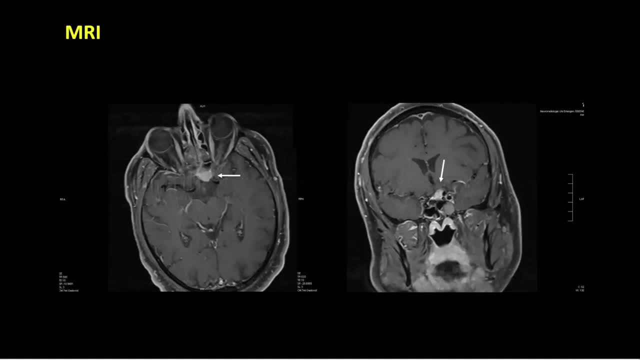 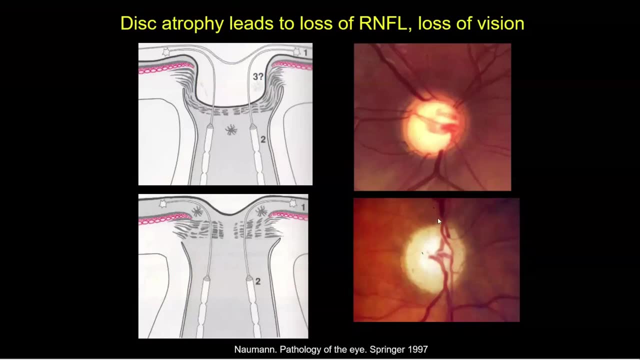 And therefore cataract surgery did not help the person much So. disc atrophy, either to glaucoma or to any other cause, causing simple optic atrophy and painless optic atrophy. This is due to nerve fiber layer and ganglion cell loss. 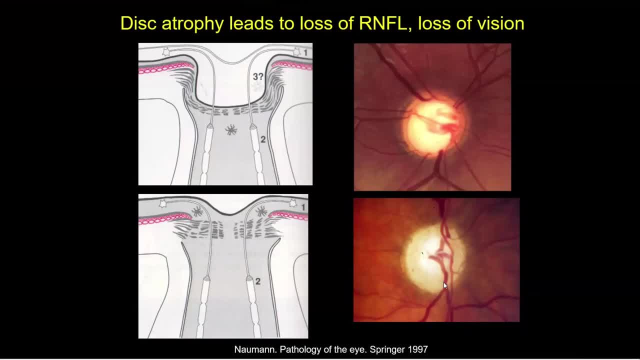 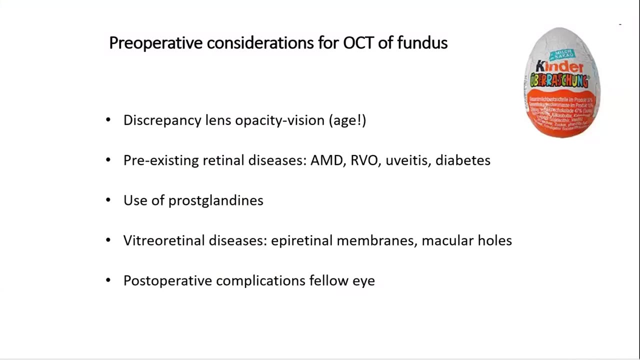 And we will discuss that in extenso in July in another talk. But this causes loss of vision, not related to cataract, but can easily be found out with the OCT scan. So two take-home messages for you: The preoperative consideration for an OCT of the fundus. you can't do it in all the 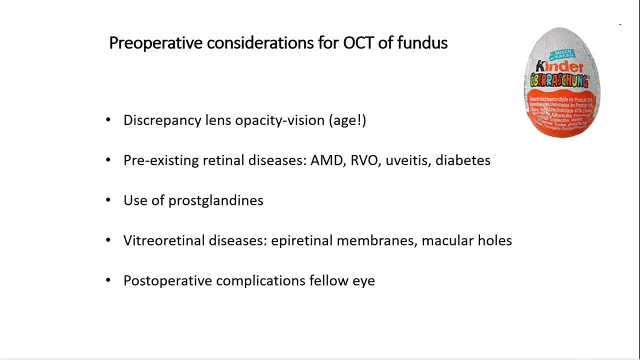 patients, because the workflow does not always occur. But if you have a discrepancy between lens, opacity and vision, especially when you consider age, as in our 15-year-old girl, then you have to ask yourself a question: whether the reason is not at another place: fundus macula or optic nerve head. 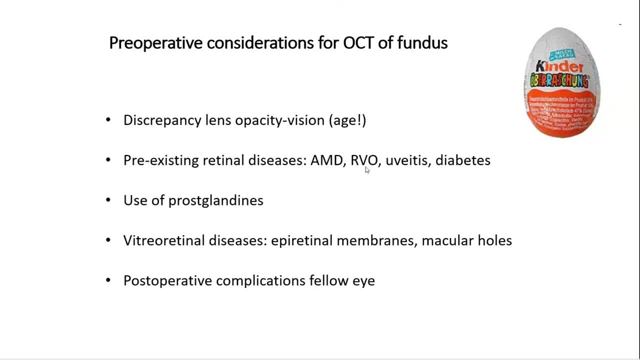 Pre-existing retinal diseases- AMD, occlusion of retinal vessels, uveitis, diabetes- should give you an idea. The OCT scan would be helpful, especially when you think about antiretinal or steroid therapy prior to cataract surgery because of CME. 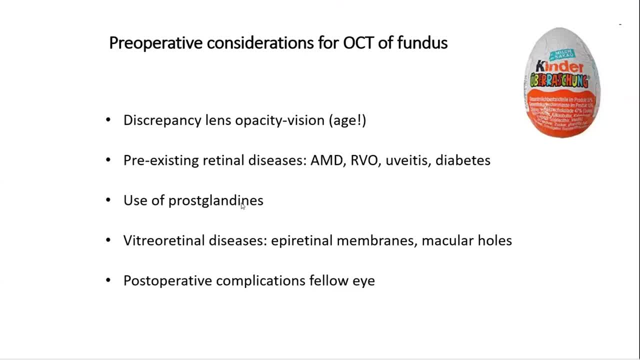 Use of prostaglandins, sometimes in cataract patients, may cause CME- Vitreo-retinal diseases like membranes and macular holes, of course, And this can easily be depicted with the OCT. And, of course, if you have postoperative programs, I personally use my positional OCT for the 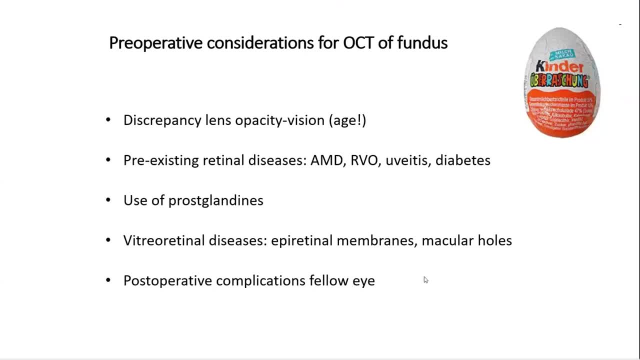 OCT complications in the fallow eye, then it's always good to get the time and to have the time to do a good workup of the eye prior to cataract surgery and look whether the patient has also another disease. So what can you do? 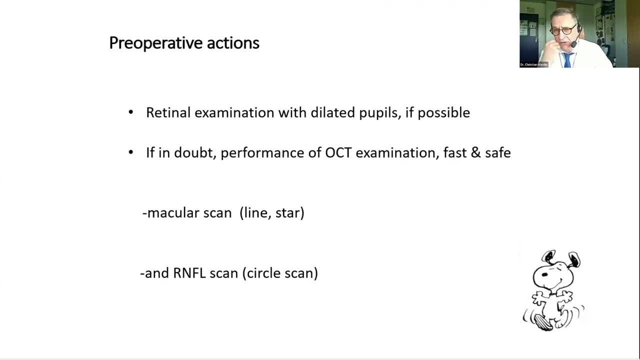 Of course an urgent examination with dilated pupils is possible. But if you are still in doubt, a performance of the OCT examination is very fast and safe for the patient. You can do a fast macular scan, horizontal, vertical or star scan. 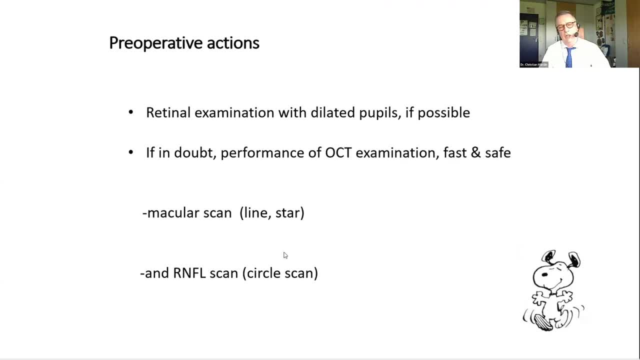 You do the nerve fiber scan in a circle scan around the optic nerve and also with ART, even in children. possible very fast and gives you a lot of information, Very helpful to avoid all the scenarios I have shown you in the cases before. 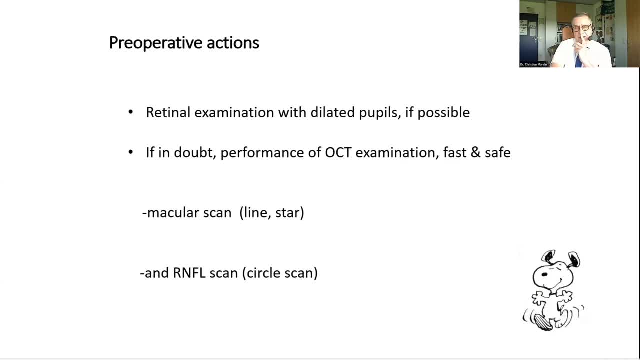 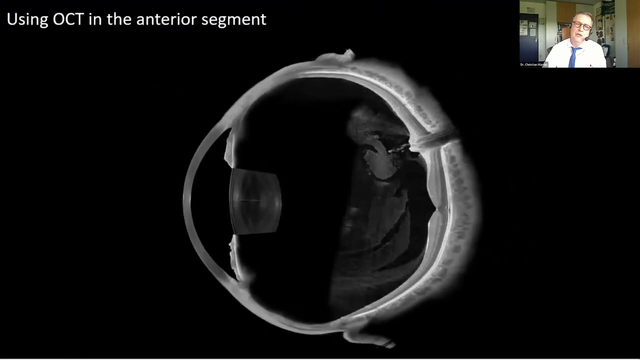 Now we have discussed in detail patients with fundus problems in the preoperative phase of our cataract surgery, But we can also apply modern OCT devices on the anterior segment And of course also in the anterior segment it can be very helpful to get high resolution. 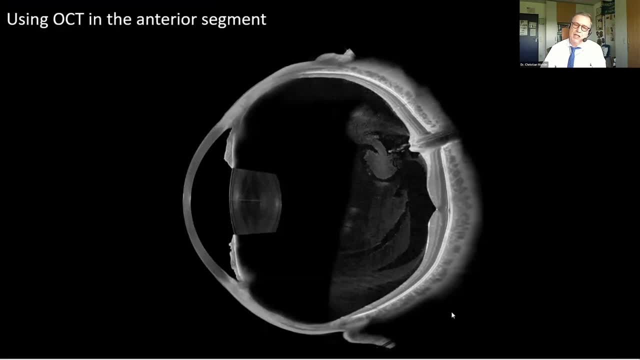 images. This is still a montage And not the reality, But perhaps someday we will be able with the OCT scan to get with one scan such a nice image of the eye with a detailed posterior and a detailed anterior segment. And about this scanning of the anterior segment and the implications we will discuss in the 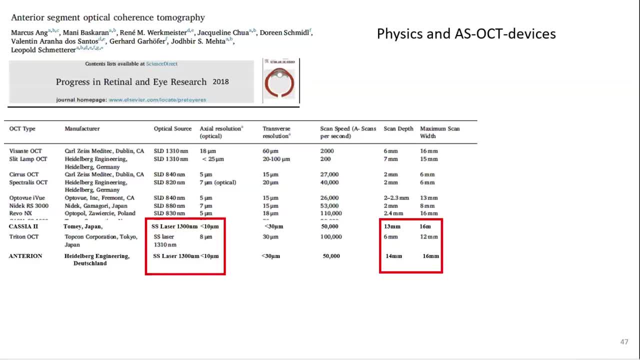 next 15 minutes, The anterior segment. OCTs have developed a lot And nowadays the sweat source technique- And in fact this is also really a specific question- is key, and the swept source technique allows you a very deep imaging of the anterior segment. 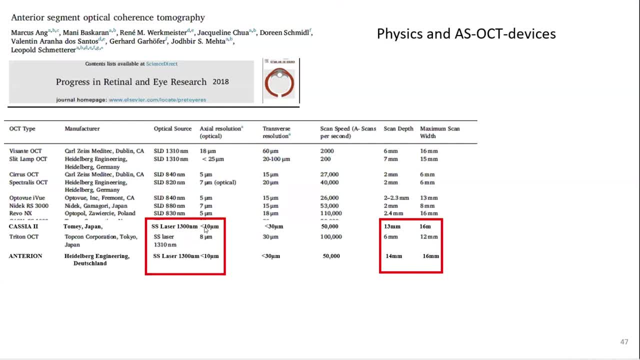 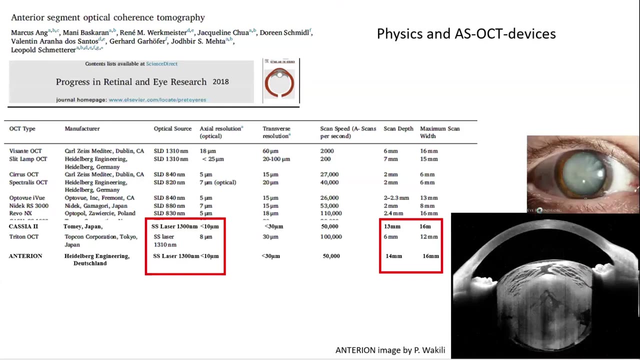 behind the lens And, if you realize, here we have a longer wavelength with the spectral domain devices from the past and the longer wavelength allows us to go deeper into the tissue and get more detailed images from the depth of the tissues. This is a very impressive example of a mature cataract where the whole lens could be imaged. 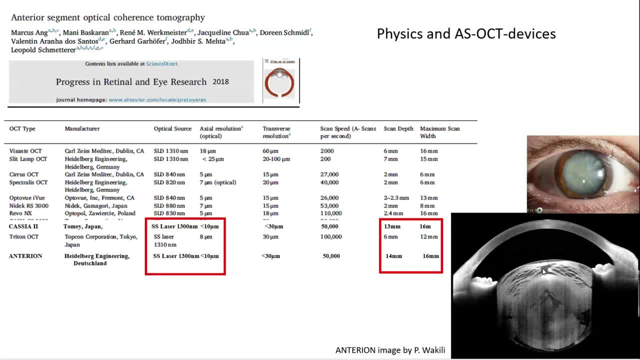 in its beauty and in its horror for the surgeon prior to surgery. This is a very nice image from the colleague of Philip Vakili, here from Germany, and this indicates that the longer wavelength of the laser is able to image even this wide opaque lens in total. 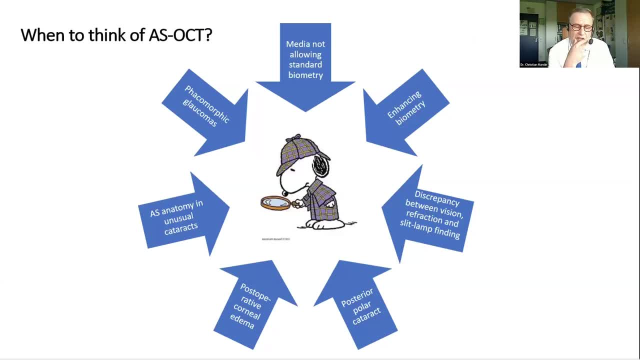 Okay, So anterior segment OCT is not always available when to think of, especially if the media are not allowing a standard biometry, for example, If you have phagomorphic glaucomas, if you want to enhance your biometry with premium. 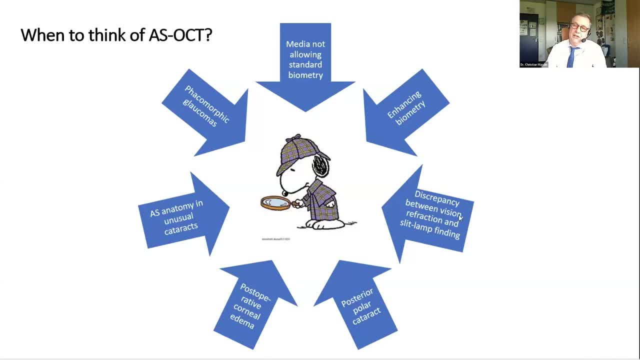 lenses used. for example, if there's again the discrepancy between vision refraction and slit lamp finding posterior polar cataracts can be. anterior segment OCT be very useful. Post-operative corneal edema or just the anterior segment anatomy, if you're unusual. 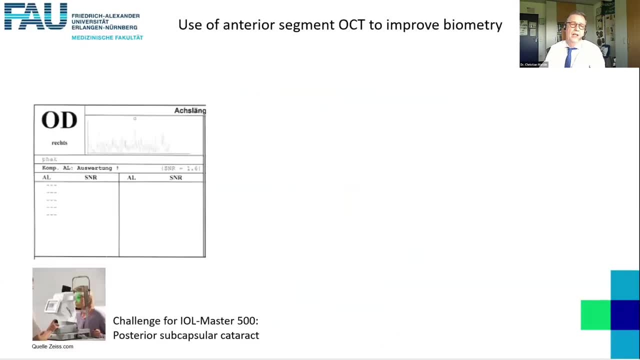 have to encounter unusual cataracts. So this is an example of a subcapsular cataract biometry where our workhorse, the IOL Master 500, couldn't find the right peak and do the right measurement. With ultrasound sonography A-scan immersion technique, of course, you are able to measure. 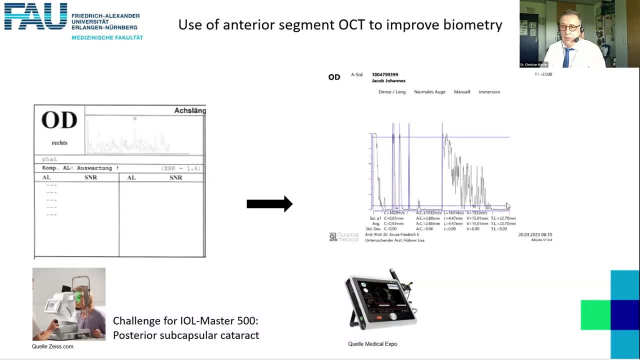 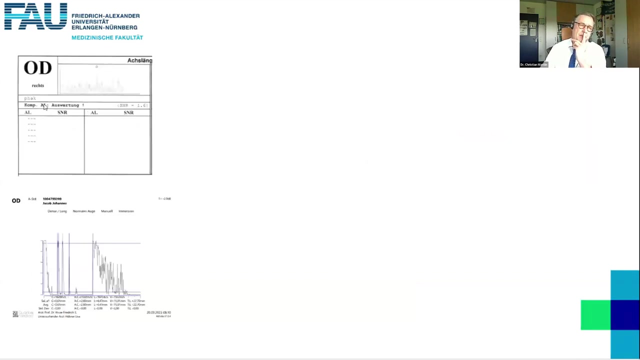 and perform in these patients biometry, axial length measurement, all the other measurements you need, But you have to take the patient away from your workflow and lie him down and do the immersion biometry with A-scan. But when you compare these measurements- our IOL Master 500, our IOL Master 500, our IOL. 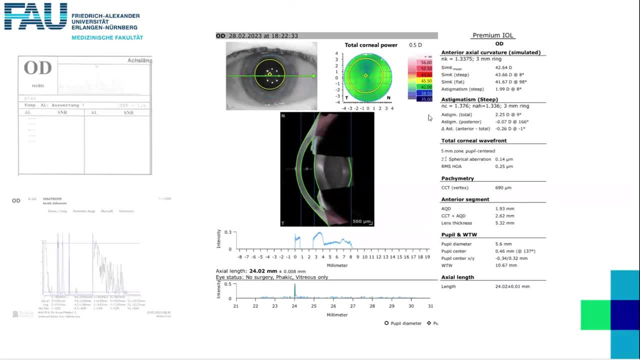 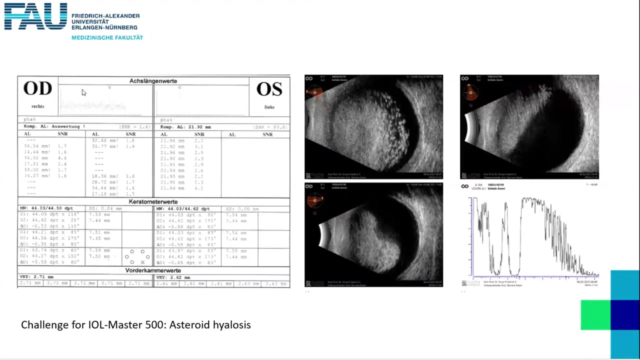 Master 500.. You will notice the those are those close ups. They're almost identical. Question 500, is not able to find the right peak in the laser measurement is due to asterotiolosis- a real pain- And this may cause also problems when you do the A-scan. 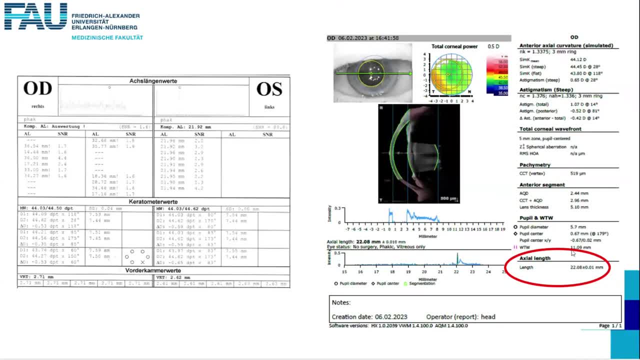 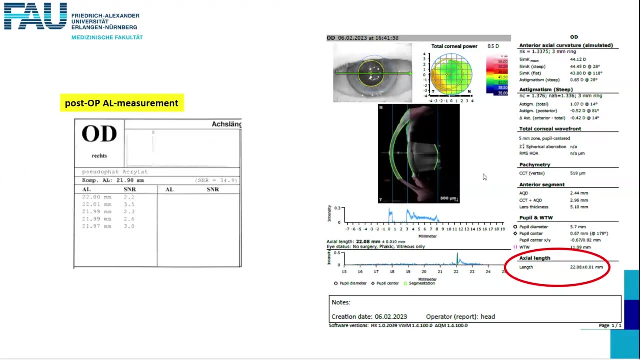 When you look with the anterior again, with the longer wavelength, you get quite a nice measurement of the axial length, rather precise, And then you can perform a normal standard biometry and lens calculation as you wish. In this patient after cataract surgery we measured with our IOL master again the axial. 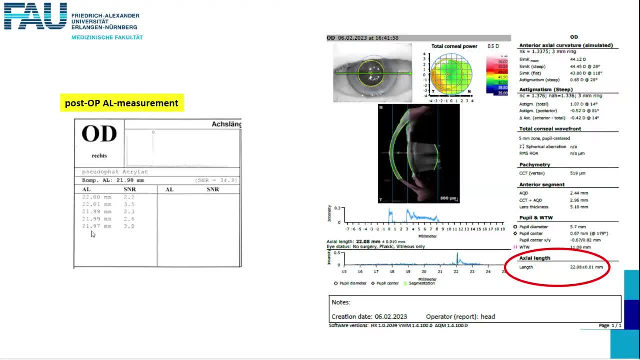 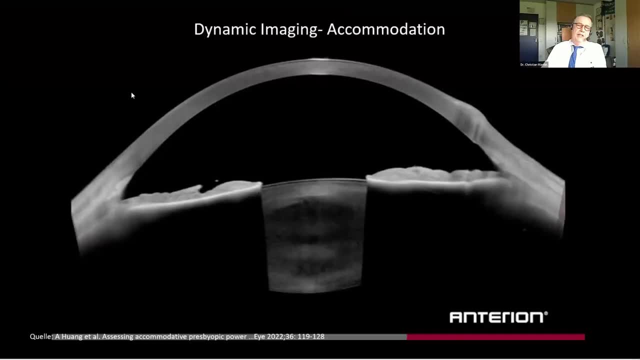 length of our eye And you see the measurement after surgery and prior to surgery very close together. This is a very nice GIF from Alex Wang. We're in the United States showing a patient who is accommodating six diopters And you see in vivo life that the lens becomes thicker during accommodation. 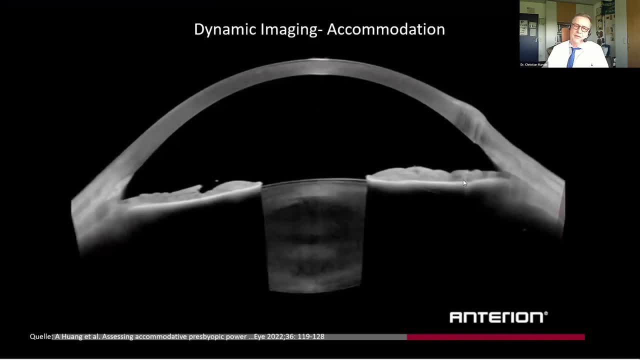 The lens wall changes And of course, the iris position and the anterior depth changes. The aperture of the pupil changes by 30%. That's quite impressive And gives us A nice idea about the high-detailed imaging we can do in the anterior segment. 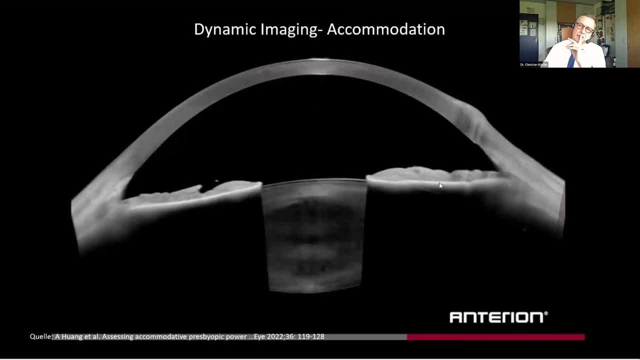 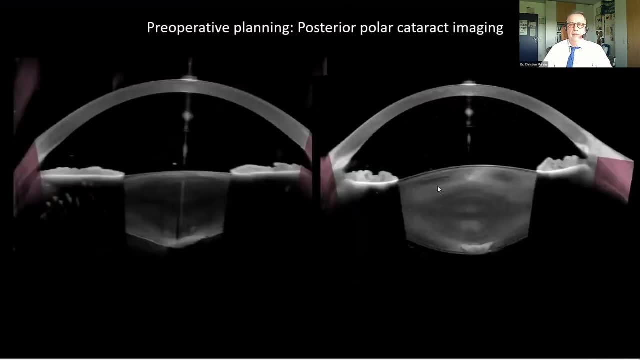 But it also shows the drawbacks of the laser. It can't penetrate the pigment epithelium of the ciliary body and the iris. Here a posterior polar cataract. Two patients I had to do surgery on. Both patients had on the slit length a posterior polar cataract. 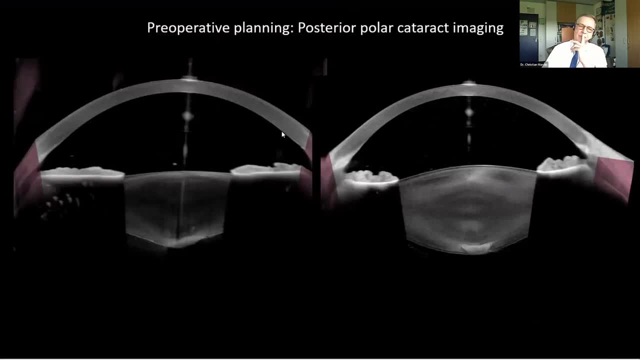 So we went to an anterior imaging Here. in this patient I expected and had the capsular defect during surgery. Here I did not expect the capsular defect And I had no capsular defect during surgery And in this fashion I was prepared what to expect to do the surgery. 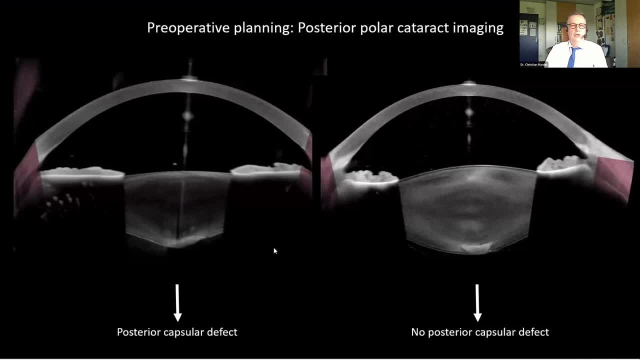 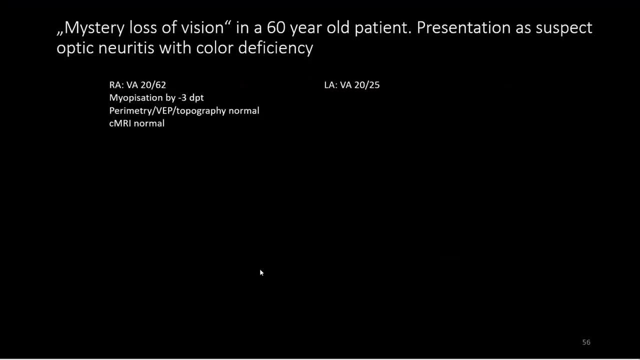 And could adapt my technique during surgery to avoid major complications due to the rupture of the posterior capsule. Here a patient with 60-year-old with a mystery loss of vision And he presented with a suspect optic neuritis with color deficiency and a reduced vision. 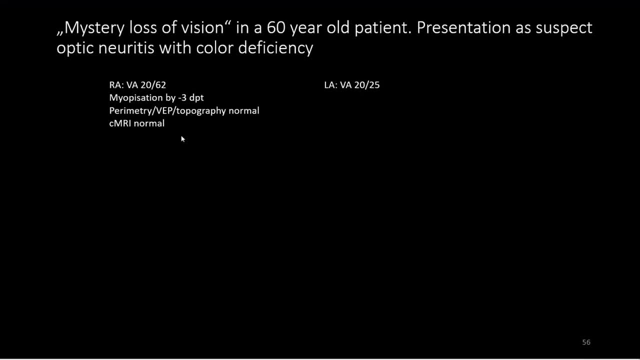 He showed a myopization minus three diopters Perimetry. VEP topography of the cornea was normal. Even MRI scan was done before and was normal. Now we have a look at the anterior segment: OCT pictures. 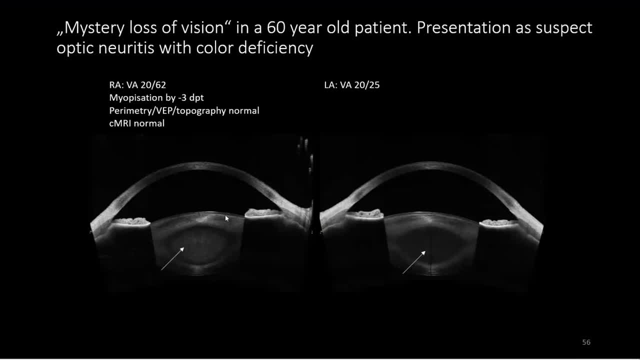 And we realize That in the right-hand eye, with the complaints, we have a slight opacification and densification of the nucleus, Causing of course a color deficiency And causing a myopization and vision loss. This is the comparison to the better eye, left eye, where the opacity is not as dense as in the right eye. 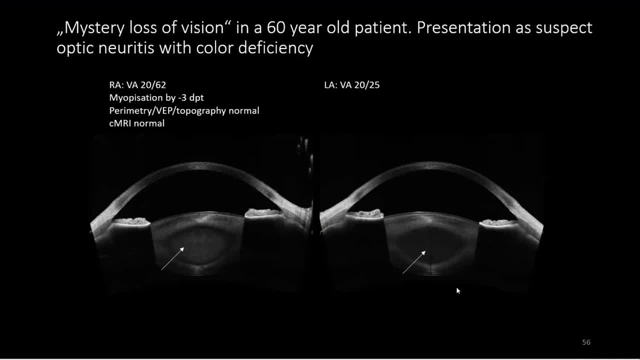 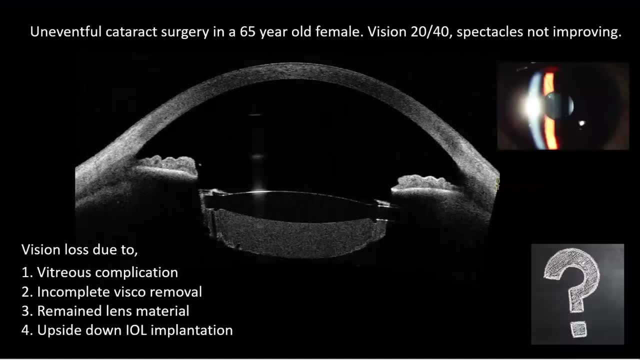 But the sclerosis of the nucleus is similar in both patients, So these phenomena can easily Be explained with the right OCT examination. Here we have an uneventful cataract surgery in a 65-year-old male, But with spectacles after surgery, vision could not be improved. 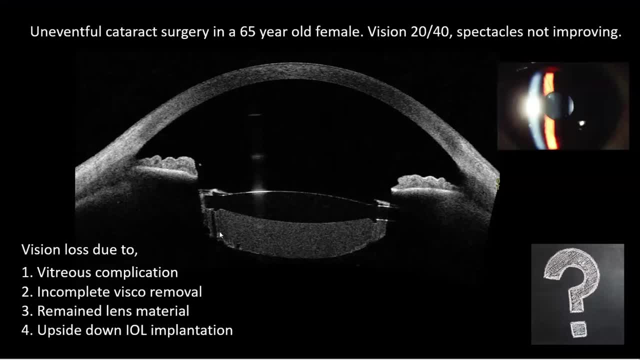 I show you this picture and ask you showing this OCT picture, why is vision loss present? Vitreous complication, Incomplete visceral removal, Remained lens material Or upside-down implantation Or fibrosis Of the IOL in the capsular back? 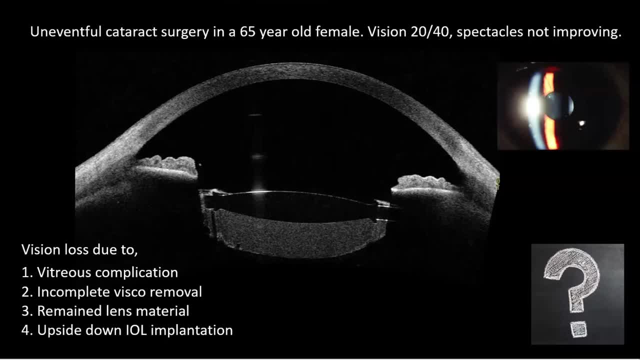 What do you think? I think this is the easiest of the questions, Because the anterior segment, OCT, gives us such a detailed image. Yes, majority is for upside-down implantation, But 21% for remained lens material. This is not Too bad. 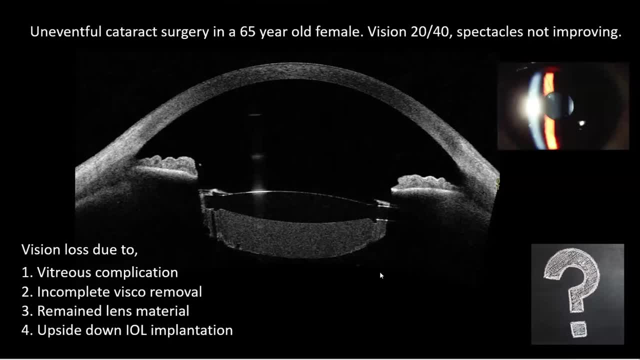 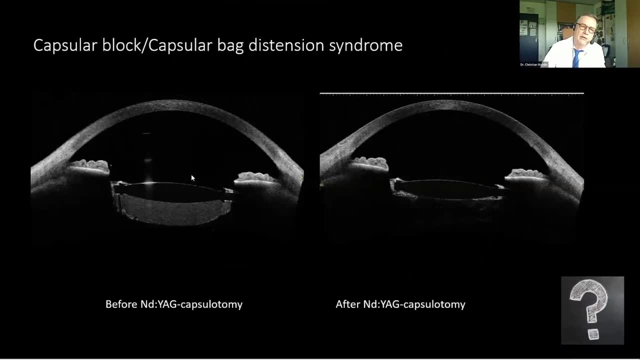 Let's have another look at the patient. The patient has, after the uneventful surgery, perhaps a very small rexus, a residual hyaluron in the posterior capsular back. It's a capsular distension syndrome And these patients are not able to gain full vision until you do a YAC capsule to me of the posterior capsule. 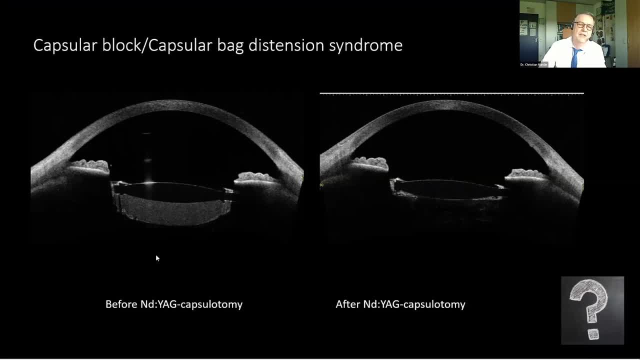 And then the viscoelastic hyaluron is released in the vitreous space and then the optics are restored again and the patient is able to see with full vision. Sometimes and often you appreciate that at the simple examination, but sometimes you are not able to see it. but the OCT is able to see it. 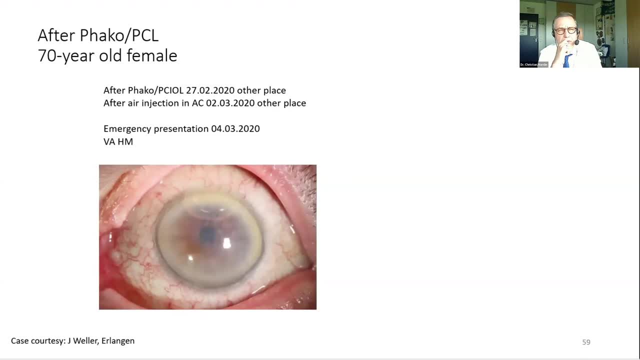 This is a patient after a FACO with posterior capsule IOL, And this This patient was done in another place When he, at the time of presentation, vision was rather down half movements. There was an air bubble in the anterior chamber and a very opaque and decompensated cornea. 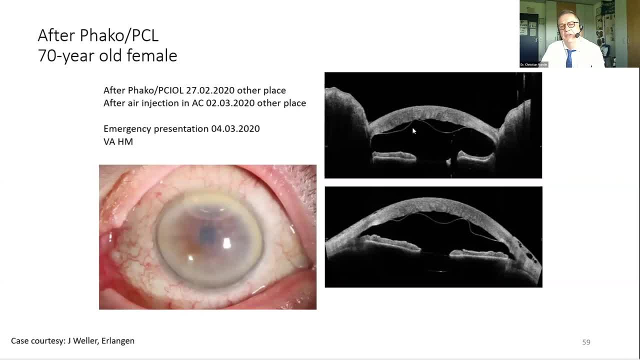 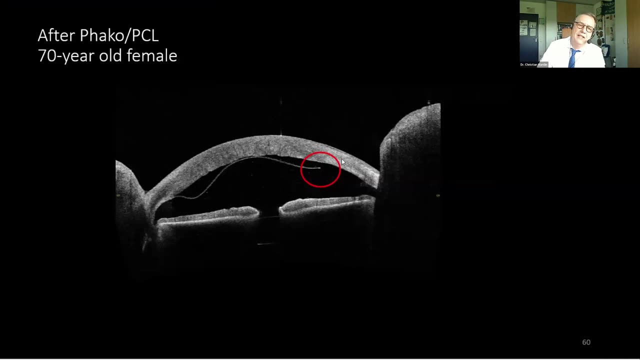 When we look at the OCT scan in the anterior segment, we see that there is a loosening of the decimet, nearly total, causing the edema of the cornea. And this is the 12 o'clock position where the surgeon entered the eye. and you see that you have here the beginning of the decimetolysis, causing a lysis of the whole decimet. 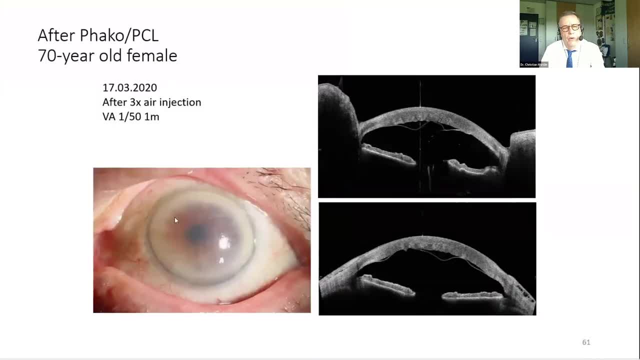 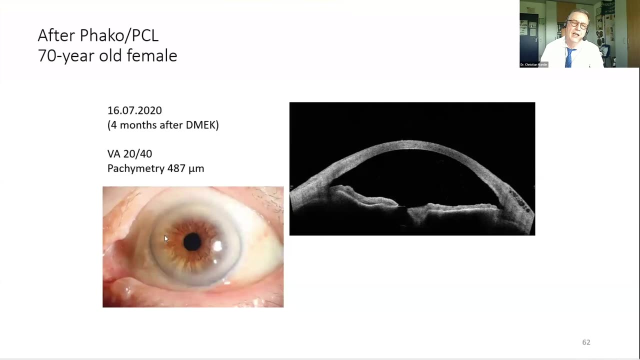 Now when you look at the patient, we tried several times air bubble injection- three times did not help much- and then had the indication for DMAG. After DMAG everything was fine again And of course- a nice technique- clear cornea. again attached this new decimet. 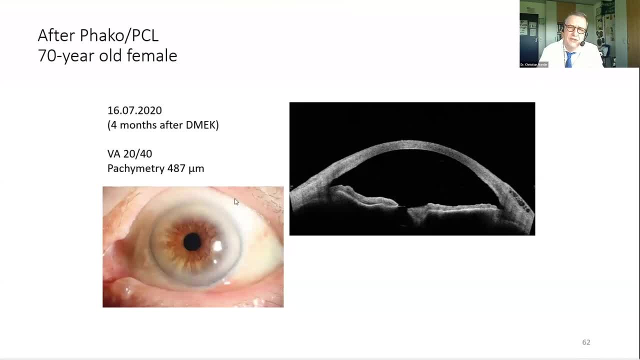 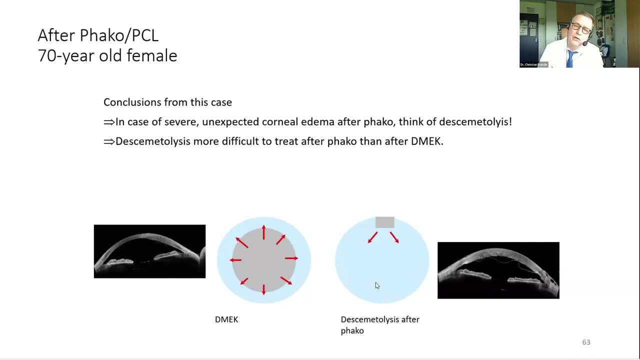 And the difficulty with the decimetolysis after cataract surgery is that you have just a very small tunnel for fluid to escape the area under the cornea. This may not happen just by air injection. It's easier after DMAG when you have a detachment to attach the transplant. 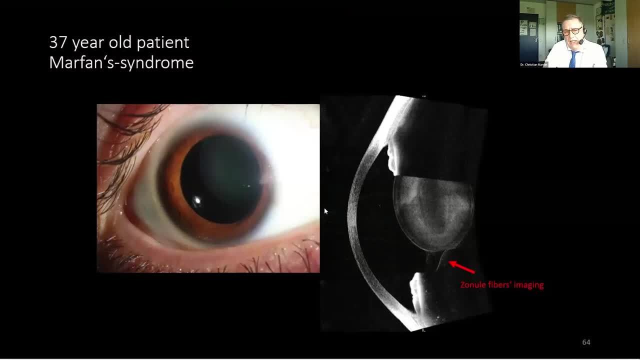 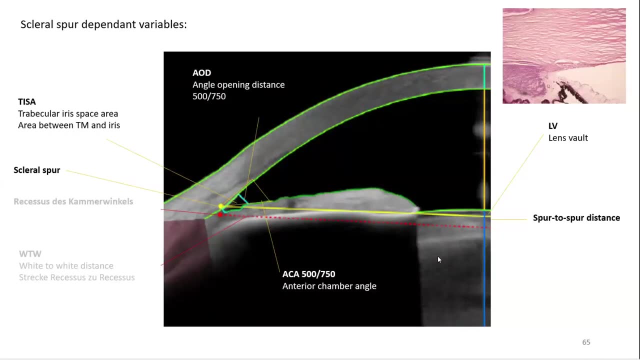 And then you can look at the OCT scan. and then the OCT scan. you can see the decimetolysis with the air bubble. Here you see a patient with Marfan's syndrome with dislocated IOL beautifully depicted here, the zonule fibers. 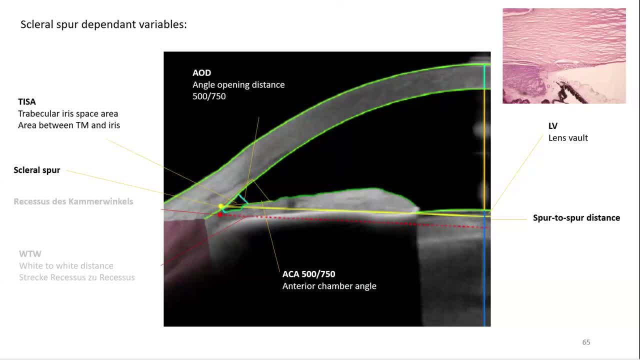 In phagomorphic glaucoma it's important to measure the anterior segment And here you have all the modalities with anterior segment OCT, giving you the right measurements to describe your chamber angle And key is to determine the angle of the chamber. 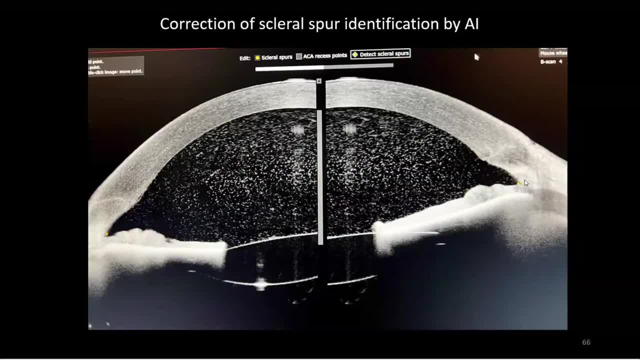 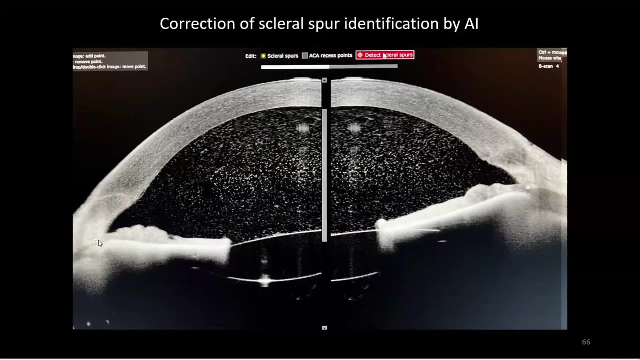 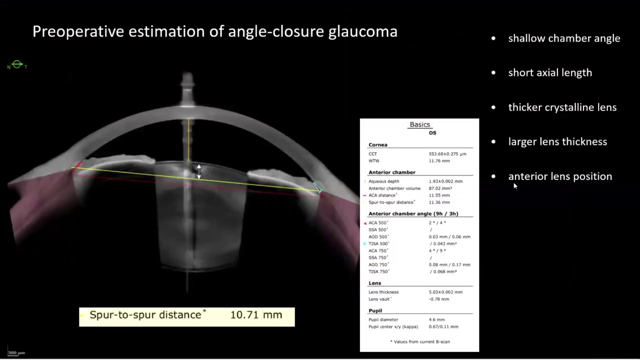 detect the scleral spur here- And this is a patient where we thought the sterile spur would be because it was not quite easy from the image quality to detect it. but with AI in the anterior, the machine showed us the right place of the scleral spur and then we were able to do the right measurements. 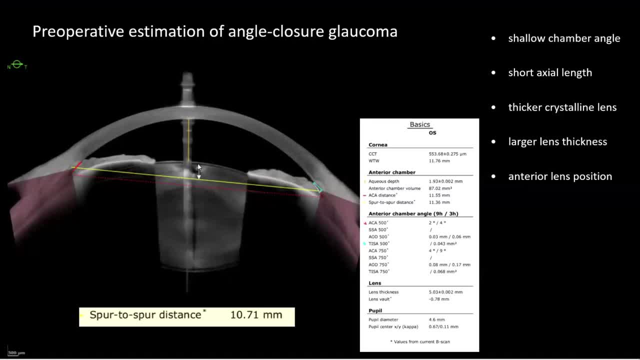 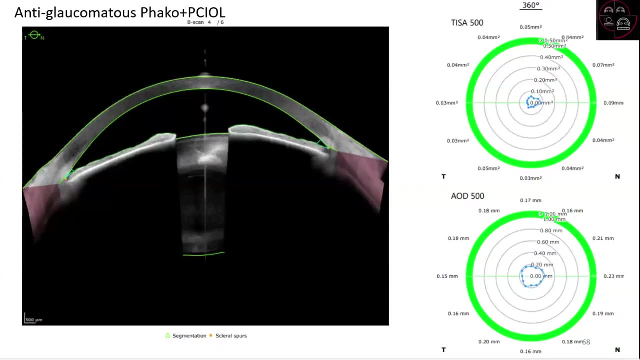 One of my favorite measurements to estimate whether an angle block may be imminent or not is here the lens vault. So it's a line between the scleral spurs and the distance to the surface of the lens. This is a patient with an anti-glycomatous phaco PCIOL. 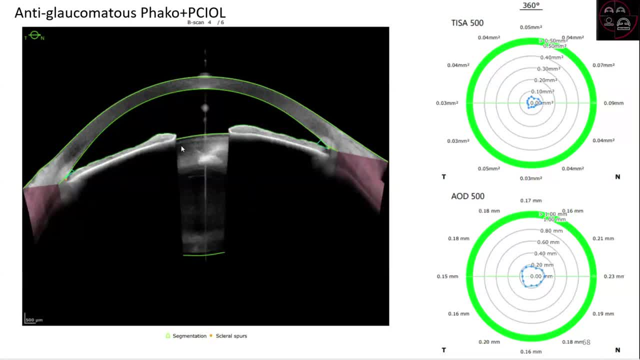 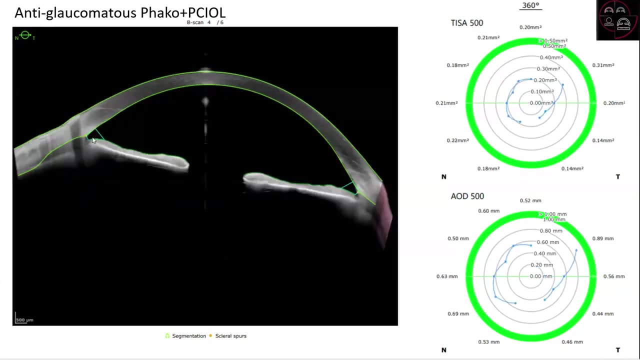 You see the narrowed chamber angle, the large lens and the flat anterior chamber. These are the measurements of the chamber angle prior to surgery, with a polar diagram delivered by the OCT device. And after surgery, the chamber angle is open again. IOL is in place. the chamber is much. 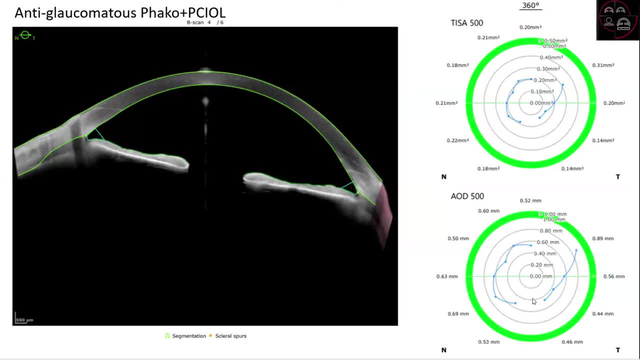 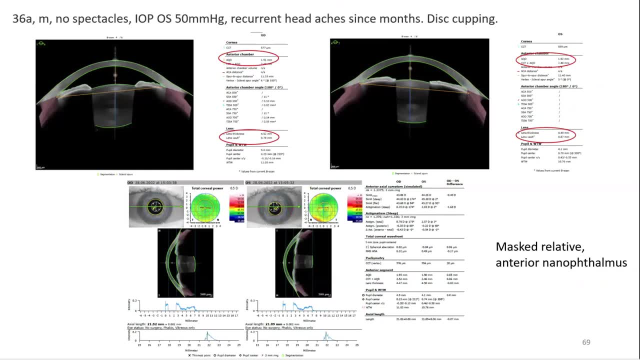 deeper and the polar diagram shows change values towards hinting towards an open chamber angle. again. This was a curious patient, rather young, wearing no spectacles, no refractive lenses and no scleral spur, But the IOP was 50mm mercury with an acute pupillary angle block, and this was recurrent. 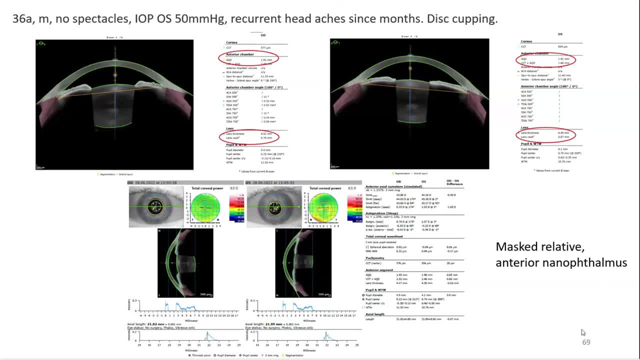 since several months and the patient already had a disc cupping. But the patient was not hyperopic. but at the SIT lamp we realized that the anterior chamber was rather shallow, the lens was rather thick and this can easily be appreciated. 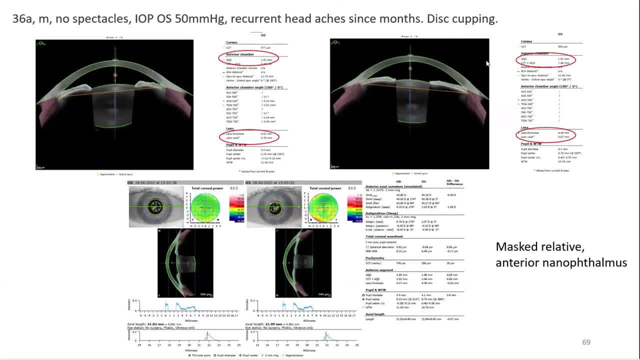 with the anterior segment scan showing the depth of the anterior chamber in both eyes and the lens thickness in no relation to the space in the anterior chamber. So it's a relative anterior non-ophthalmos and the axial length was measured also by. 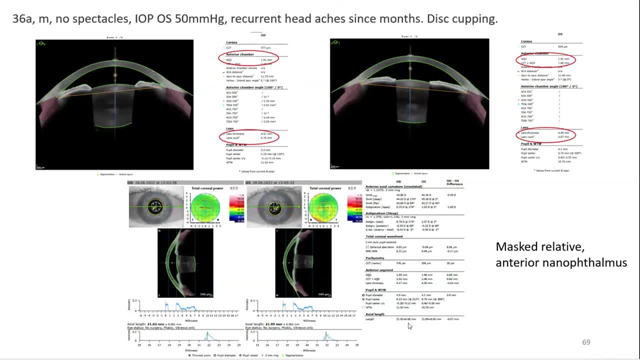 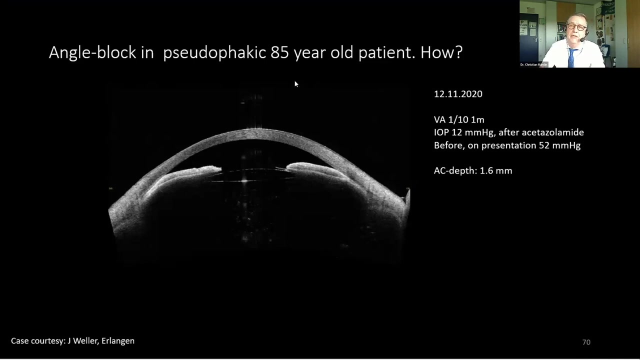 the same device: 21.8mm, a little bit shorter, but the hole was a little bit disguised by a little bit steeper corneal measurements. So all this information can be done in one scan with the anterior segment OCT. This is a patient with an angle block in pseudophagia, 85 years old. 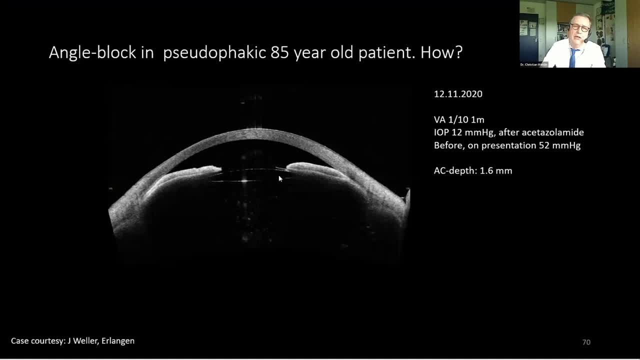 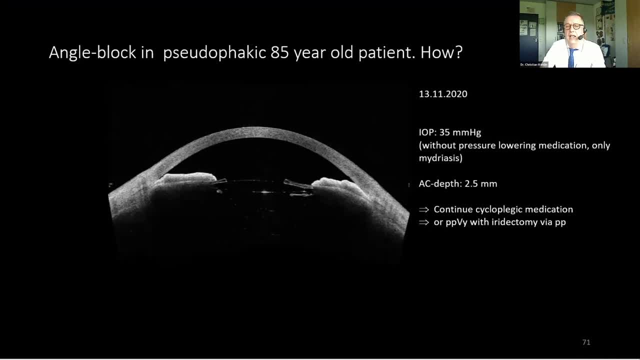 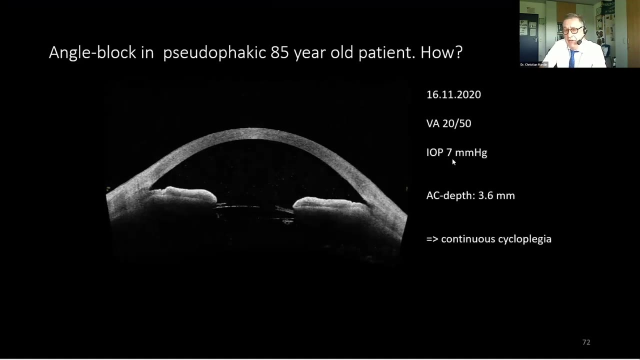 We've done this, We've done this, We've done this, or pseudofecal block to be precise, And we were able to deepen the anterior chamber just by cycloplegia, and the IOP afterwards fell also down and to a very low pressure, without any other medication. 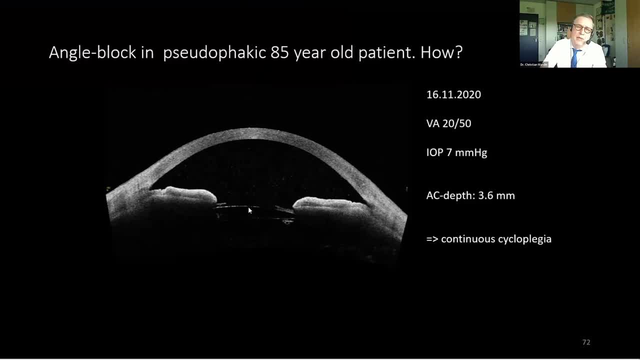 The patient was elderly, therefore, and was not disturbed by the a little bit wider pupil. Therefore, we decided to continue with the eye drops. A second option would be to go via pastana and do a corvitectomy. do your iridectomy a zololectomy. 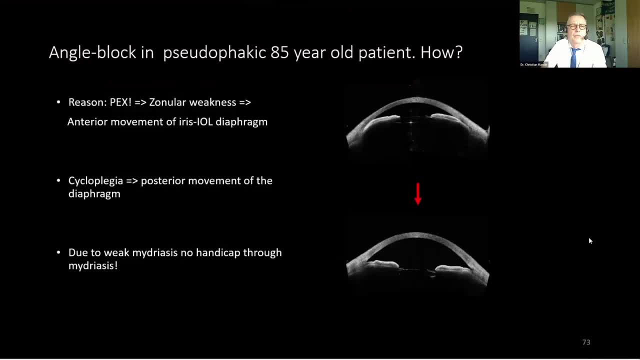 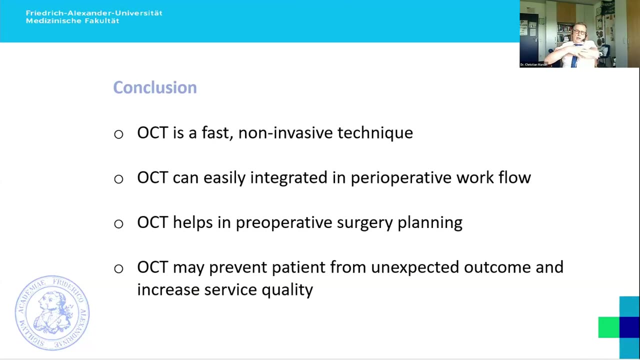 and then the anterior chamber can be deepened. also, The reason for this was pseudoexfoliation syndrome with a very weak sonula and anterior displacement of the whole diaphragm. So, in conclusion, another fundus and anterior segment OCT is a fast and non-invasive technique. 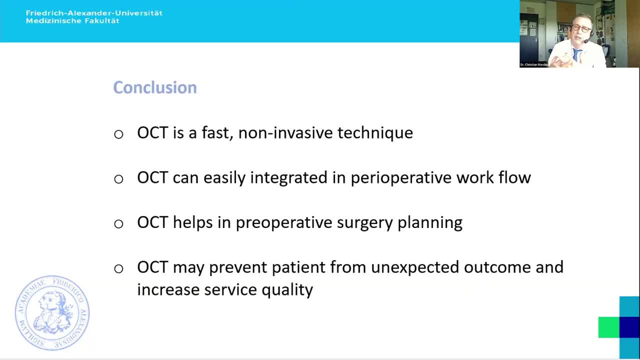 It can easily be integrated because it's so fast in the perioperative workflow. You have to think of it to do it. OCT helps, as you have seen, in preoperative surgery planning, and OCT may prevent patient from unexpected outcome And, of course, increase our service quality for the patients. 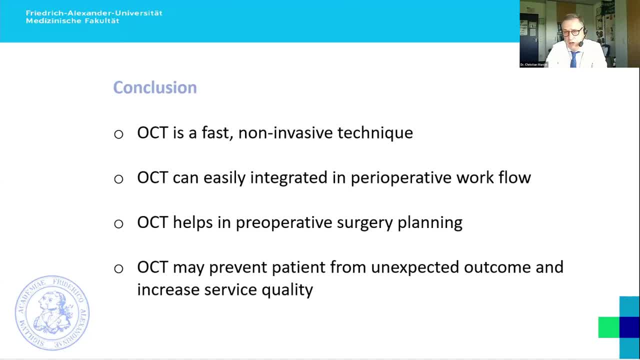 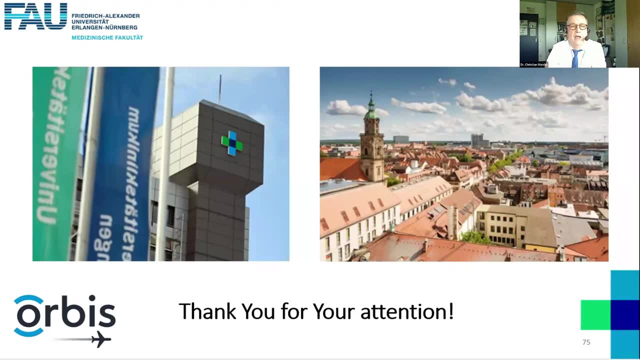 With this last slide, I would like to say thank you very much for listening, listening, and I would send my kindest regards from Erlangen, in Bavaria, in Germany, where our small University Hospital is, and now I'm looking forward to questions from the discussion. thank you. 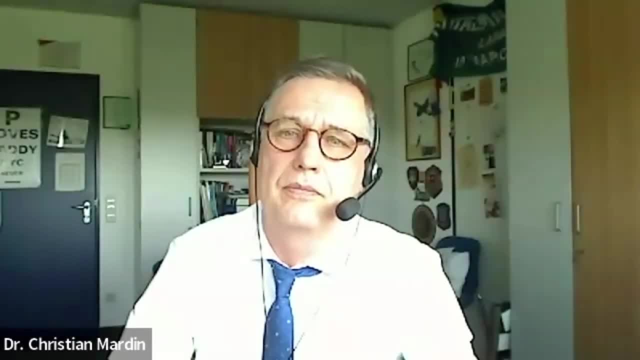 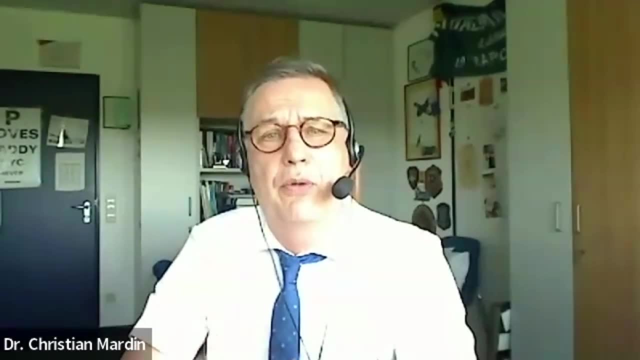 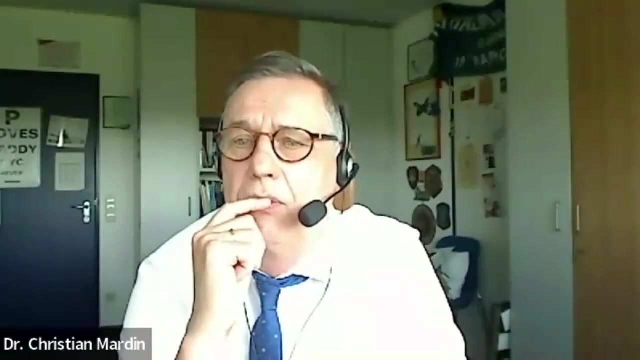 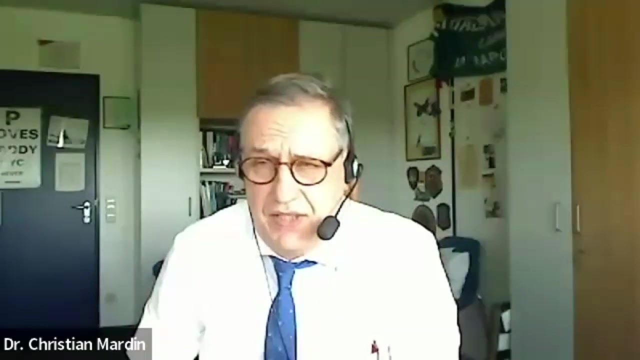 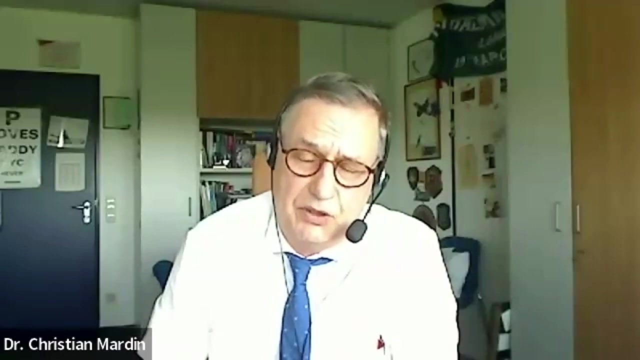 very much. so I would read the first question to you: can we opt out cataract surgery merely OCT features in a patient with dry AMD? if you look on your OCT's high resolution OCT scan at the formation of the outer photos, outer photoreceptor segments or ellipsoid zone, and if 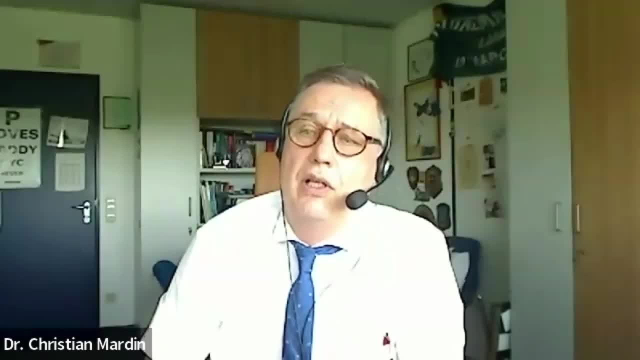 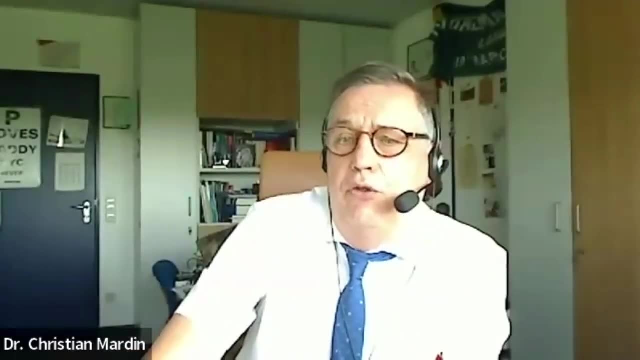 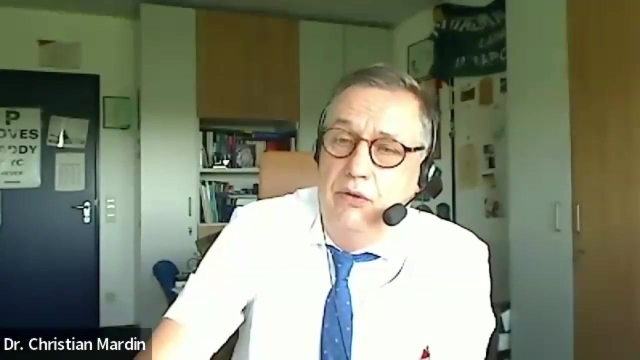 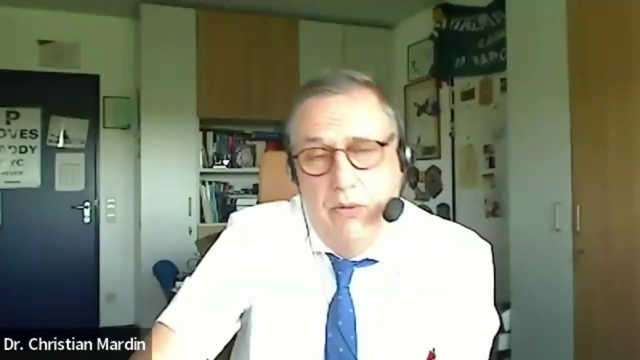 they are present, then it gives you a good idea that the vision will not be too bad after surgery. the second question is: with the current and future advances with special swept source OCT and more infrared laser imaging, will a scan still remain relevant? yes, especially in very dense vitreous hemorrhages, where you want to. 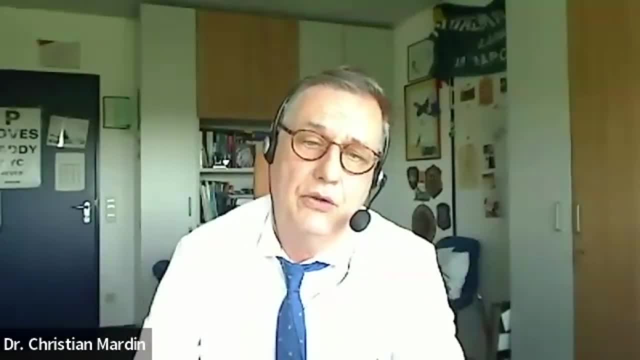 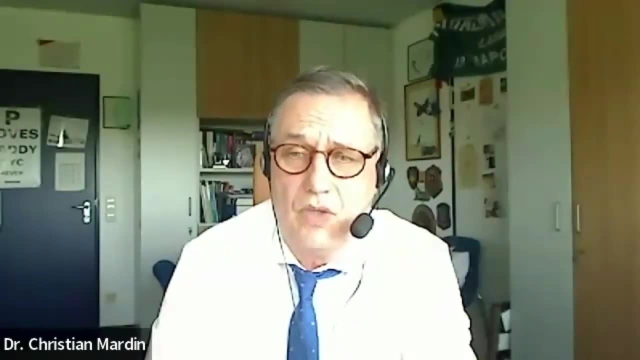 combine vitreous surgery with cataract surgery when you need a good measurement, and then a scan is still the best thing to do. yes, I think we might use less a scans as we did in the past, but I think it will not be obsolete in the future. 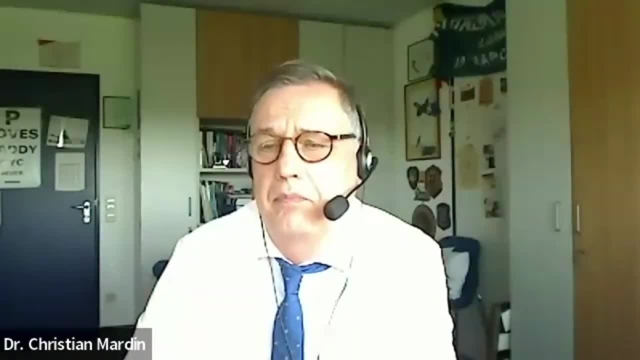 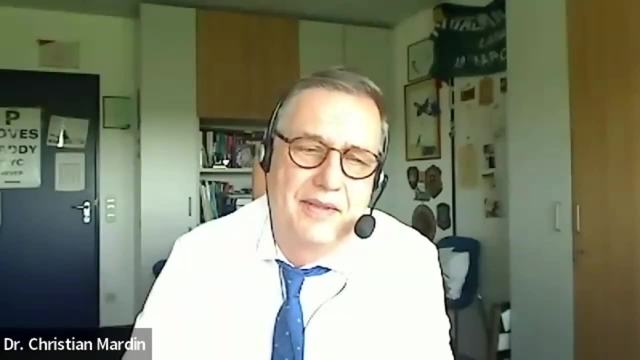 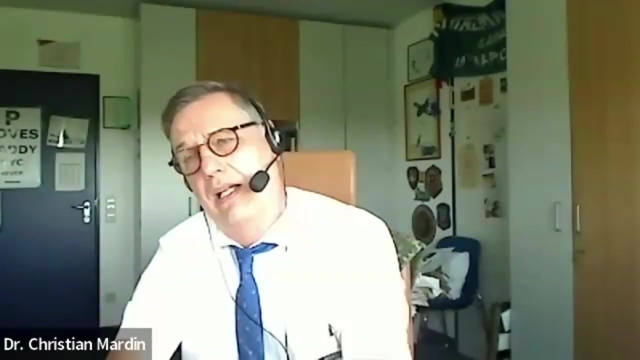 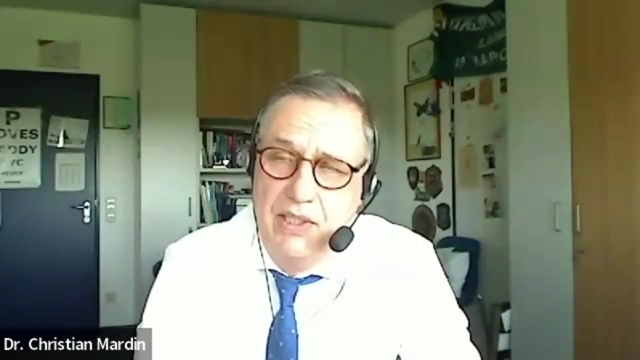 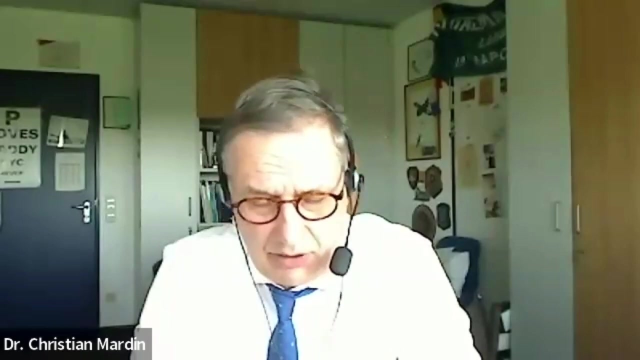 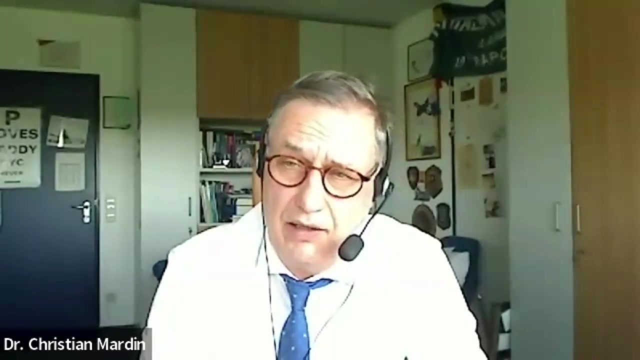 another questions. I go back. how much does OCT add to the cost spawn by the patient? this this depends on the healthcare system in our place. when the patient comes as an outpatient, you get us the same amount of money. um, irrelevant how many examinations to do in the private practice, in the private sector, when you 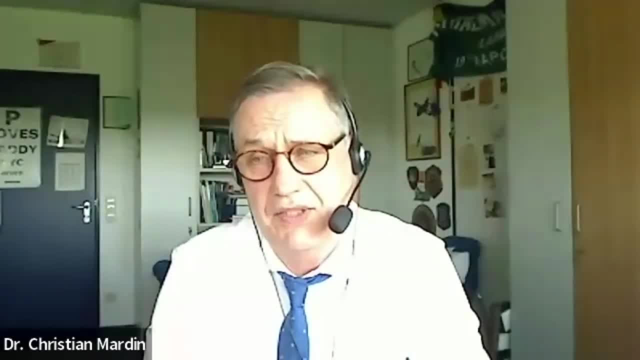 have to charge money for your OCT scans. but I think if you explain the patient's the advantages to do the OCT scan where we're willing to pay, and I think it's it's, it's tough if we're we're, you're okay and I think it's we're okay. I think I think you really need a humanチ sẽ việc là. 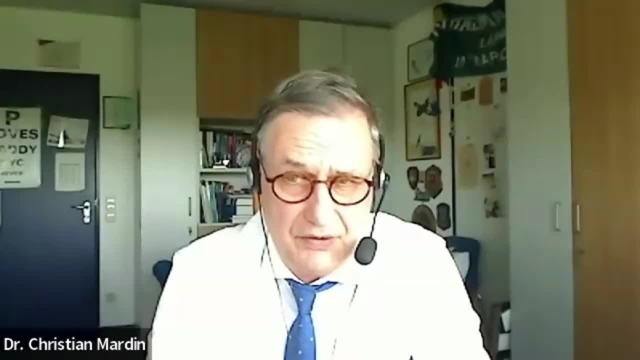 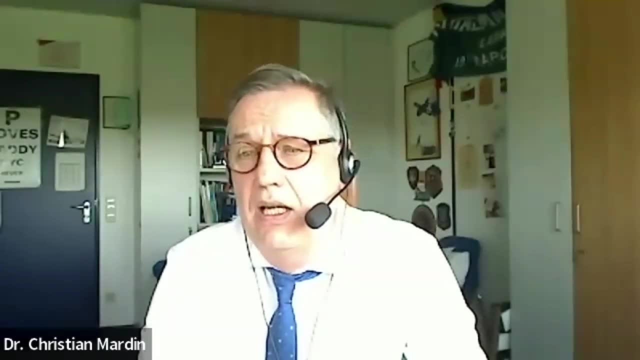 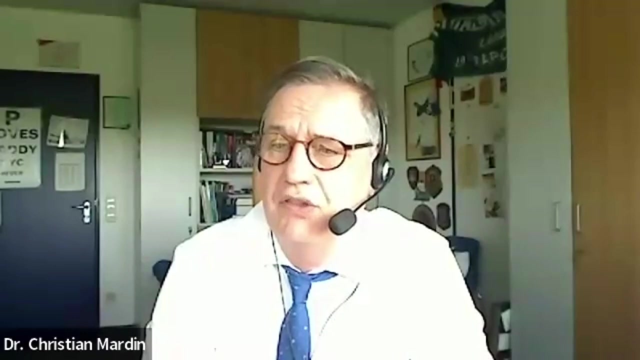 ease để sở��. chứ depends on your health care system and an reimbursement. The next question in OCT posterior capsular opacity: OK, it doesn't continue. The next question would be: would you suggest having an anterior segment OCT image? 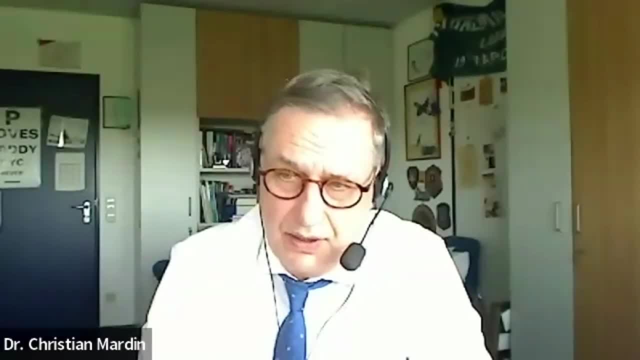 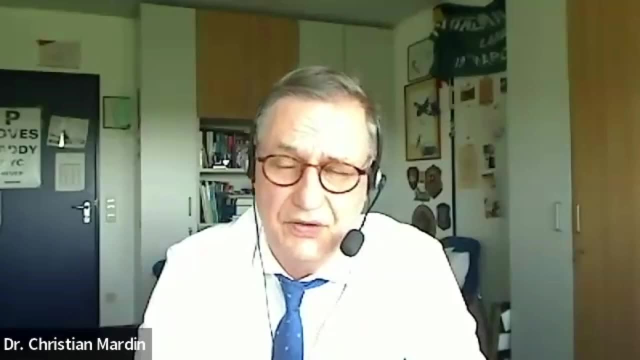 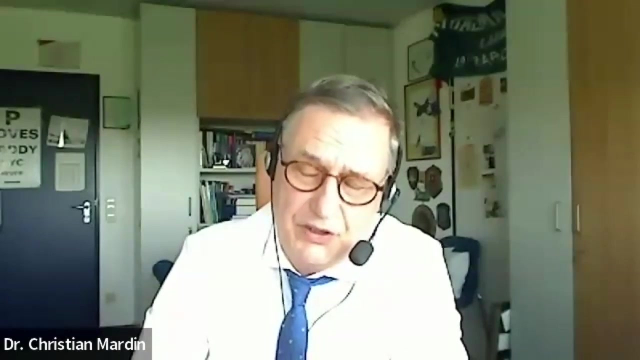 for routine cataract surgery in all patients. No, I wouldn't, because the availability of anterior segments OCT is not as common as posterior segment OCT In posterior segment OCT. for posterior segment OCT we do in our hospital, we do routinely. 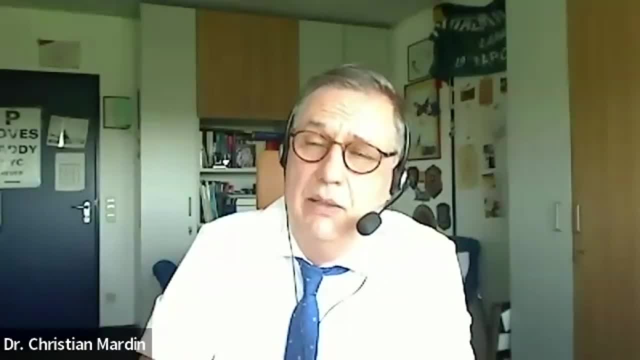 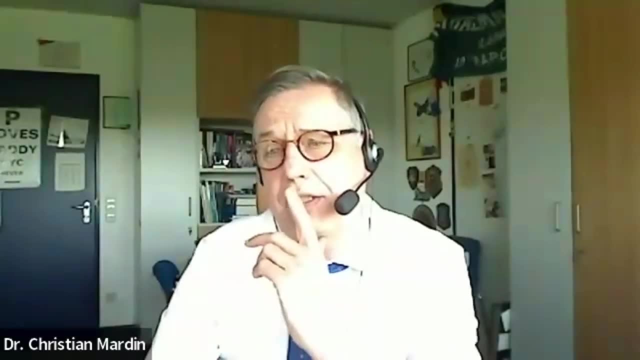 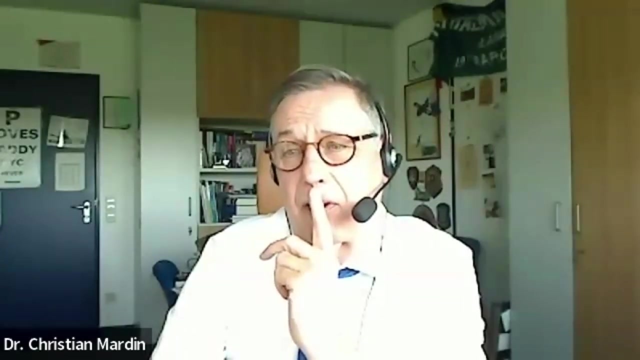 a scan of the posterior- especially when ophthalmoscopy is very blurred- of the fundus. How can we avoid the development of cataract? I think No. don't have other ocular pathologies and don't get old. 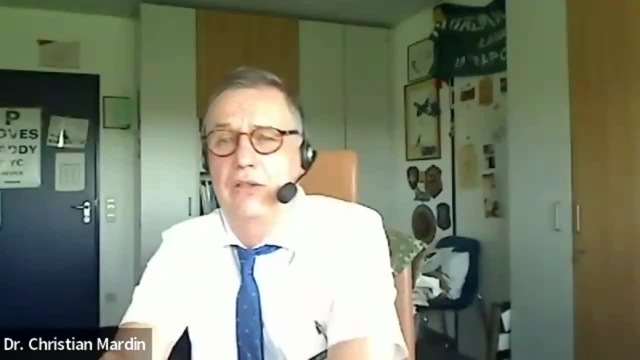 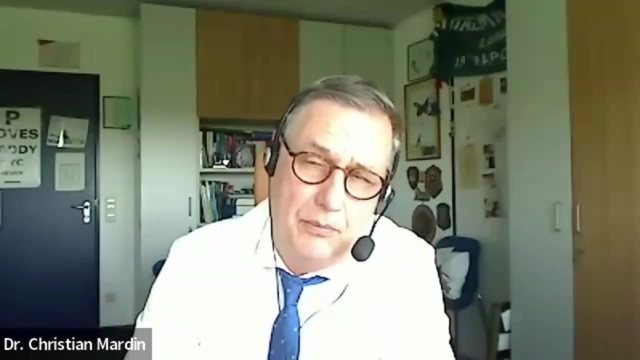 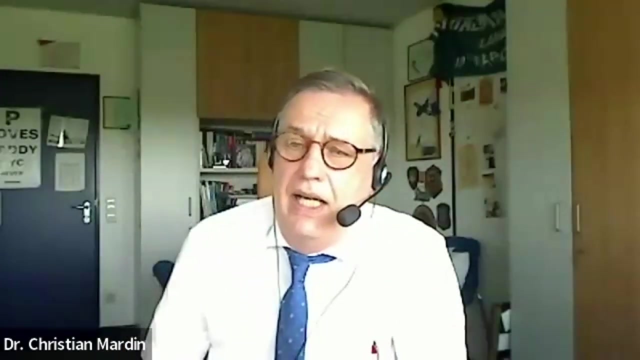 That would be my answer at the moment. Is it logical to do fundus OCT for every cataract patient pre-op? I think if you offer premium service then I would do it yes. The next question is: in OCT, any different kind of eye? 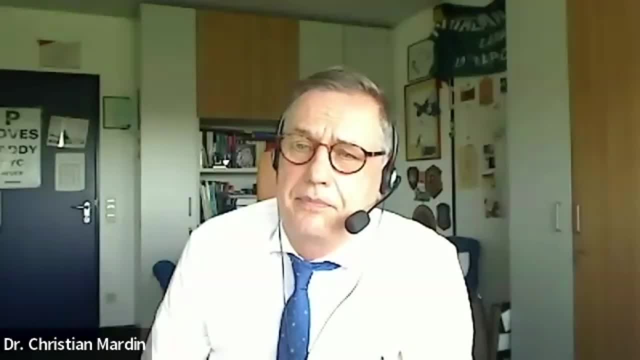 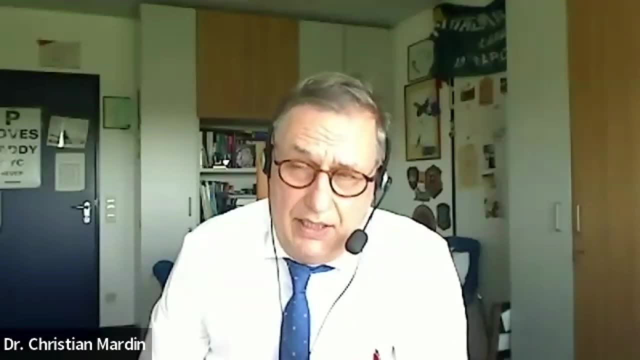 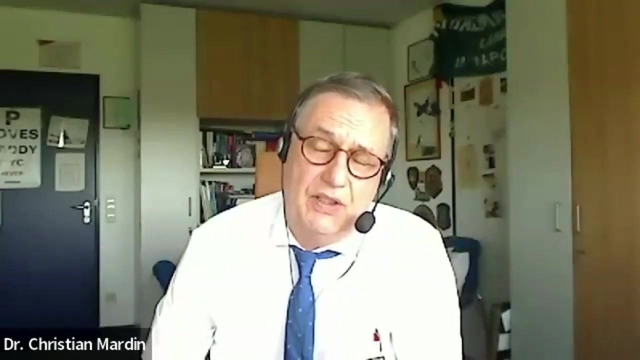 condition can show or not. I think You see most of the conditions if they're imminent in the central retina or optic nerve head. of course central changes like brain changes can't be estimated so easily. You can measure a ganglion cell layer. 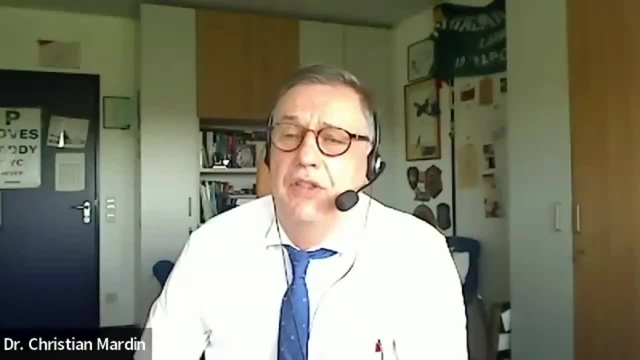 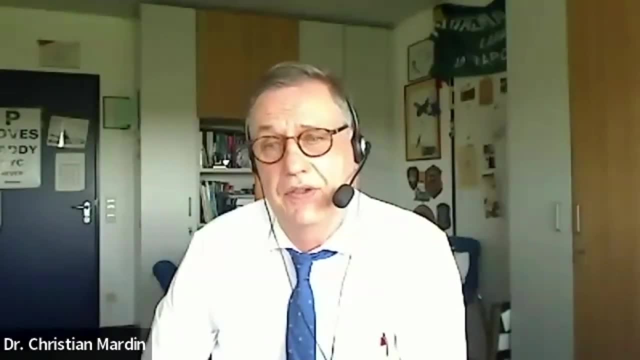 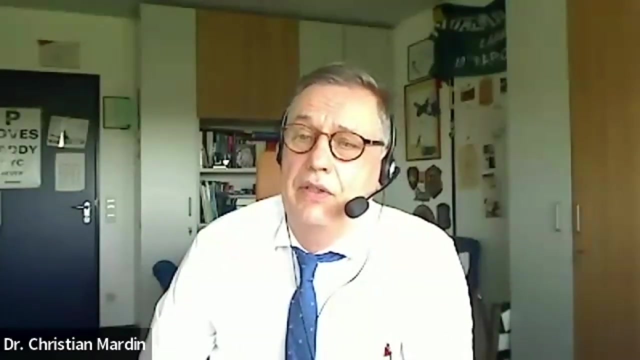 but that's very complicated. But eye conditions of the fundus can easily be appreciated. yes, Also, you have the infrared image I like very much and appreciate the fundus if I have a blurred ophthalmoscopic picture. PCO, do you use yak on the table or with needle after IOL insertation? 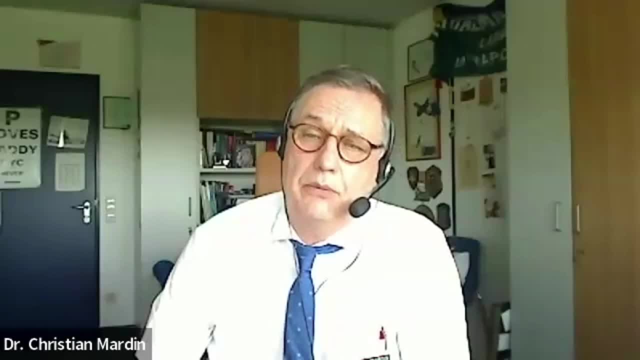 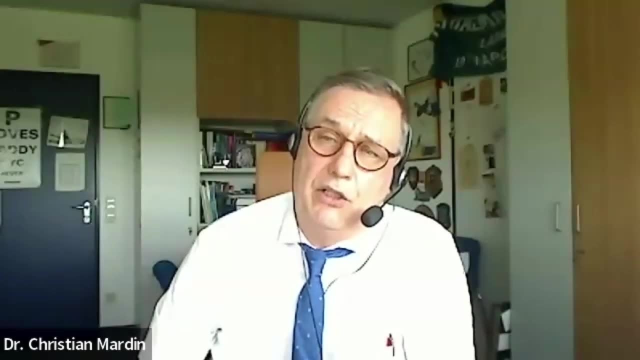 When I have posterior capsule opacity and I can't deal with it during surgery, I avoid opening up my capsular bag. I recall the patient after three weeks And do you? Yes, I can't do the yak in a sitting position for him. 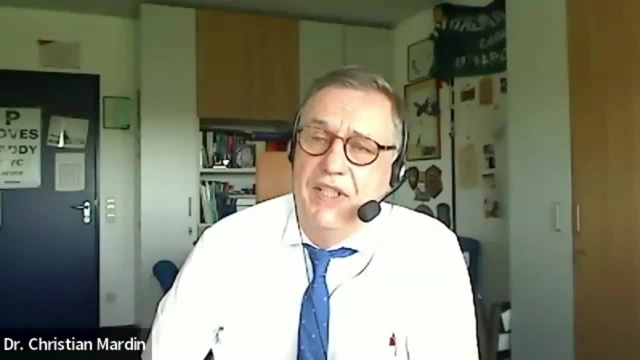 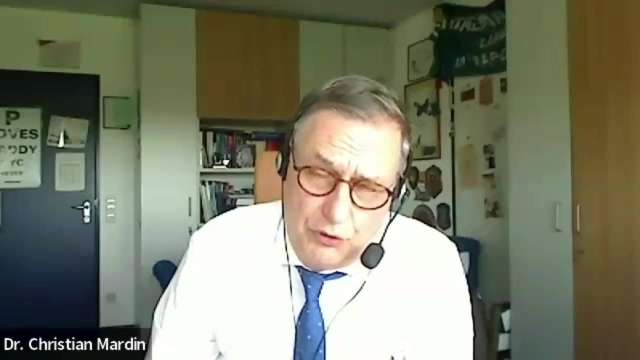 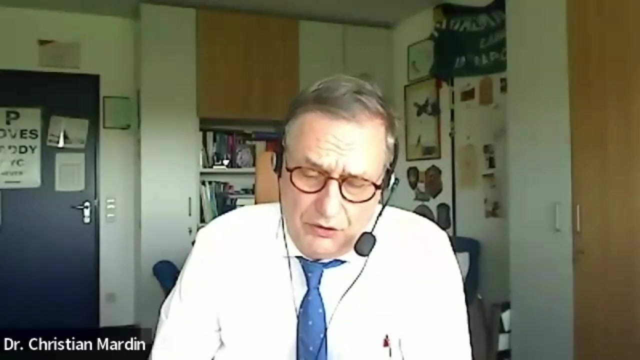 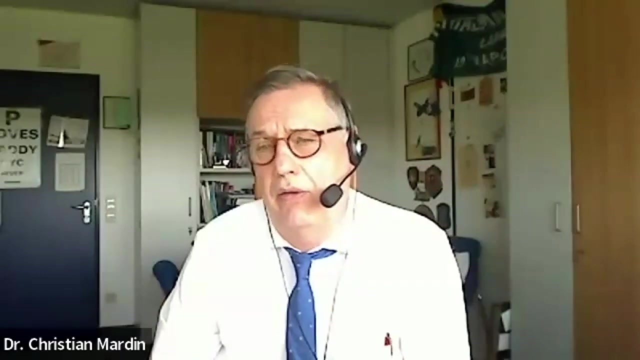 I think that's the most, the less dangerous way. How much signal strength of OCT is considered to be reportable? That depends on the producer of the device. There are, for each device, signal to noise ratios And the producer manufacturer tells you where the producer can do it and the producer can do it. 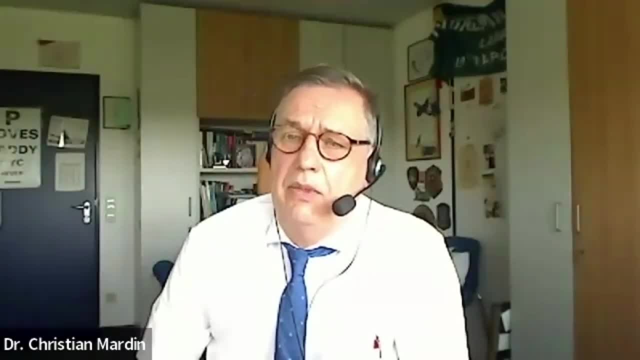 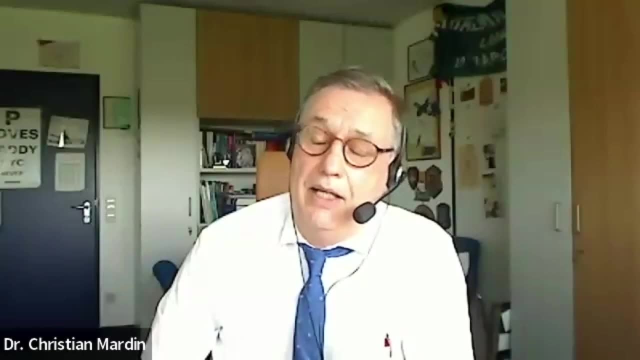 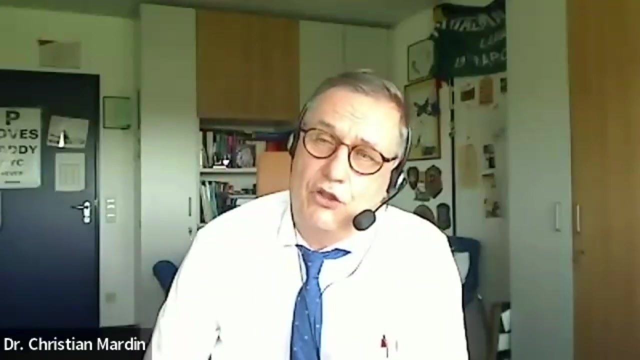 the border is OCT in animals. can it be replicated across other animals, not just humans? I think it depends on the anatomy of the animal you want to examine. I have done OCT already on some dogs presented to me. It works if you have the dog under the right condition not to bite you. 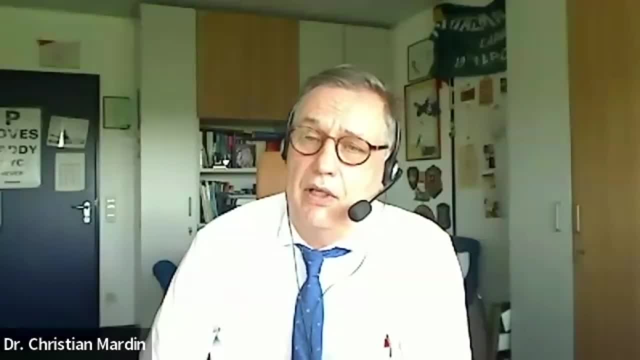 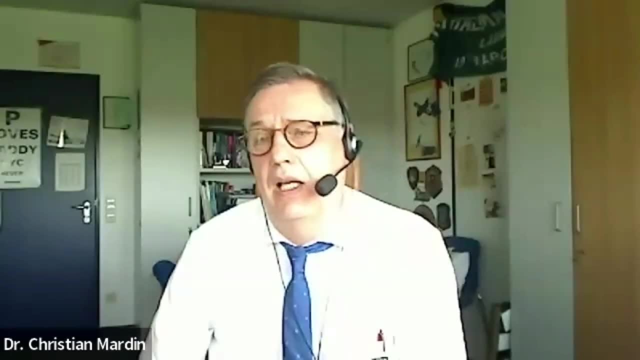 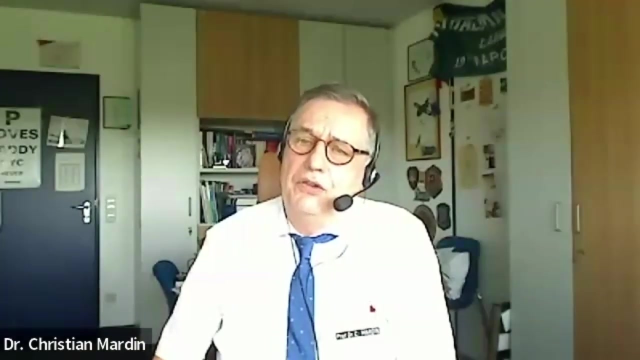 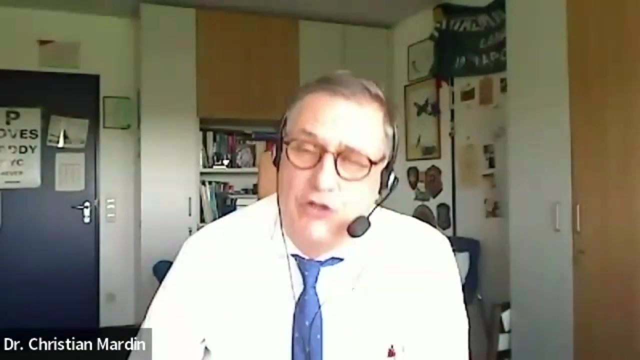 but it's possible, And even OCTs are done on rats, on very small eyes or mice, with special optics applied to the commercially available devices. Would you recommend posterior segment OCT for all elderly patients due for cataract surgery, If you are able to manage that and 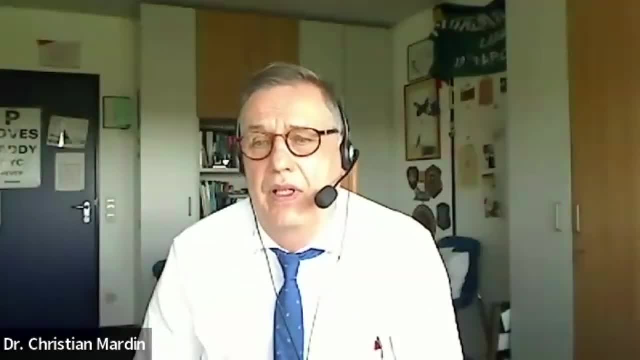 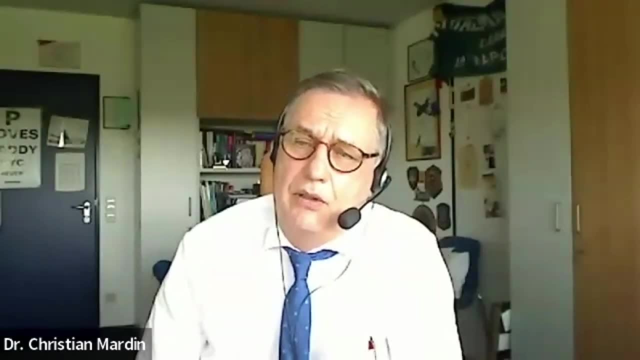 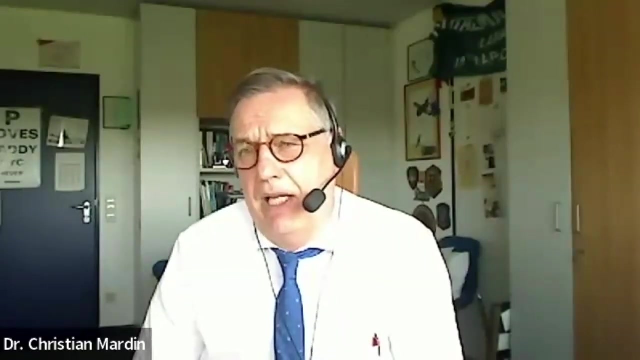 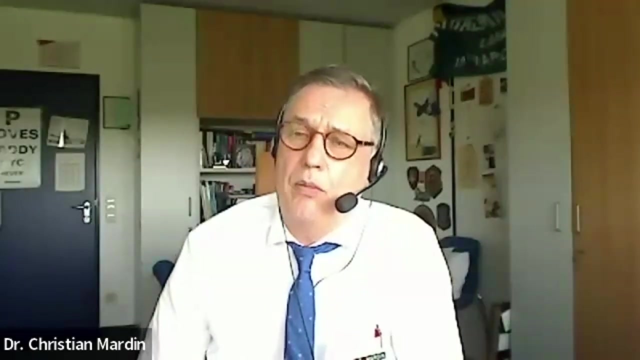 cataract is rather dense, I would recommend it. yes. Is it sufficient for surgery merely done by anterior segment OCT? This question I don't understand. but anterior segment OCT I would only apply in special cases like imminent angioglossal glaucoma or any pathologies of the anterior segment prior to. 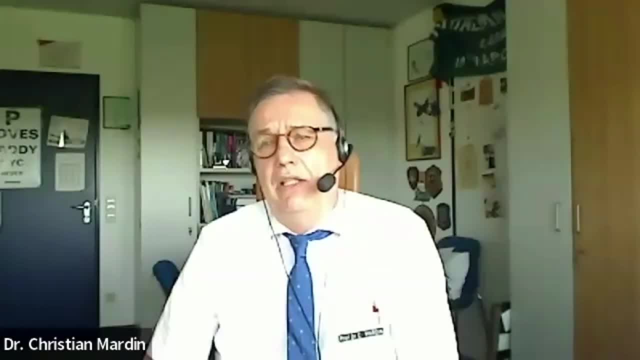 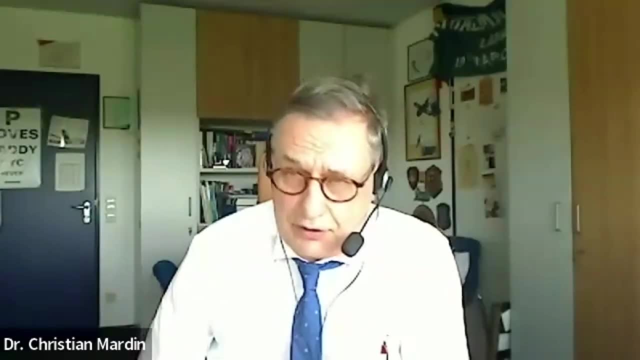 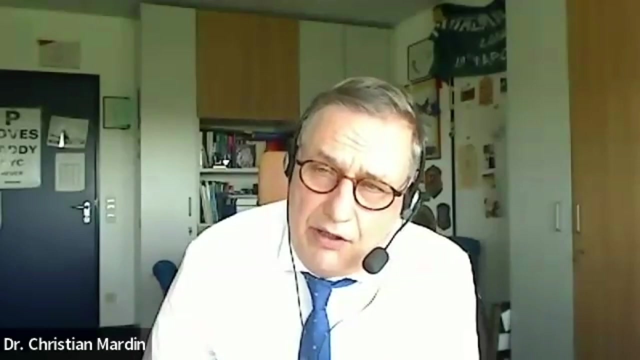 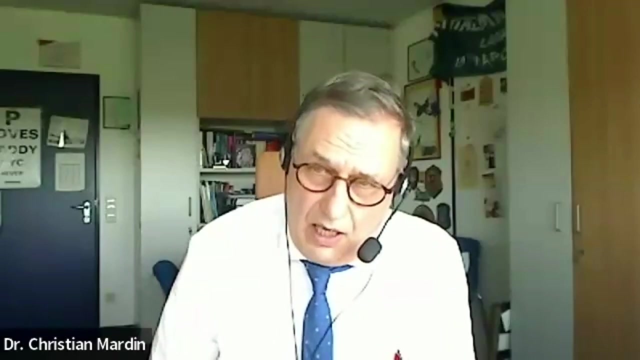 surgery. Can we only rely on OCT of the patient for cataract surgery? Of course not. I still prefer to see the patient with my own eyes and do my ophthalmoscopy. It's a very important additive examination but you can't replace all our skills we do when we do ophthalmoscopy and sit-lamp biomicroscopy. 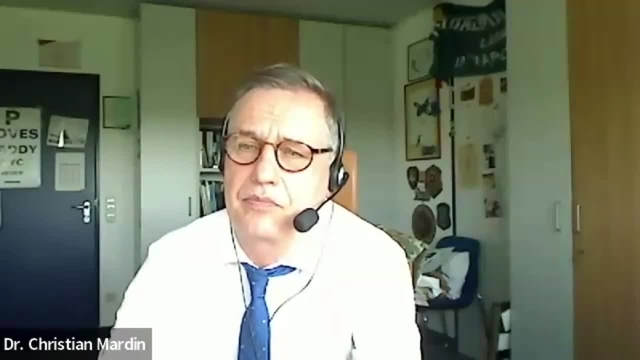 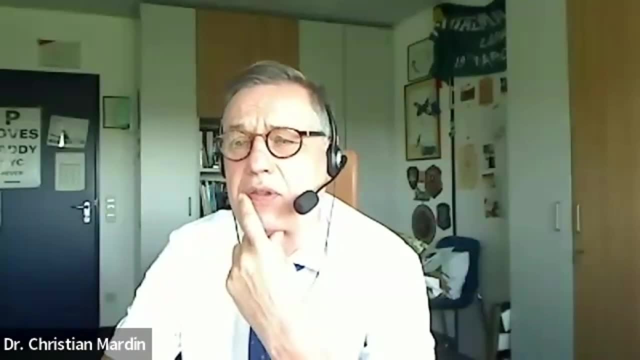 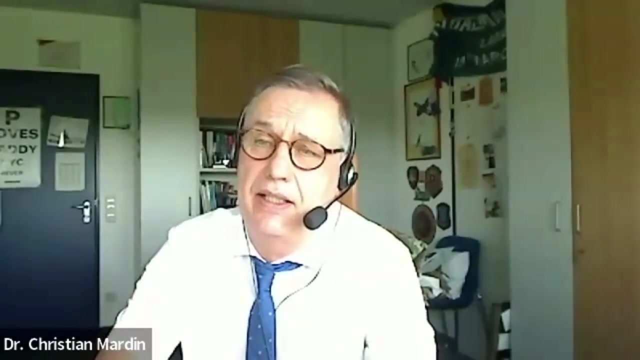 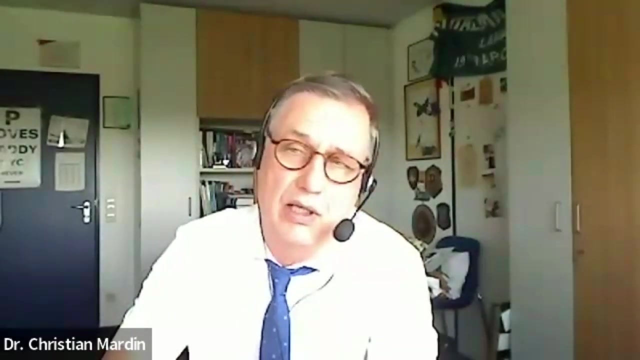 Another question from the chat: is anterior segment OCT indicated in post-operative refractive surgery eyes? If the patients are not satisfied, it's worth to look whether the anterior chamber depth is in the range you calculated or if the length position is okay. yes, 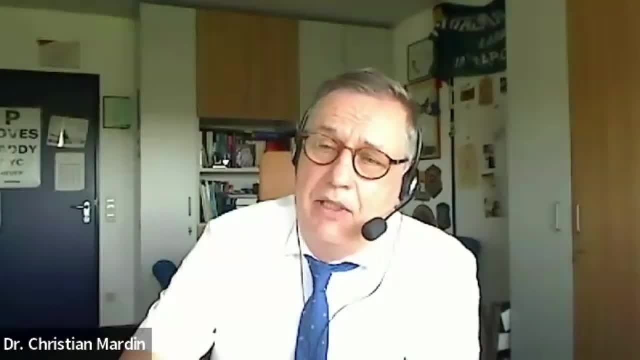 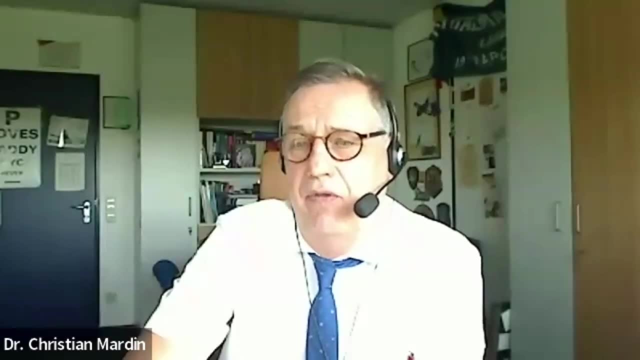 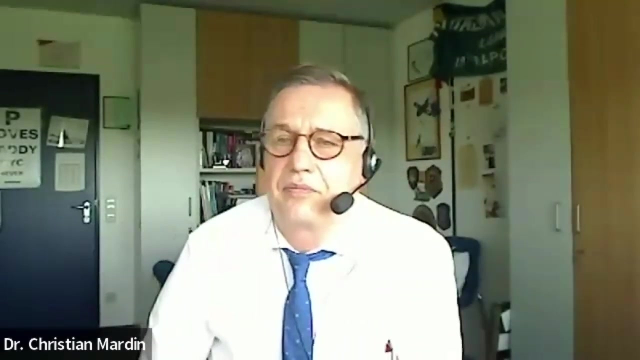 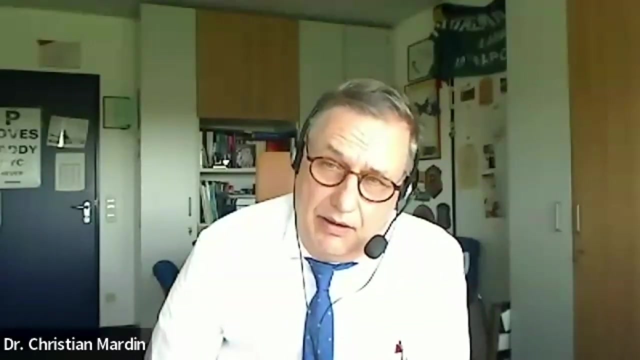 Yes, anterior segment OCT is not addressed so often. therefore, I used the last 15 minutes to address this point because there are indications where you can make patients happy or yourself happy. I answered that last question already. I would do OCT in the routine for all the cases where 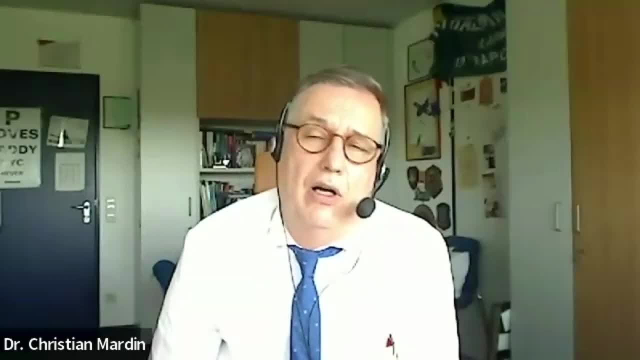 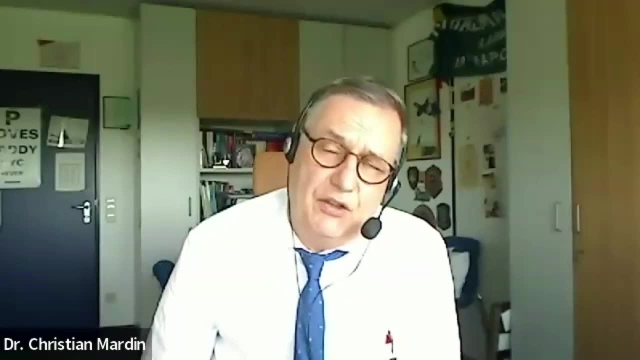 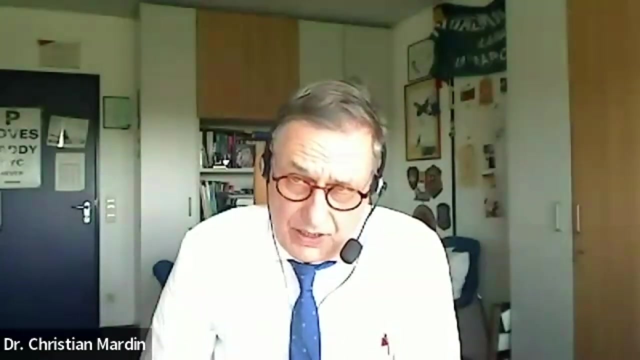 the ophthalmoscopy may be different. I showed the slide where to think of if it is discrepancy between lens opacity and vision. If the patient has a history on the fundus, then I always would perform OCT, in all diabetics of course, because they may have CME and after cataract surgery. 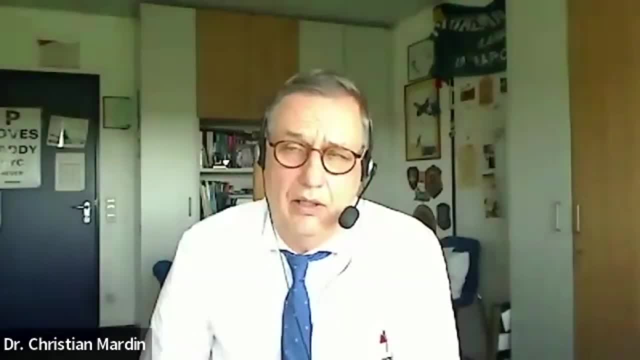 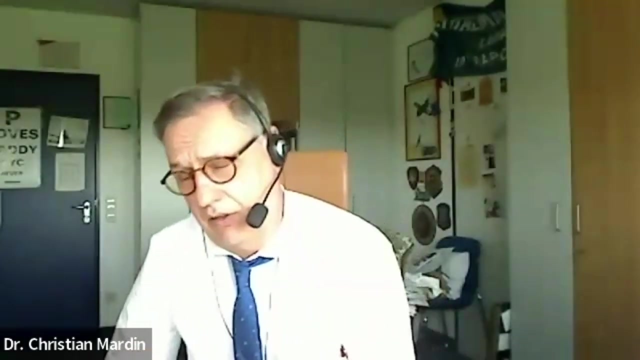 it may turn larger and then it's very difficult to treat these patients. You need steroids anti-VEGF for a long time. Can OCT be done in intumescent cataracts? If you have the right wavelength in the infrared picture spectrum then it may be possible, but not always. 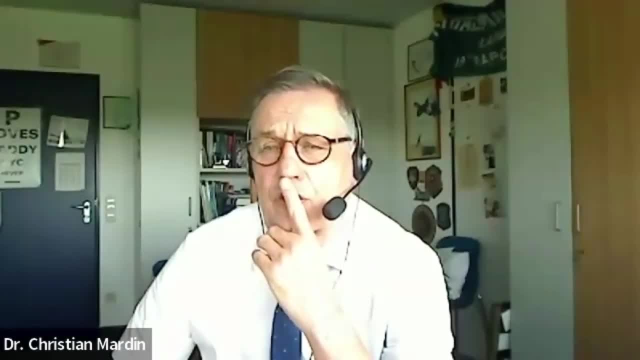 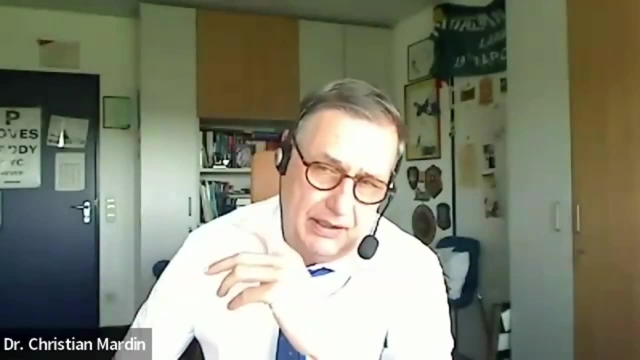 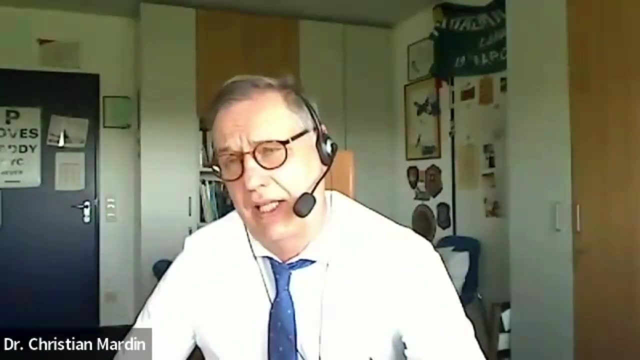 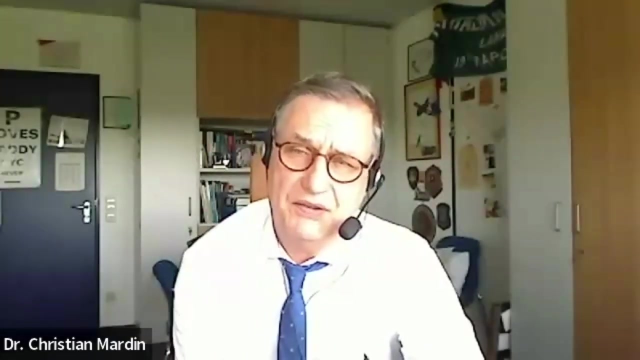 Is OCT the best option surgery for cataracts. At the moment, optical corals tomography is still, I think, the best option to image posterior and anterior segment, higher in the resolution than echography at the moment. But if you want to look at the cellular body for tumors, for example for solid masses, then you 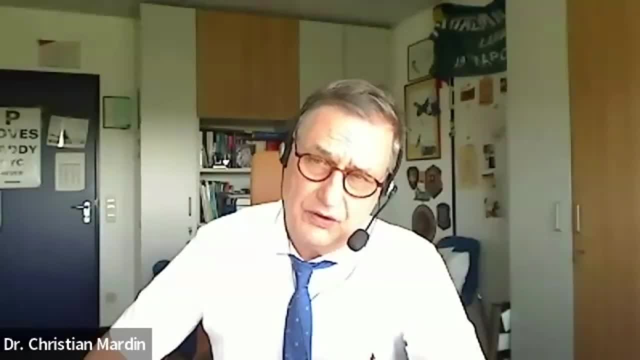 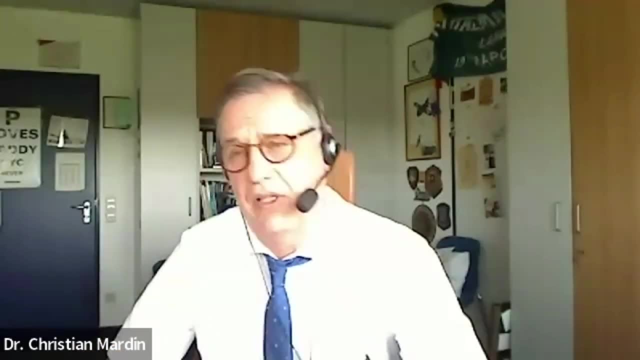 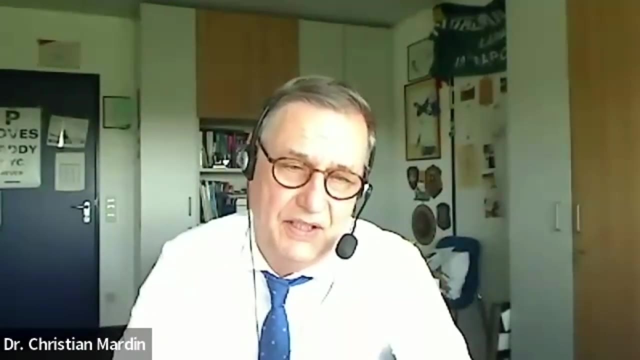 have to use ultrasound biomicroscopy because ultrasound penetrates the pigment of epithelium and the pigment of epithelium, on the other hand, blocks our laser light. It was my pleasure to have so many listeners- We are at the moment 221- from all over the world. 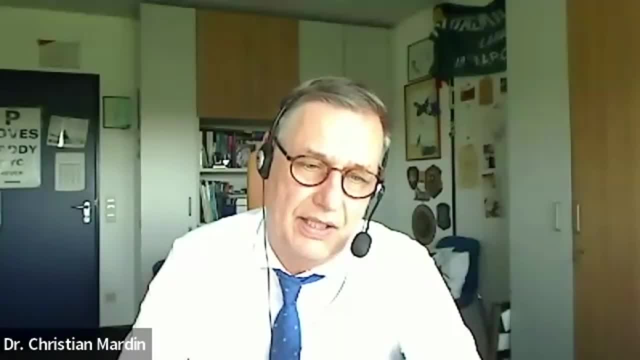 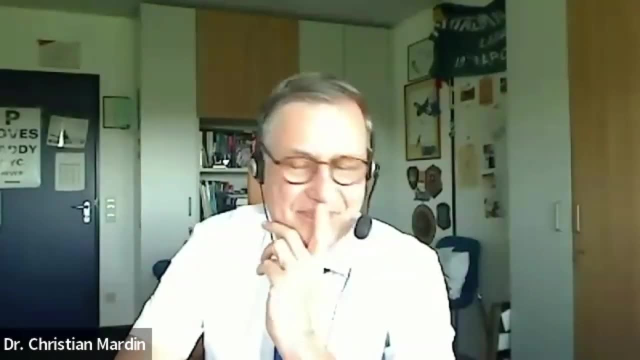 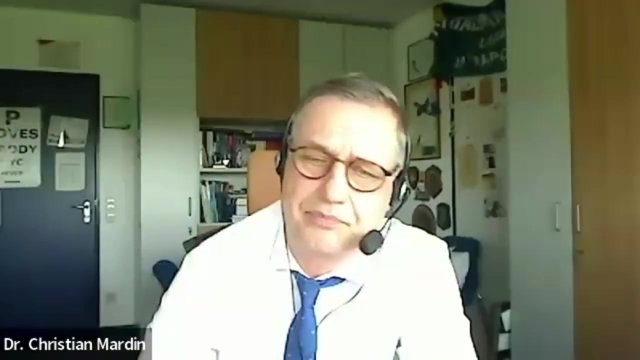 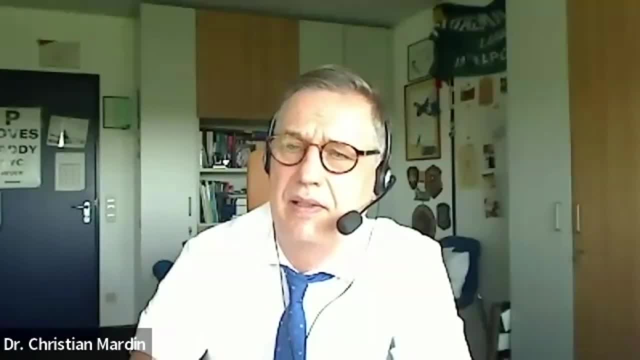 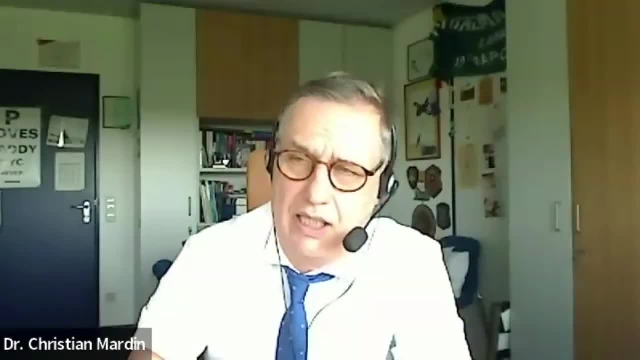 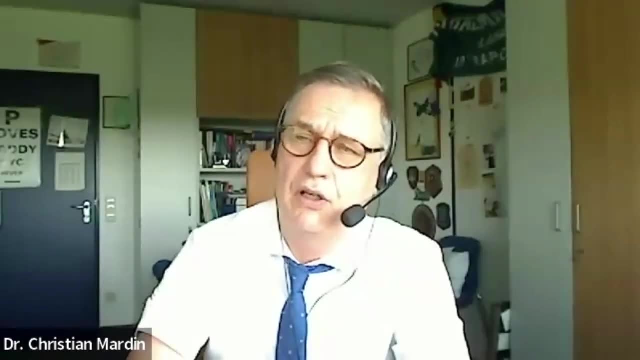 If there are more detailed questions you can't ask at the moment, of course, Orbis, I think, will feel happy to pass the questions to me to be solved by email. That's no problem at all, Thank you, Thank you. 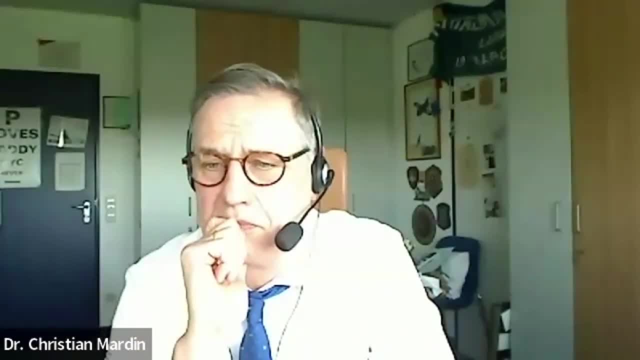 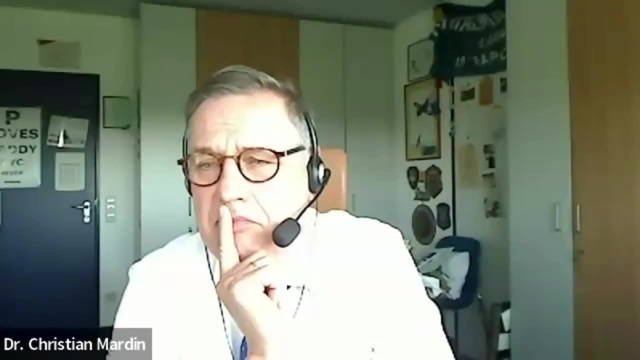 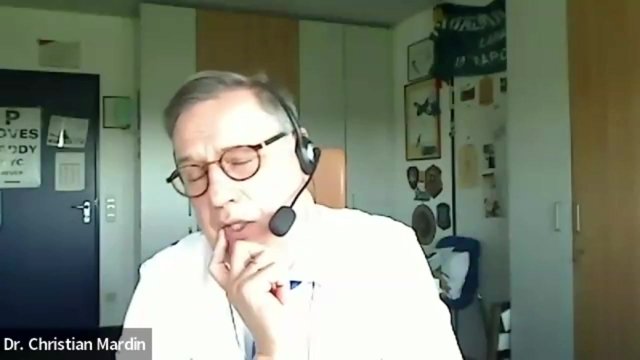 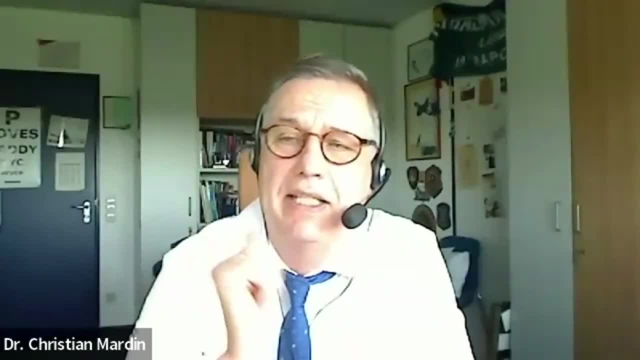 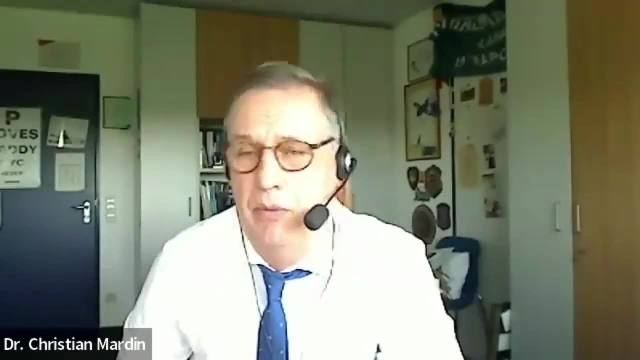 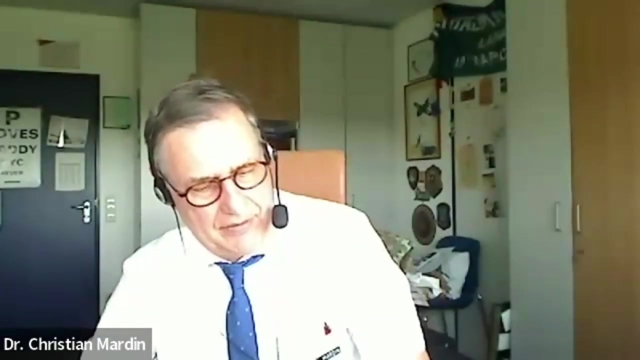 Therefore, I thank you very much for all attending the lecture, even if it's very late for you or, for some people, rather early where you still have to work. I have to thank the guys from Orbis, Andy and Hunter, which made it so easy from the 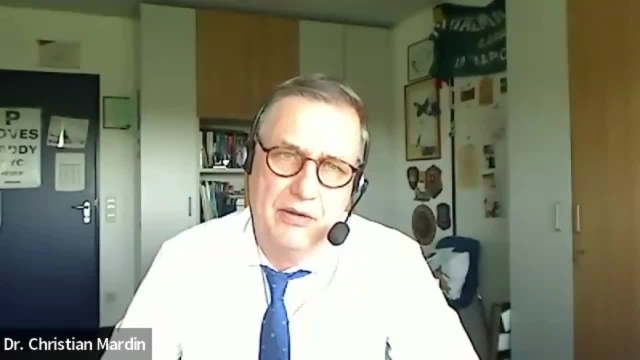 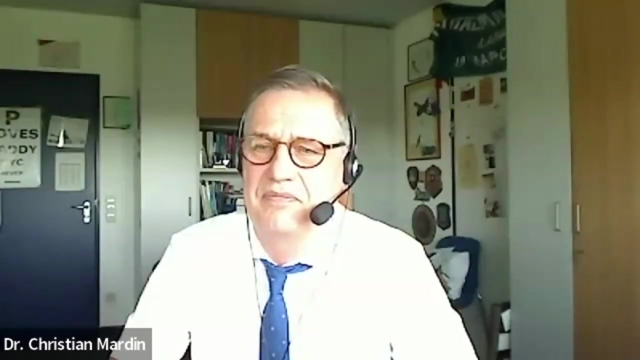 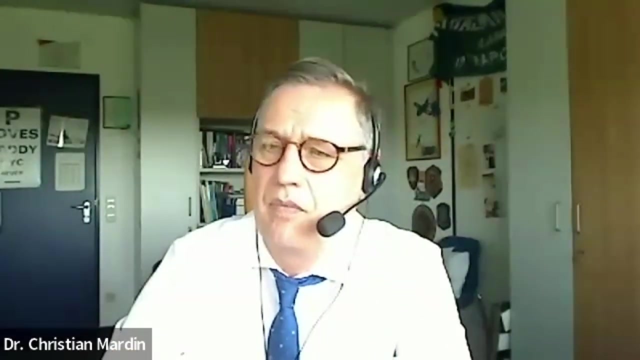 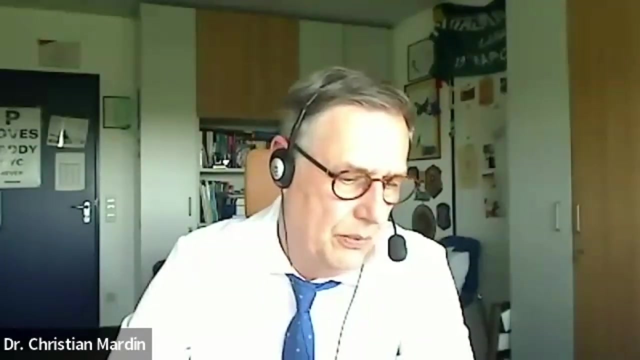 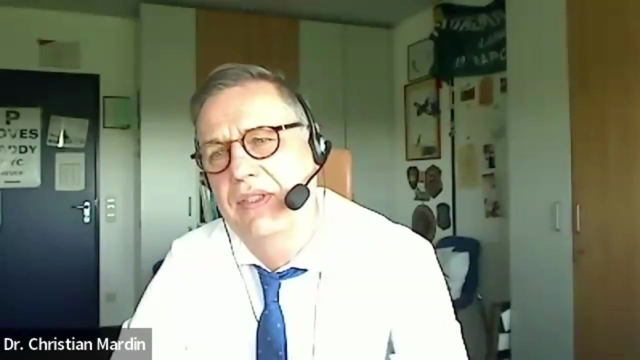 technical side to reach you and make the polling possible. They are really professionals. I'm really looking forward to the next lecture in July. So at the moment, all questions are answered. We still got two more minutes for questions. I will stay online for the next two minutes to take perhaps a late-comer question. 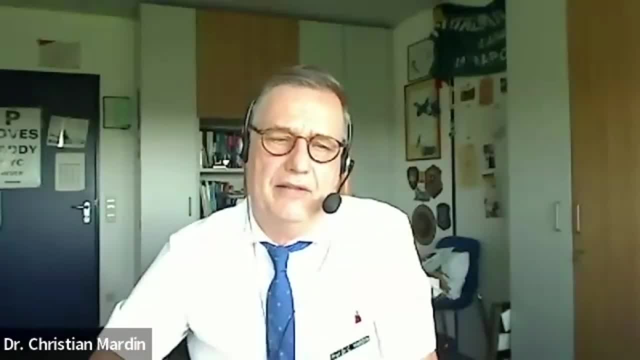 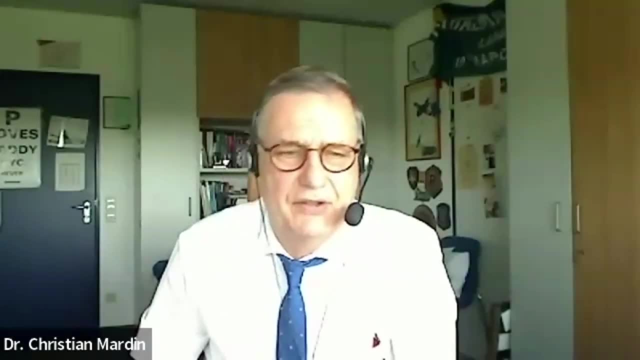 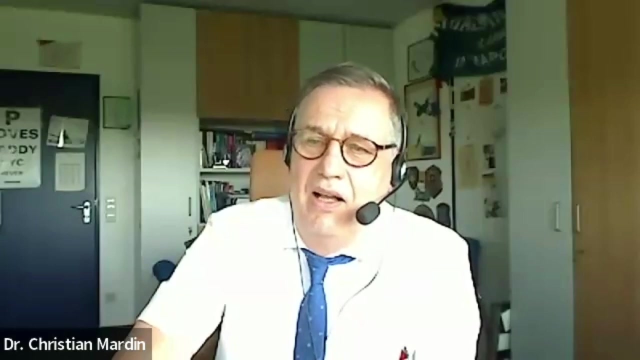 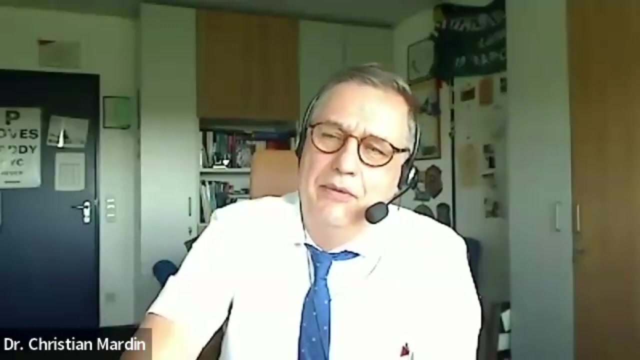 Otherwise, I would like to thank you again for listening from all over the world and I hope you have a great day. Bye-bye project. i think 11 times and always, i think, learned more myself than i taught at the hospital. it was great fun. 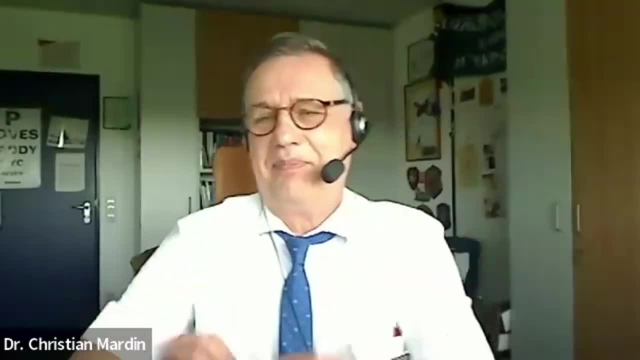 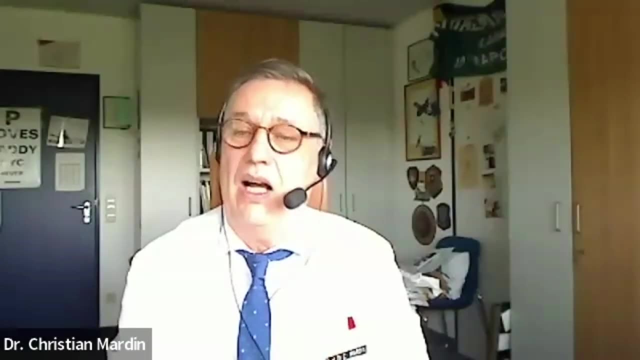 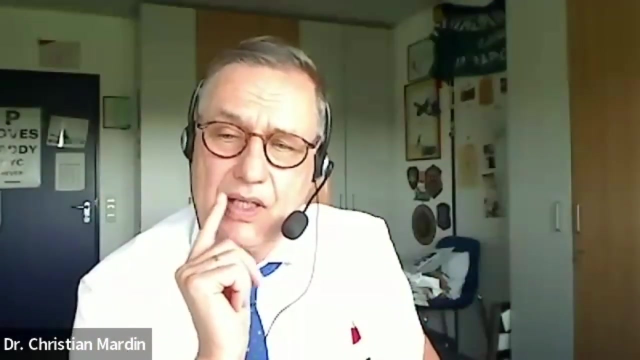 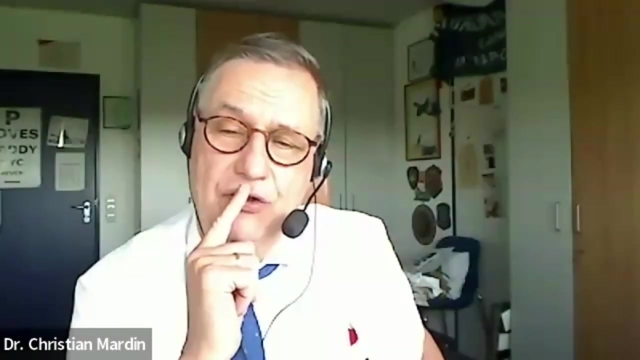 oh, peru is very far, but it's early in the morning, four o'clock, ah, in the afternoon, okay, um, ah, good question: any age above which you will always do ocq in cataract patients? um no, no, i wouldn't think so, because you saw that even you get in a young patient's surprises. 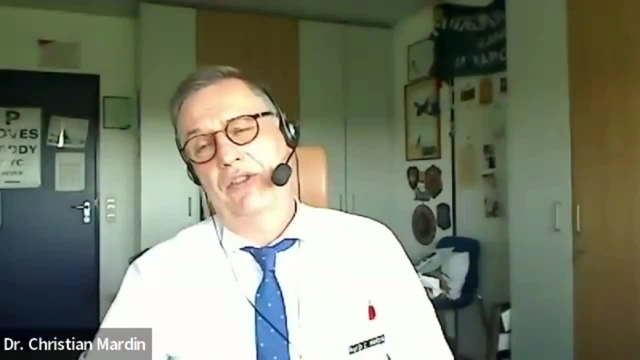 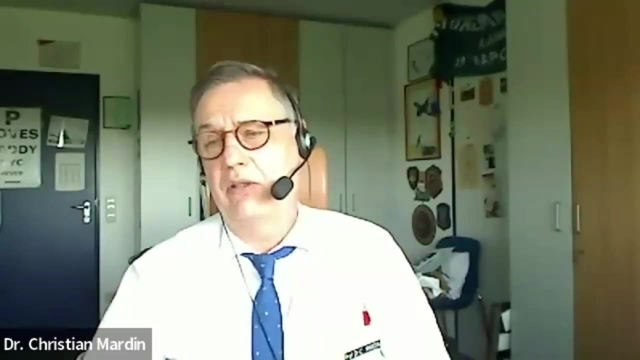 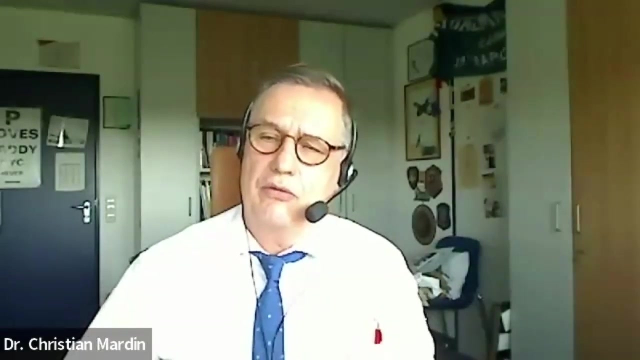 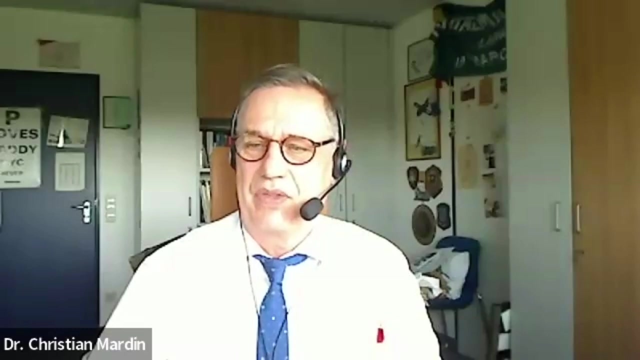 and in very old patients you have a higher chance to meet amd, diabetes, changes from arterial hypertension or epidural membranes of the brain. so it's very good question. um, um course, but i would not name here as a certain age without trying to discriminate anyone. the lens thickness influences scattering operating procedure. 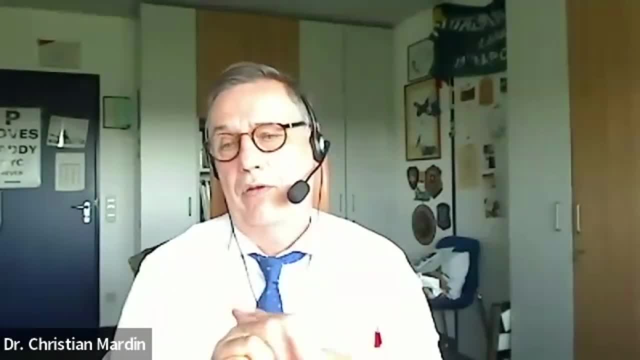 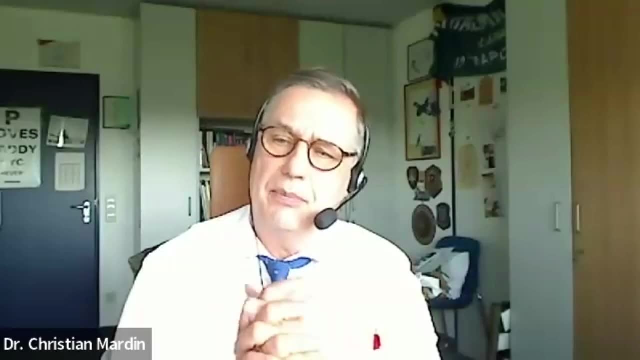 yes, you might need more faco energy, of course, and i think the density of the lens is the the bigger problem. but, um, the space you have in the capsular back may cause problems for the posture effect, a post-operative refraction you might end up in. 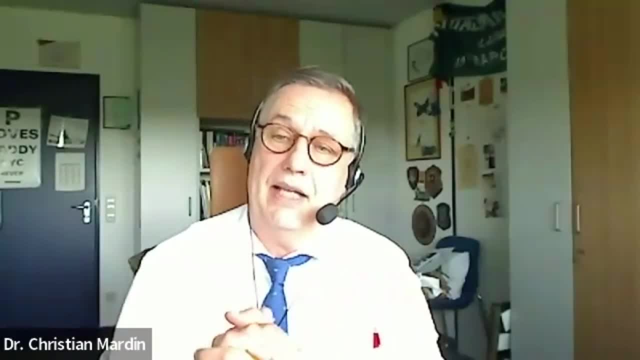 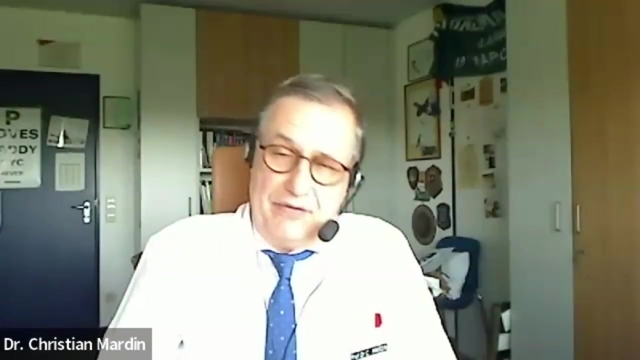 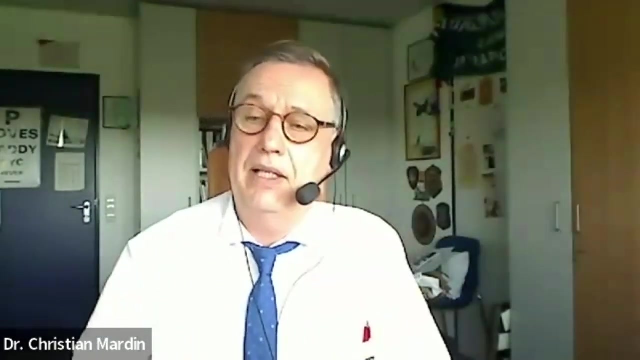 a hypopia, more myopia side, and, and that's um that may cause an unhappy patience, that's right. and of course, the lens thickness. if the lens thickness is double as thick as the anterior chamber, death, then you have to um keep in mind that you, by dilating the pupil for surgery, you might end up in a angle block.